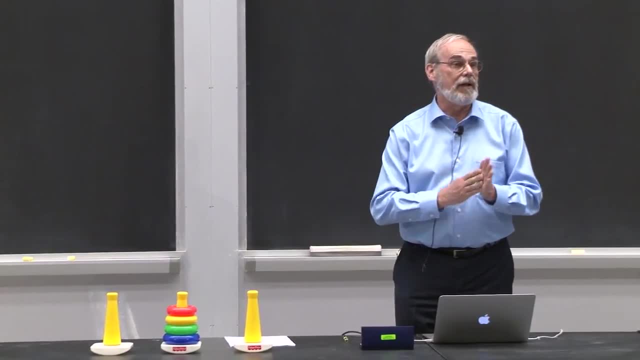 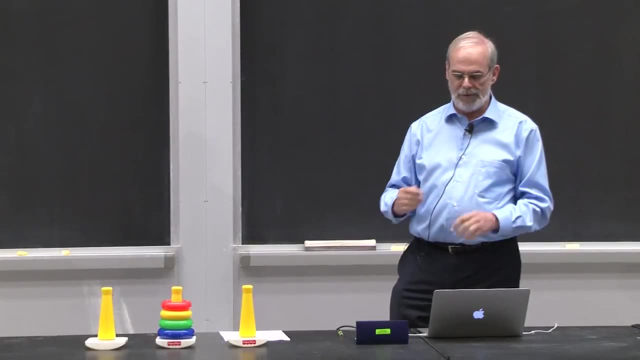 It would change the appearance of the contents of the other, And that leads to some nice challenges. So the side effects of mutability are one of the things you're going to see, both as a plus and a minus as we go through the course. 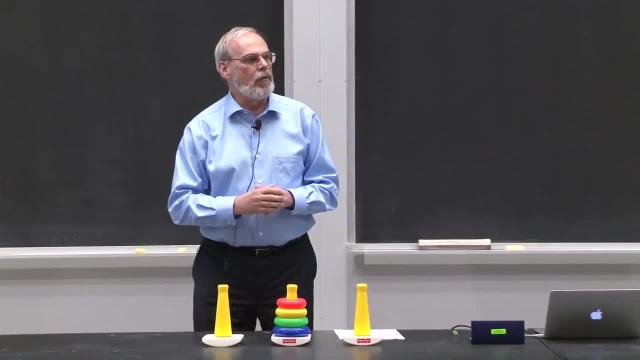 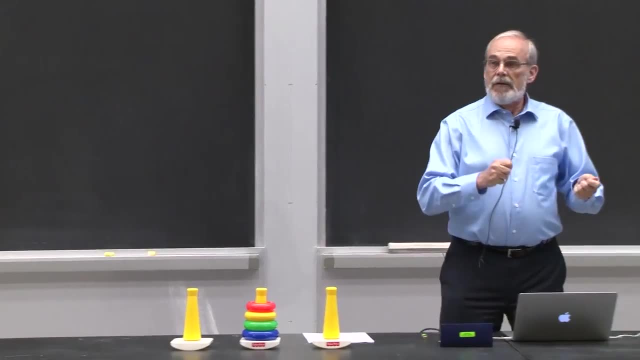 Today, we're going to take a different direction for a little while. We're going to talk about recursion. It is a powerful and wonderful tool for solving computational problems. We're then going to look at another type of compound data structure, a dictionary, which is also mutable. 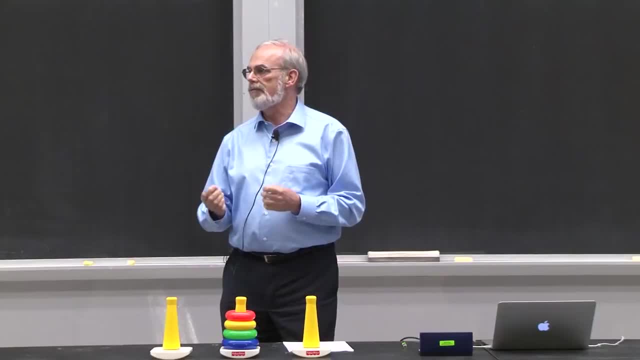 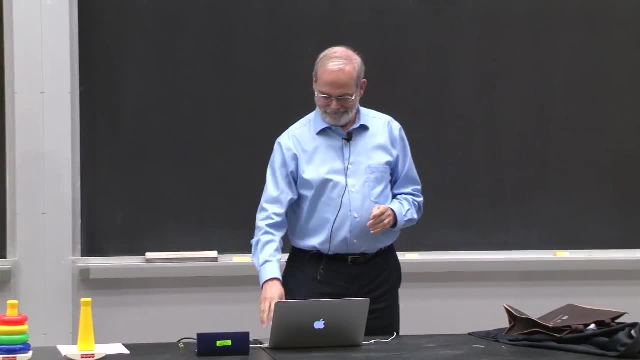 And then we're going to put the two pieces together and show how together they actually give you a lot of power for solving some really neat problems very effectively. But I want to start with recursion, Perhaps one of the most mysterious- at least according to programmers- concepts in computer science. 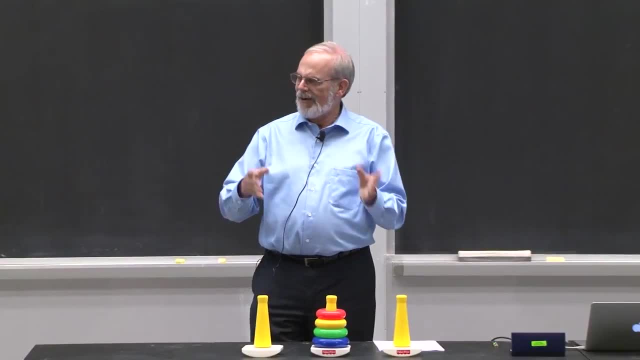 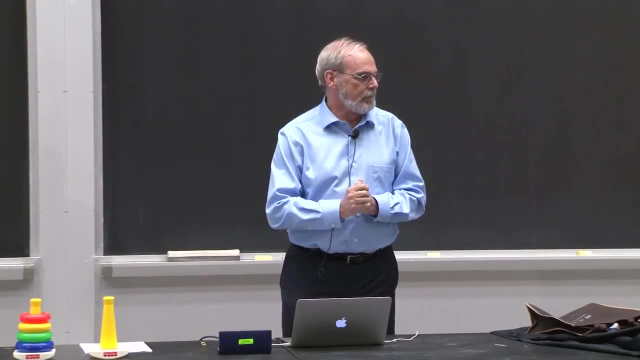 One that leads to lots of really bad computer science jokes. Actually, all computer science jokes are bad, but these are particularly bad. So let's start with the obvious question: What is recursion If you go to the ultimate source of knowledge, Wikipedia? 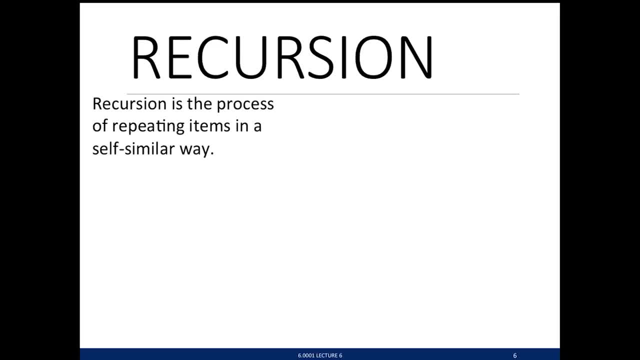 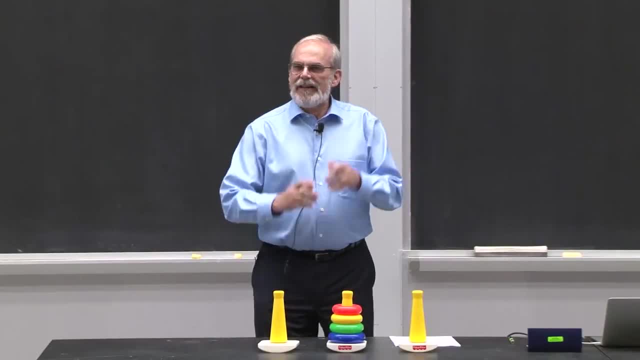 you get something that says, in essence, recursion is the process of repeating items in a self-similar way. Well, that's really helpful, right? But we're going to see that idea, because recursion, as we're going to see in a second, is the idea of taking a problem. 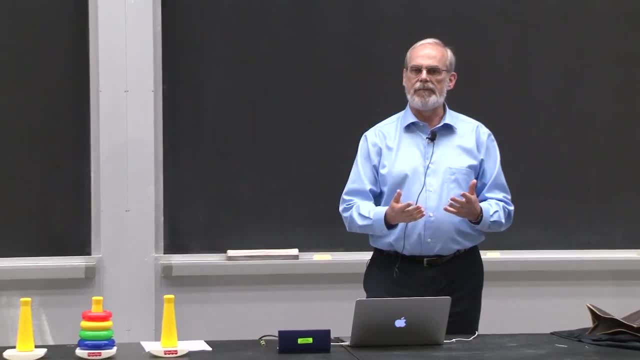 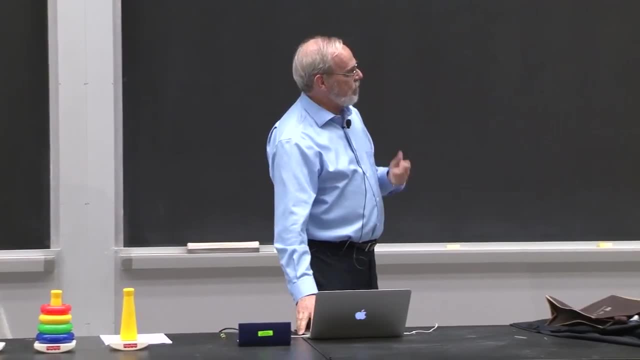 and reducing it to a smaller version of the same problem and using that idea to actually tackle a bunch of really interesting problems. But recursion gets used a lot of places, So it's this idea of using a recursion. So it's this idea of using a recursion. 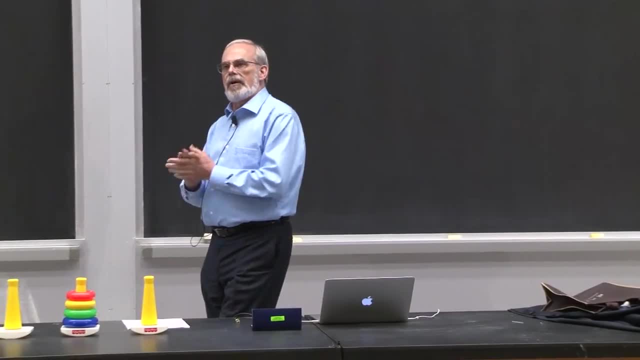 So it's this idea of using a recursion. You're repeating the idea multiple times, So you know, wouldn't it be great if your 3D printer printed 3D printers and you could just keep doing that all the way along? 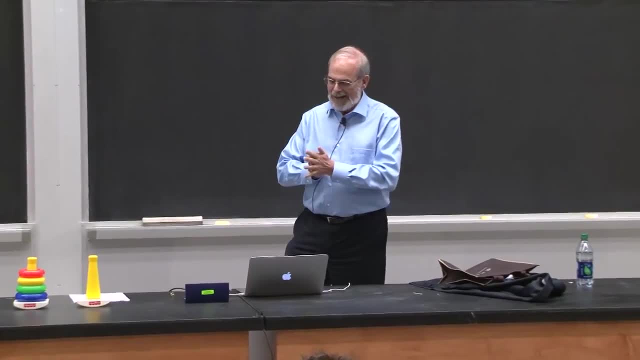 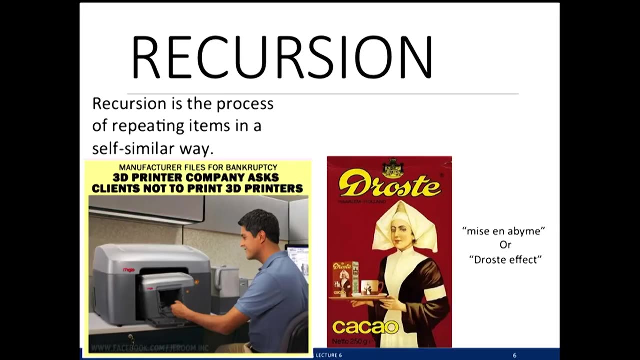 Or one that's a little more common. It's actually got a wonderful name: It's called mise en abîme, in art sometimes referred to as the Drost effect. Pictures that have inside them a picture of the picture, which has inside them a picture of the picture, and you get the idea. 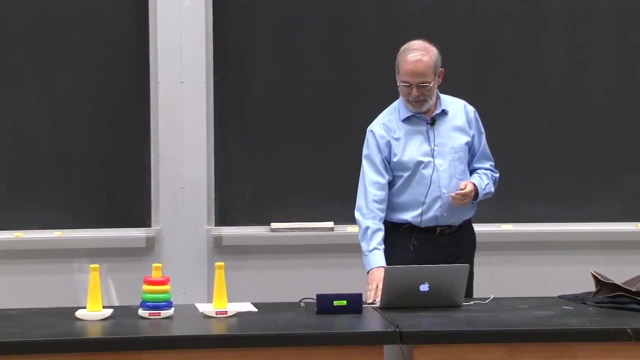 And, of course, one of the things you want to think about in recursion is not to have it go on infinitely. And yes, there are even light bulb jokes about recursion. If you can't read it, it says: how many twists does it take to screw in a light bulb? 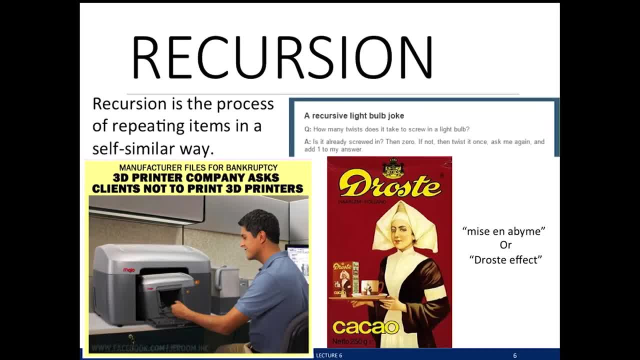 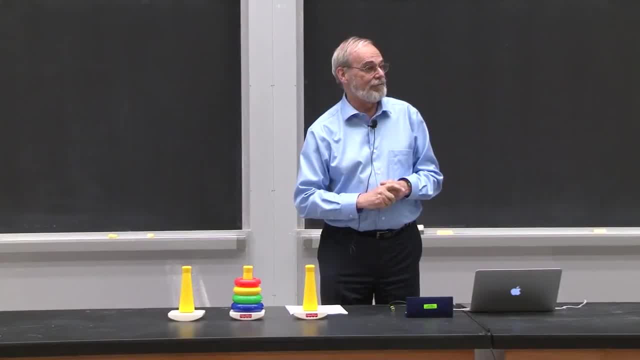 And it says: if it's already screwed in, the answer is zero. Otherwise twist it once. ask me again, add one to my answer. And that's actually a nice description of recursion. So let's look at it more seriously. 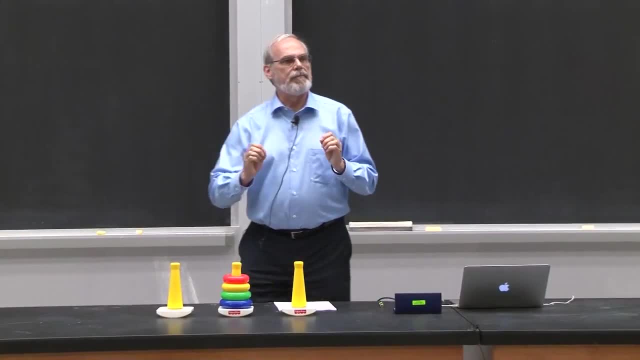 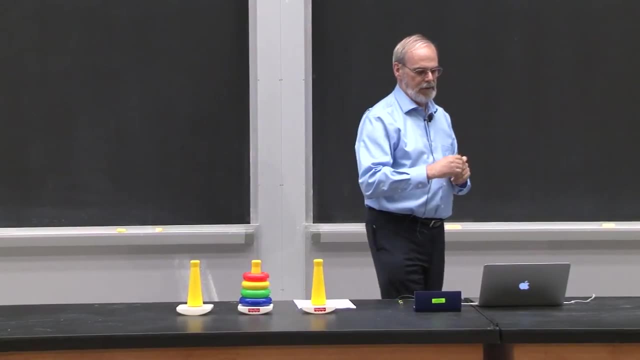 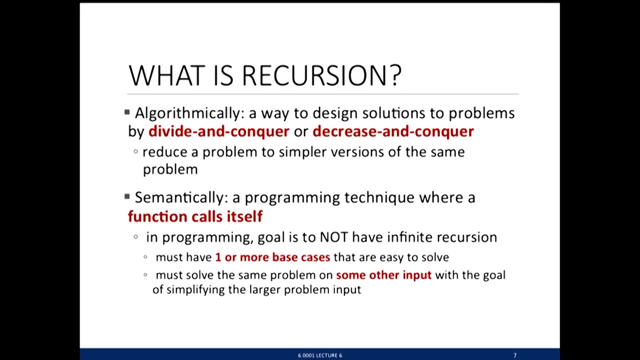 What is recursion? I want to describe it both abstractly or algorithmically and semantically or, if you like, in terms of programming. Abstractly, this is a great instance of something often called divide-and-conquer or sometimes called decrease-and-conquer. 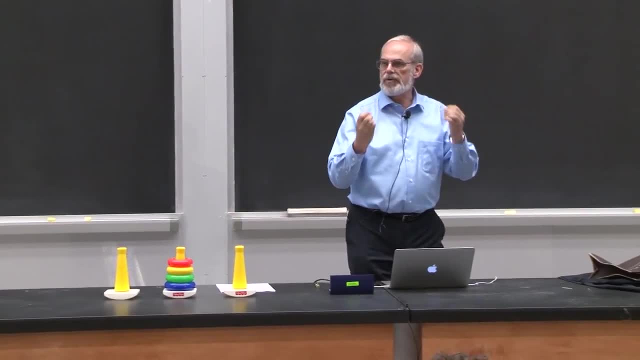 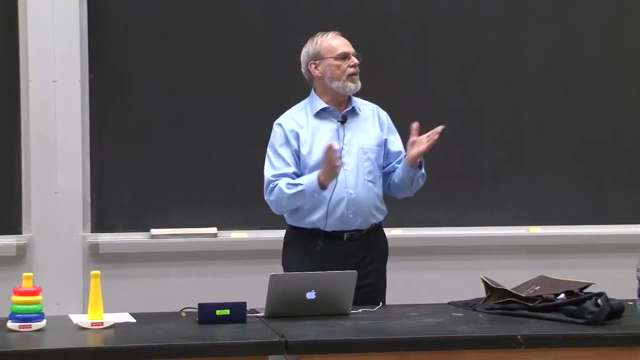 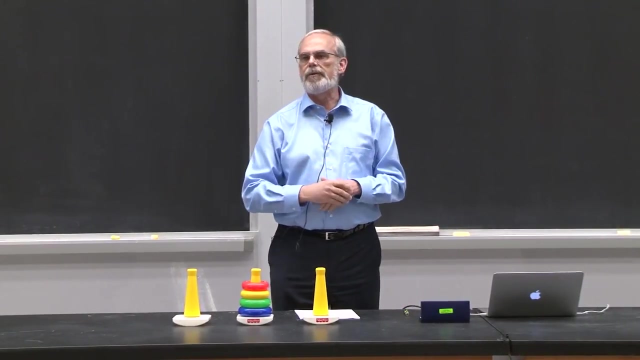 And the idea of recursion is: I want to take a problem I'm trying to solve and say: how could I reduce it to a simpler version of the same problem, plus some things I know how to do, And then, that simpler version, I'm going to reduce it again and keep doing that until I get down to a simple case that I can solve directly. 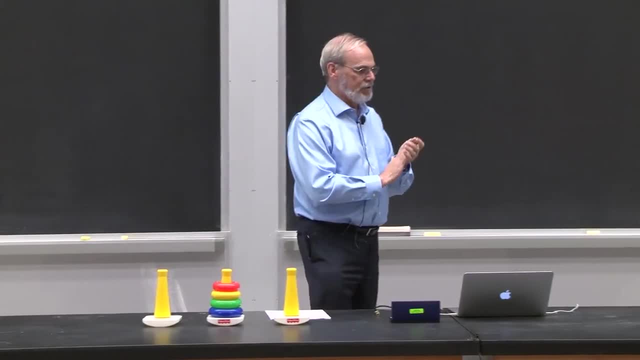 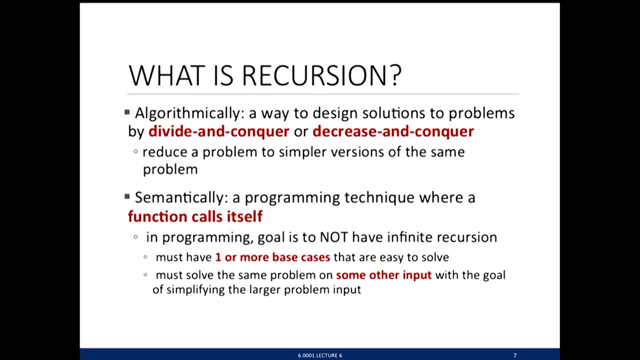 That is how we're going to think about designing something, And only if we're going to have solutions to problems. Somatically, this is typically going to lead to the case where a program, a definition, a function will refer to itself in its body. 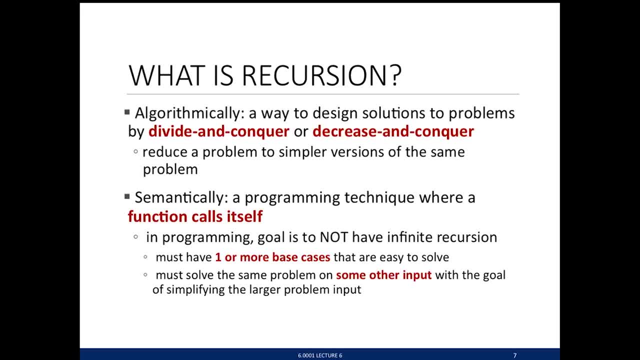 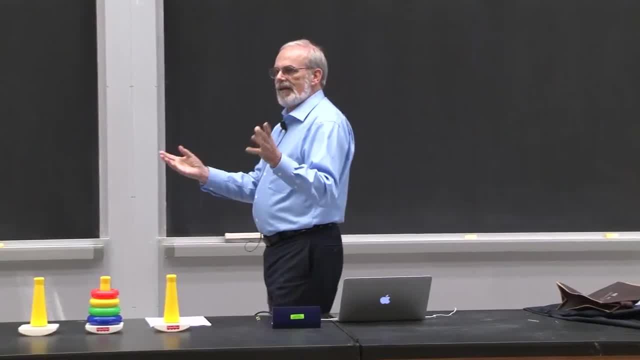 It will call itself inside its body. Now, if you remember your high school geometry teacher, she probably would wrap your knuckles, which you're not allowed to do, because in things like geometry, you can't define something in terms of itself. 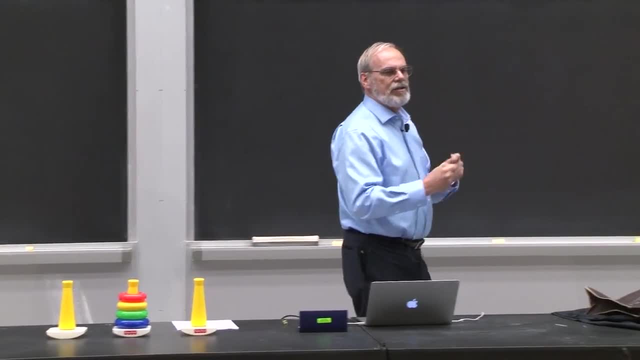 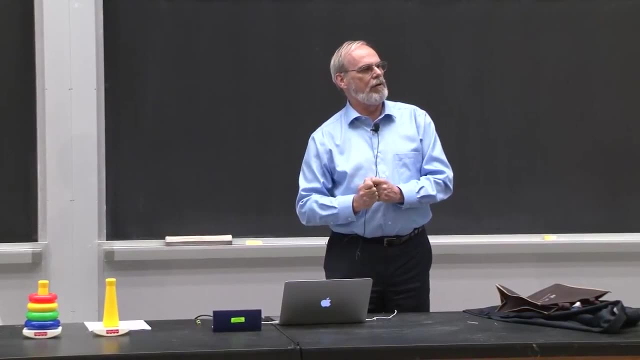 That's not allowed In recursion. this is okay. Our definition of a procedure can, in its body itself, stop itself, So we're going to imagine that body call itself, so long as I have what I call a base case, a way of stopping that unwinding of the problems when I get 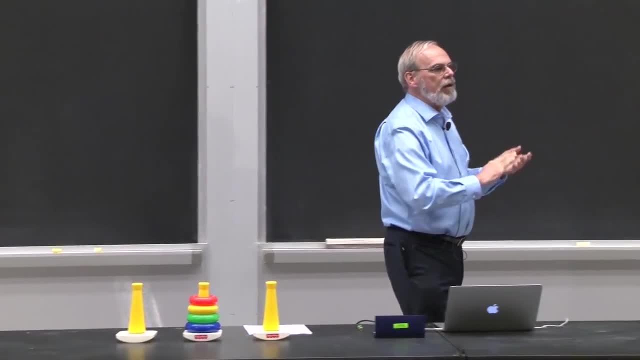 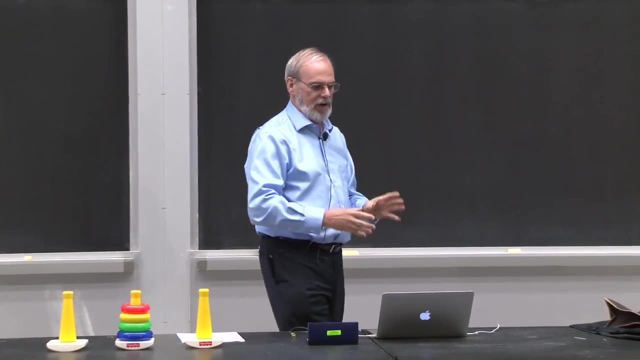 to something I can solve directly, And so what we're going to do is avoid infinite recursion by ensuring that we have at least one or more base cases that are easy to solve, And then the basic idea is: I just want to solve the same problem on some simpler input. 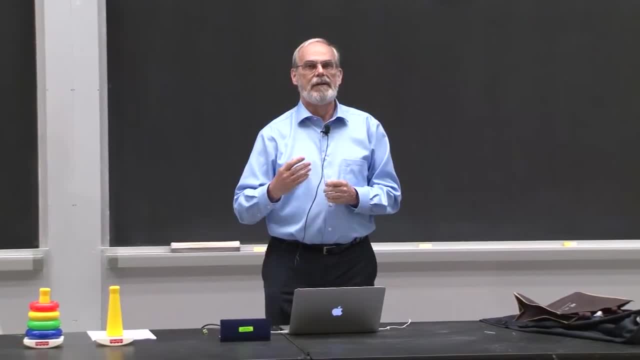 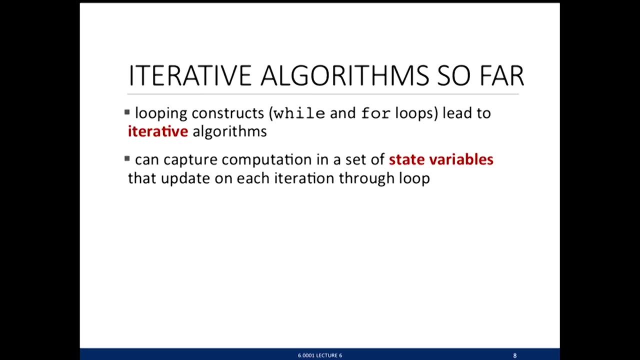 with the idea of using that solution to solve the larger problem. OK, let's look at an example And, to set the stage, I'm going to go back to something you've been doing: iterative algorithms For loops. while loops, they naturally 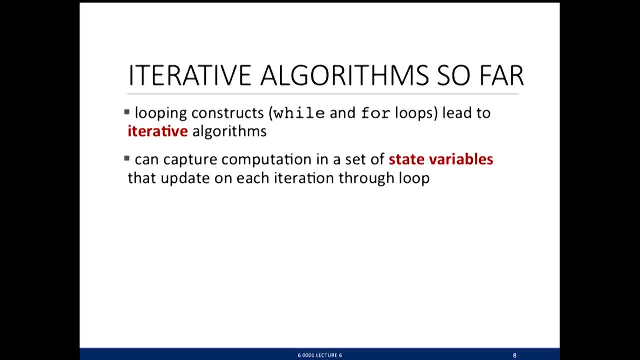 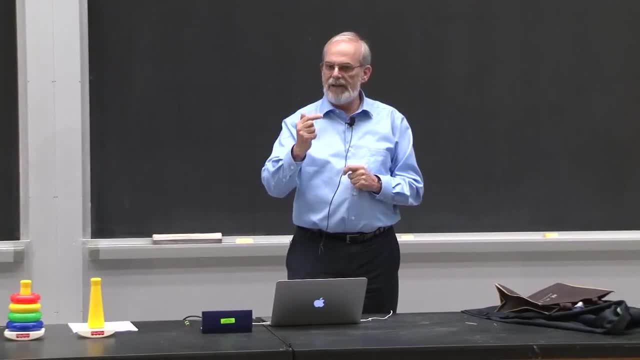 lead to what we would call iterative algorithms, And these algorithms can be described as being captured by a set of state variables, meaning one or more variables that tell us exactly the state of the computation. It's a lot of words. Let's look at an example. 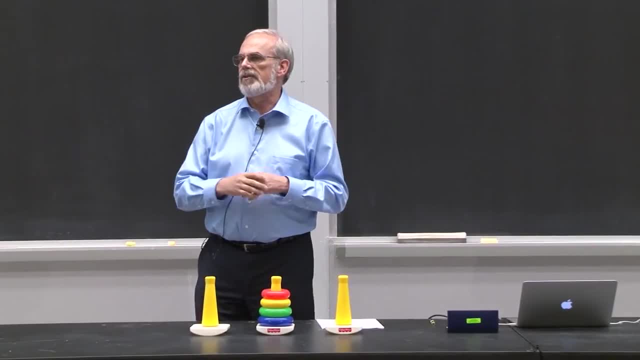 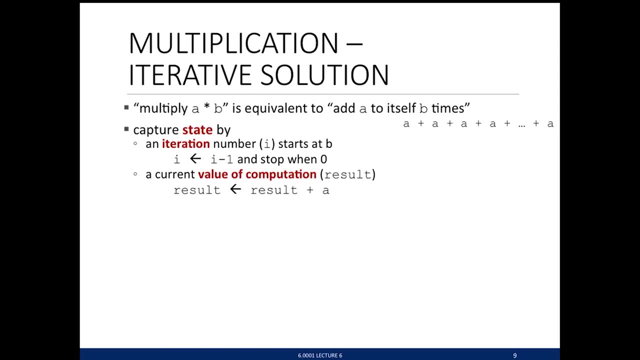 I know it's trivial, but bear with me. Suppose I want to do integer multiplication. multiply two integers together and all I have available to me is addition. So a times b is the same as adding a to itself, b times, If I'm thinking about this iteratively. 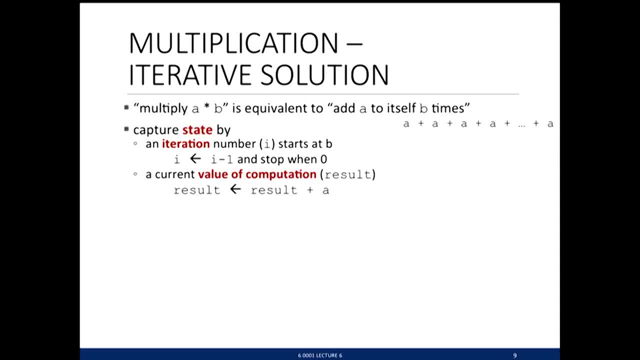 I could capture this computation with two state variables. One would just call the iteration number And it would be something, for example, that starts at b And each time through the loop reduces by one, And it will keep doing that until I've counted down b times. 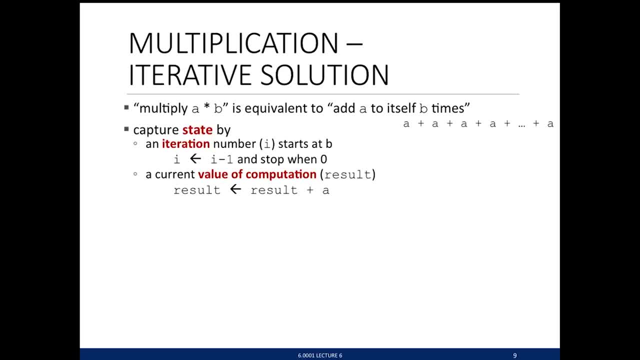 and I get down to 0. And at the same time I would have some value of the computation- I might call it result- which starts at 0,, first time through adds in a, next time through adds in a, And it just keeps track of how many things have I added up. 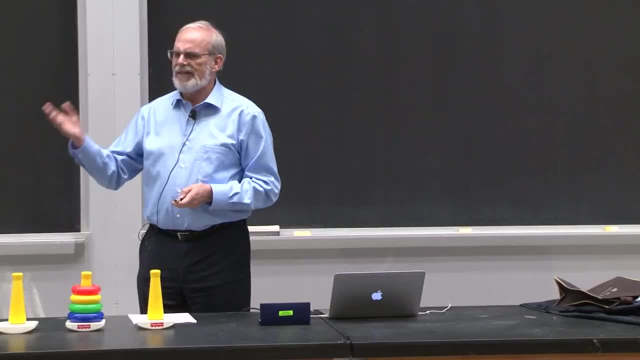 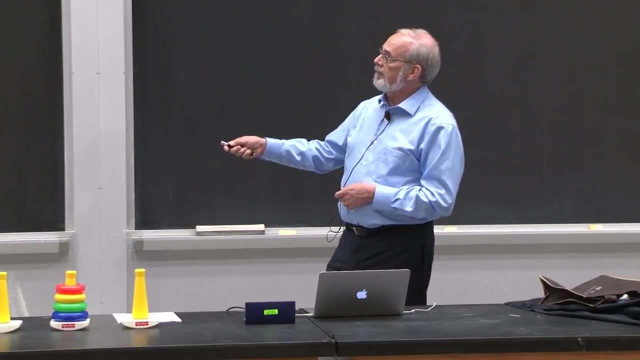 until I get done. And yeah, I know you could just do mult, but this is trying to get this idea of how would I do this iteratively. So I might start off with i saying there are b things still to add and result is 1.. 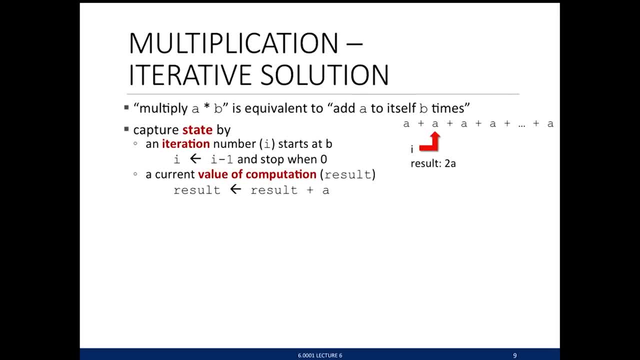 The first time through the loop, I add in a reduce i by 1.. Next time through the loop, I add in another a reduce i by 1.. And you get the idea. I just walked down it until eventually I got to the end of this computation. 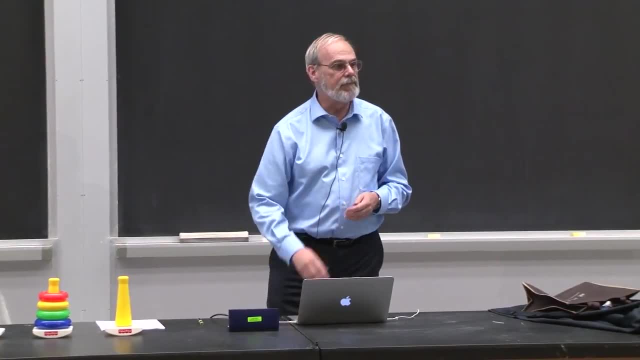 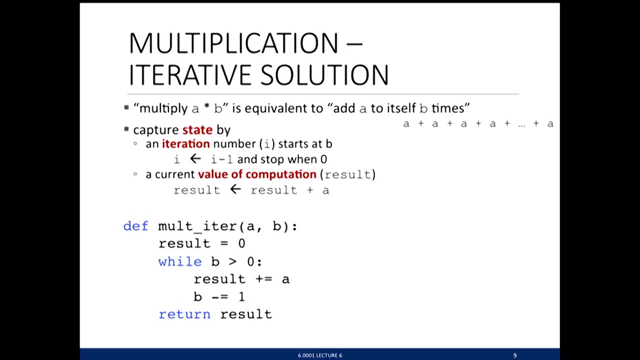 So we could write code for this, And actually it should be pretty straightforward. There it is. I'm going to call it: mult iter Takes in two arguments, a and b, And I'm going to capture exactly that process. So notice what I do. 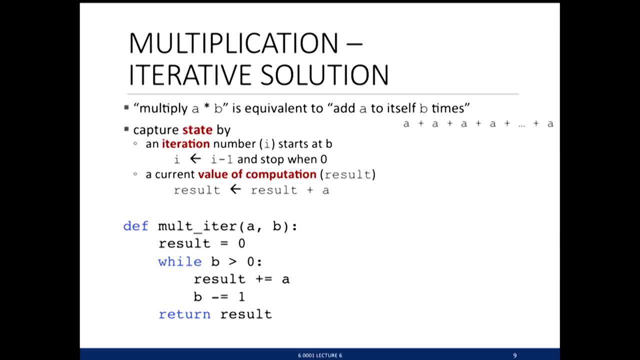 I set up result internally as just a little variable I'm going to use to accumulate things. And then there's the iteration: as long as b is greater than 0. What do I do? Add a to result, store it away, Reduce b by 1.. 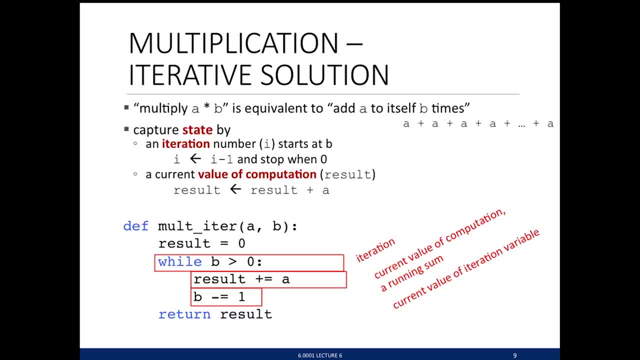 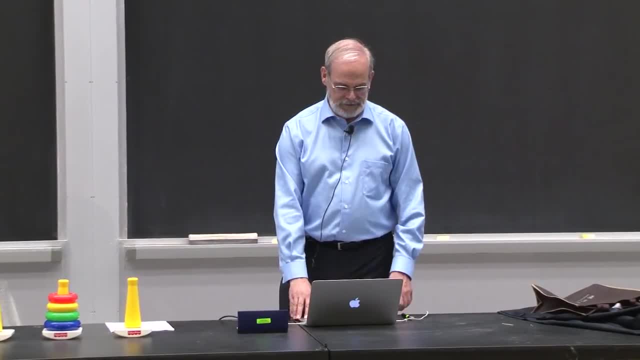 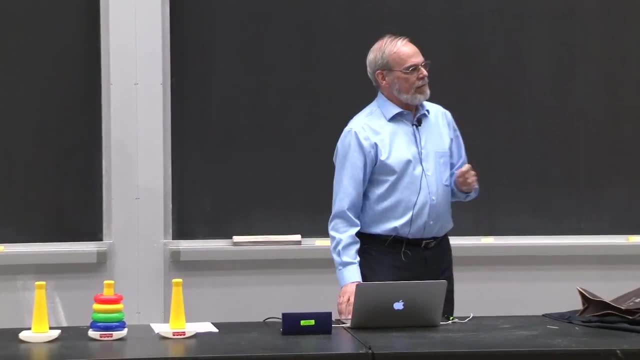 And I'll keep doing that until b gets down to being equal to 0,, in which case I just return the result. OK, Simple solution. Now let's think about this a different way. A times b is just adding a to itself, b times. 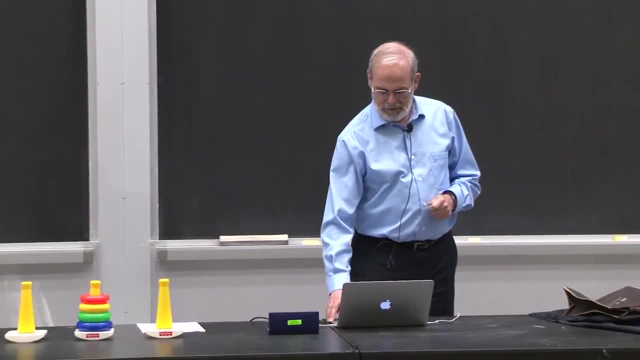 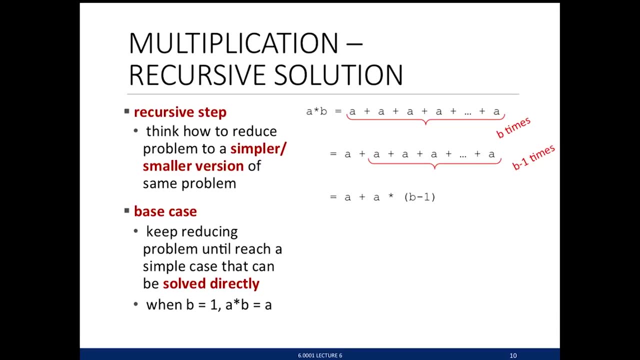 And that's the same as a plus adding a to itself: b minus 1 times. OK, that sounds like leisure domain, That sounds like just playing with words, But it's really important, because what is this? Ah, that's just a times b minus 1,. 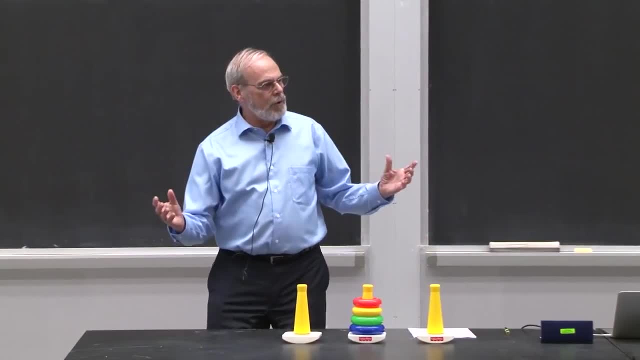 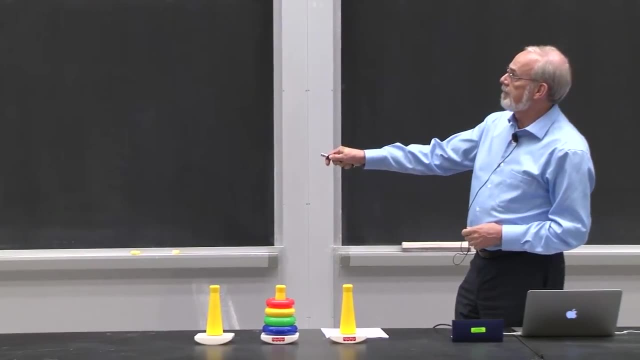 by the definition at the top point, And I know you're totally impressed. but this is actually really cool, Because what have I done? I've taken one problem, this one, up here and I've reduced it to a simpler version of the same problem. 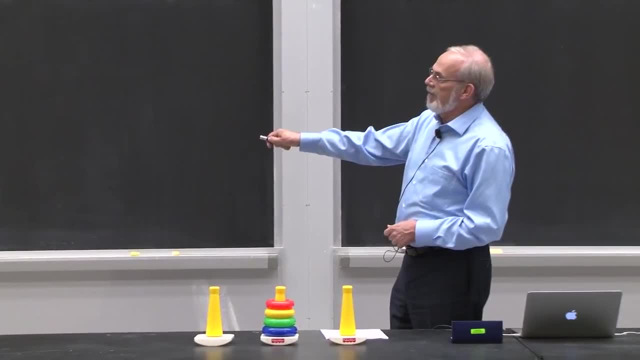 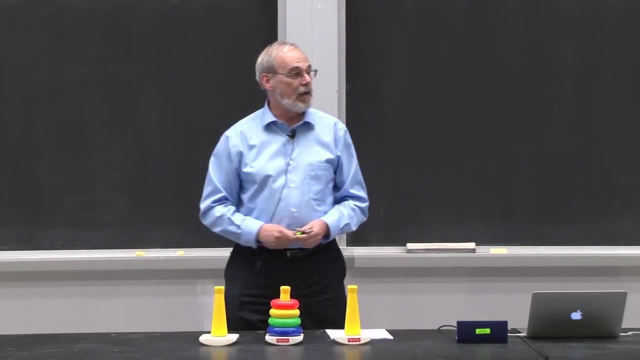 Plus some things I know how to do. And how would I solve this Same trick, That's a times a times b minus 2.. I would just unwrap it one more time And I would just keep doing that until I get down to something. 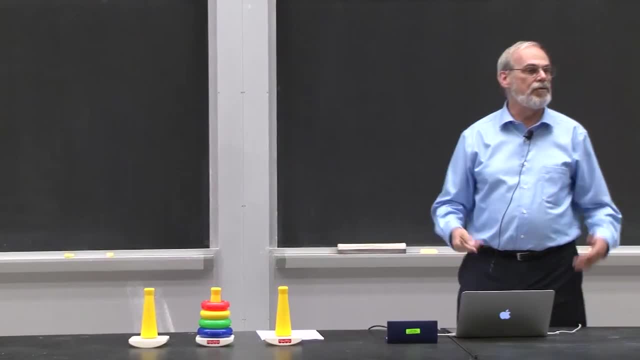 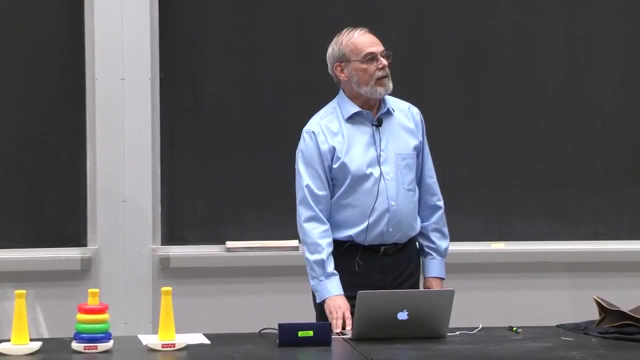 I can solve directly a base case, And that's easy. When b is equal to 1, the answer is just a. Or I could do: when b is equal to 0, the answer is just 0. And there's code to capture that. 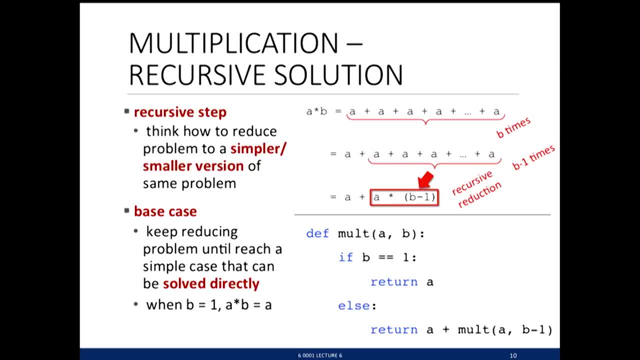 Different form, Wonderful, Compact description. What does it say? It says: if I'm at the base case, if b is equal to 1, the answer is just a. Otherwise, I'm going to solve the same problem with a smaller version and add it to a. 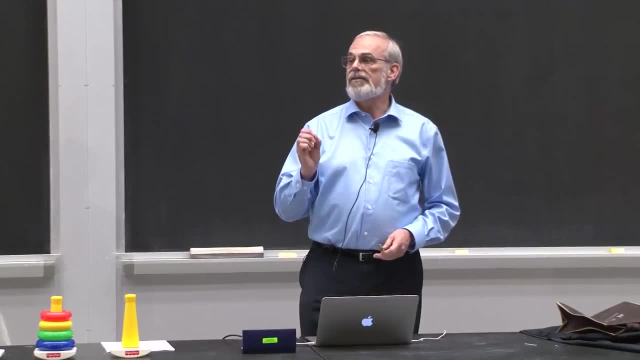 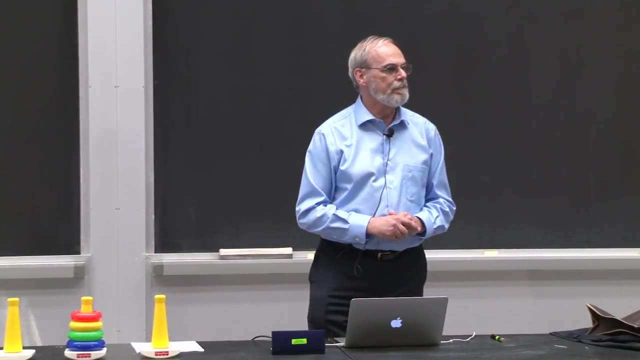 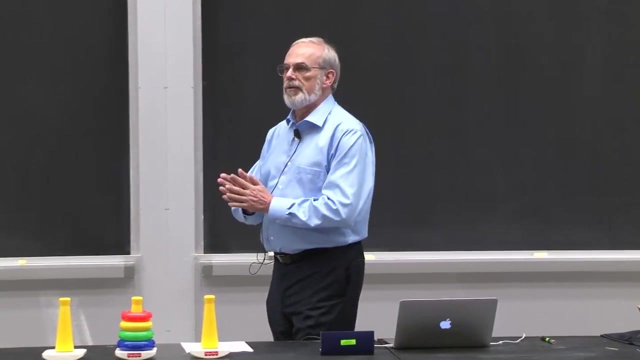 and return that result. And that's nice. crisp characterization of a problem. Recursive definition that reduces a problem to a simpler version of the same problem. OK, Let's look at another example. Classic problem in recursion is to compute factorial right. 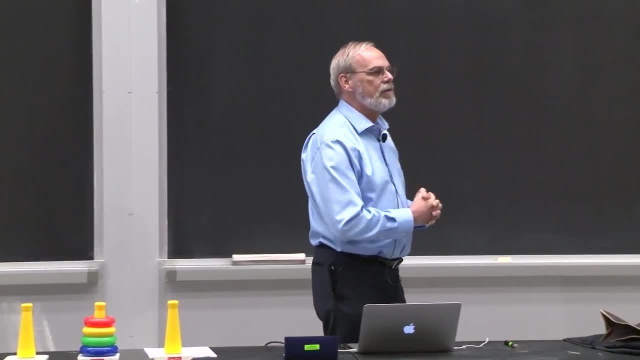 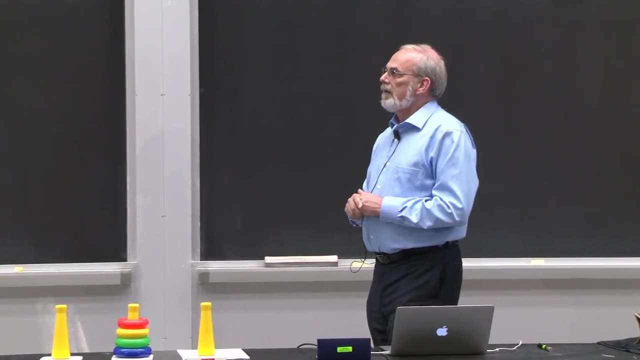 n factorial, or n bang if you like, and exclamation point is n times n minus 1, all the way down to 1.. So it's the product of all the integers from 1 up to n, assuming n is a positive integer. 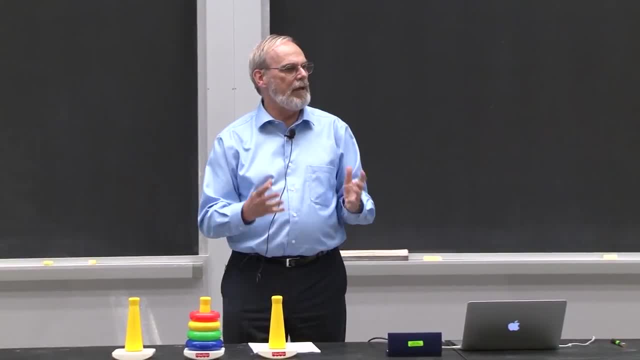 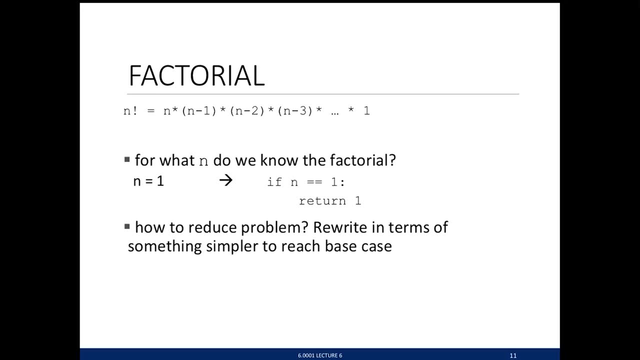 So we can ask the same question. If I wanted to solve this recursively, what would the base case be? Well, when n is equal to 1, it's just 1.. In the recursive case, well, n times n minus 1, all the way. 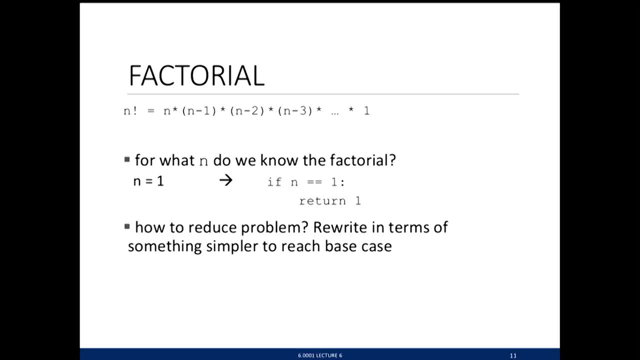 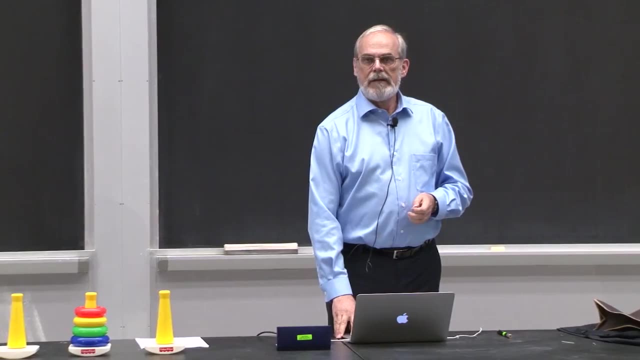 down to 1.. And that's the same as n times n minus 1 factorial. So I can easily write out the base case And I've got a nice recursive solution to this problem. OK, If you're like me- and this is the first time you see it- 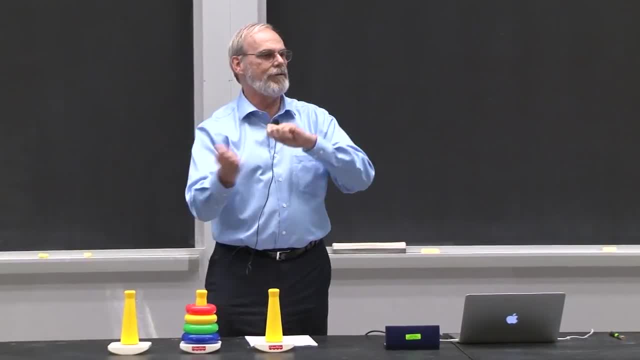 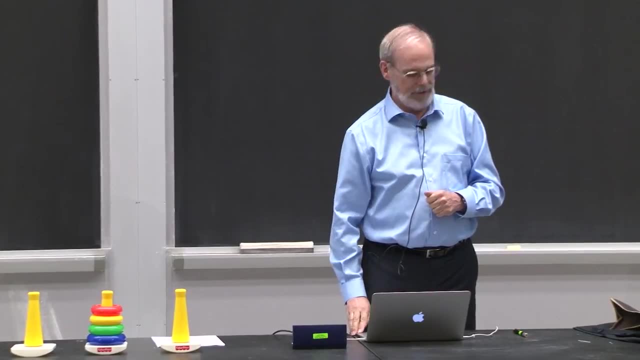 it feels like I've taken your head and twisted it about 180 degrees. I'm going to take it another 180 degrees Because you might be saying: well, wait a minute. How do you know what really stops, How do you know what really terminates the computation? 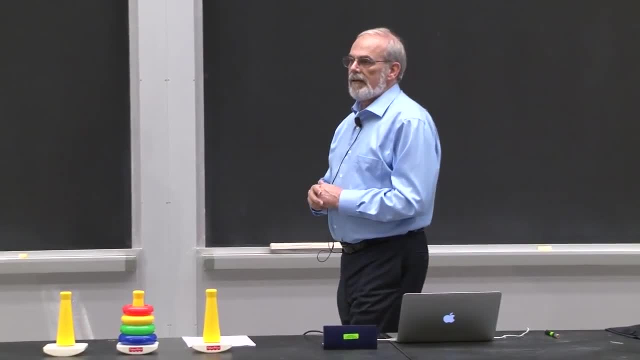 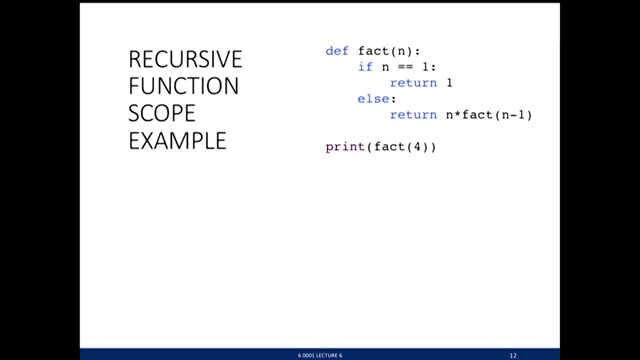 How do you know what really ends the computation? So let's look at it. There's my definition for fact, short for factorial. Fact of n is: if n is equal to 1, return 1.. Otherwise, return n times fact of n minus 1.. 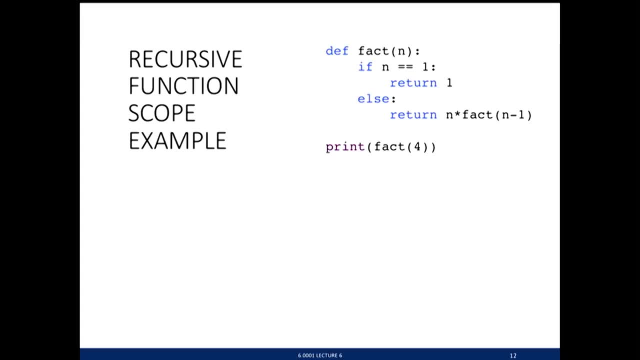 And let's use the tools that Anna talked about in terms of an environment at a scope and think about what happens here. So when I read that in or I evaluate that in Python, it creates a definition that binds the name fact to some code. 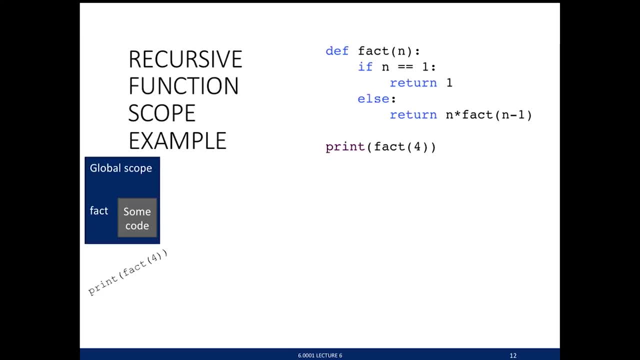 just all of that stuff over here. the name for the formal parameter Hasn't done anything with it yet. And then I'm going to evaluate print of fact of 4.. Print needs a value, so it has to get the value of fact of 4.. 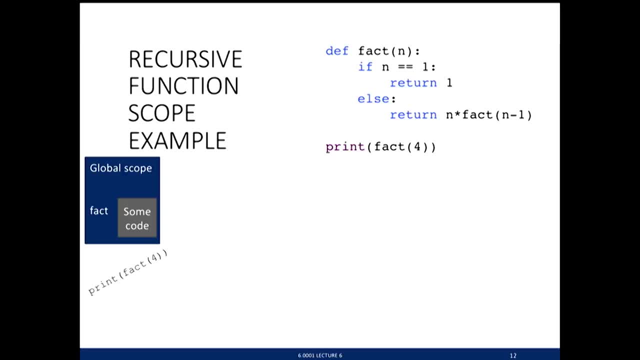 And we know what that does. It looks up fact. There it is its procedure definition. So it creates a new frame, a new environment. It calls that procedure And inside that frame, the formal parameter for fact is bound to the value passed in. 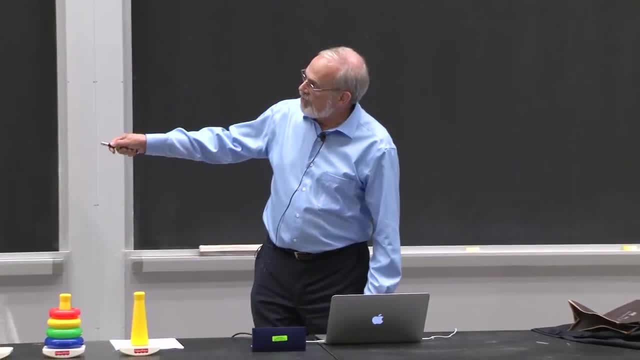 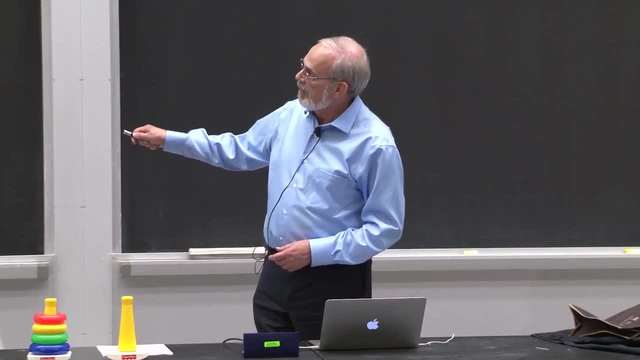 So n is bound to 4.. That frame is scoped by this global frame, meaning it's going to inherit things in the global frame. And what does it do? It says, inside of this frame, evaluate the body of fact. OK, so it says, is n equal to 1?? 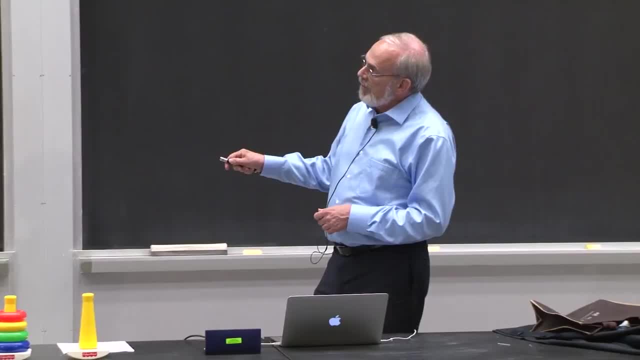 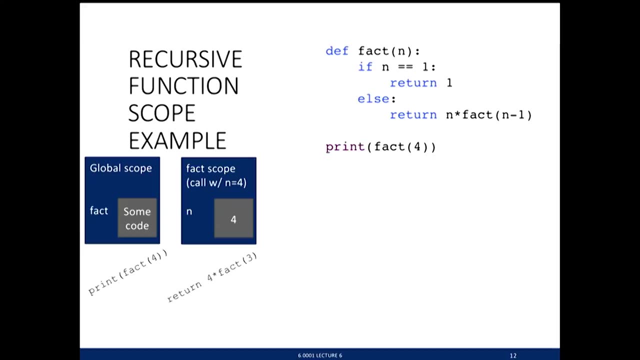 Nope, it's not, It's 4.. So in that case, go to the else statement And it says: oh, return n times fact of n And n is 4.. Fact of n minus 1 says I need to return 4 times fact of 3.. 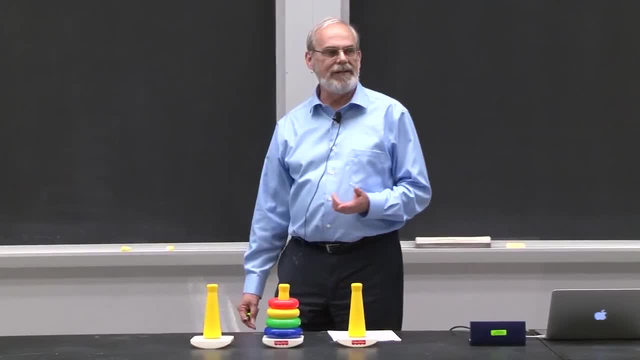 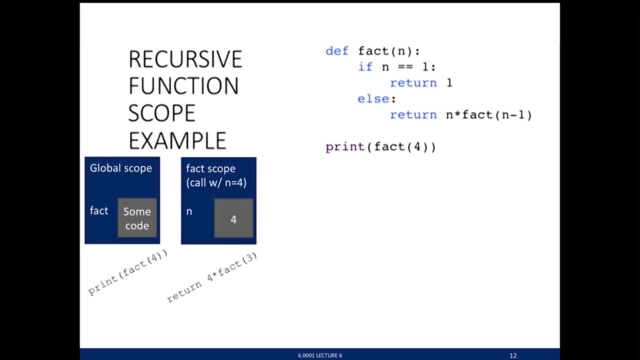 4 is easy, Multiplication is easy. Fact of 3,. ah, yes, I look up fact. Now I'm in this frame. I don't see fact there, But I go up to that frame. There's the definition for fact. 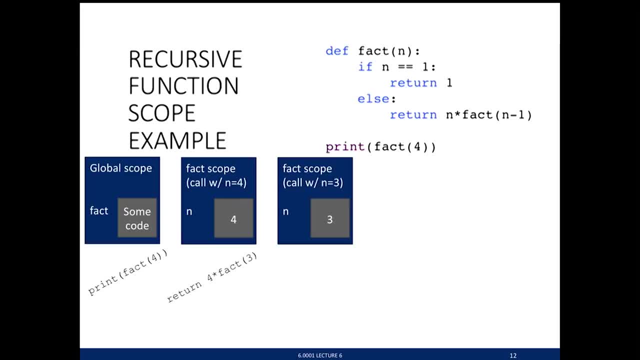 And we're going to do the rest of this a little more quickly. What does that do? It creates a new frame called by fact, And the argument passed in for n is n minus 1, that value, right there, of 3.. So 3 is now bound to n. 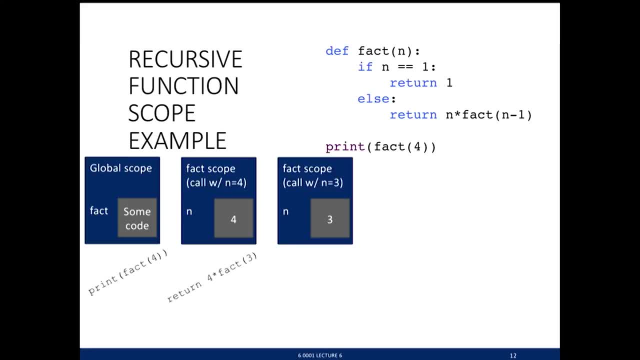 Same game: Evaluate the body. Is n equal to 1? No, So in that case I'm going to go to the return statement. It says: return 3 times fact of 2.. And notice it's only looking at this value of n. 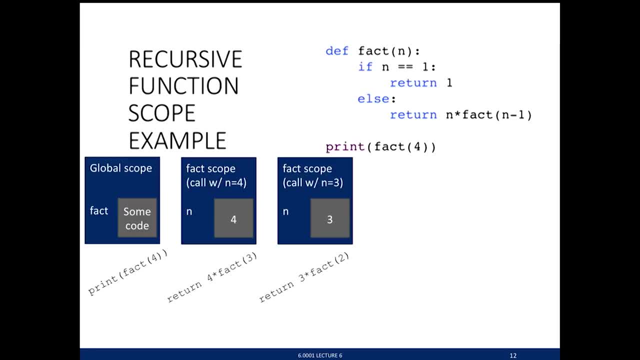 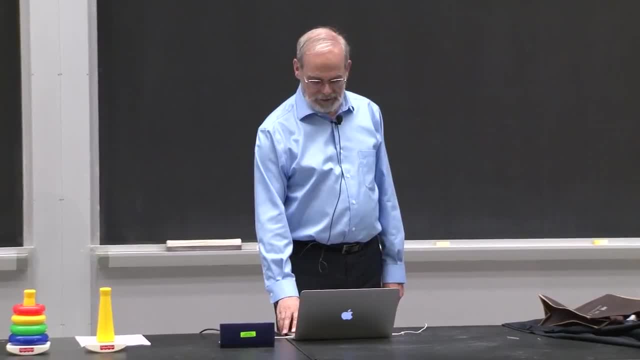 because that's the frame in which I'm in. It never sees that value of n. OK, aren't you glad I didn't do fact of 400? We've only got two more to go, But you get the idea. Same thing. 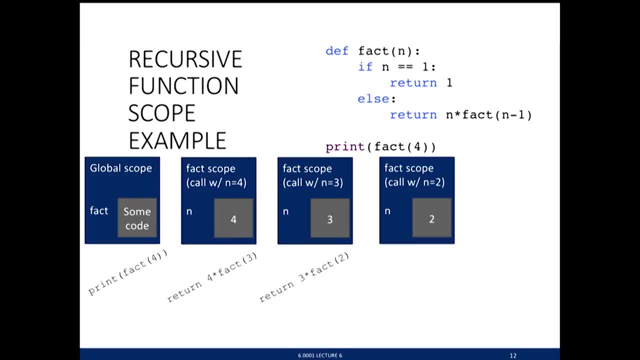 I need to get fact of 2.. It's going to call fact again with n bound to 2.. Relative to that evaluates the body n is not yet equal to 1.. That says I'm going to the else clause and return 2 times fact. 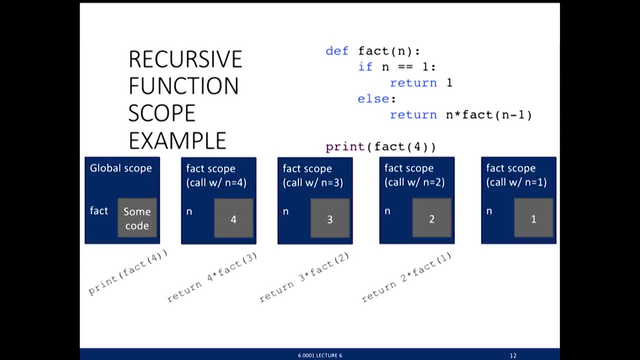 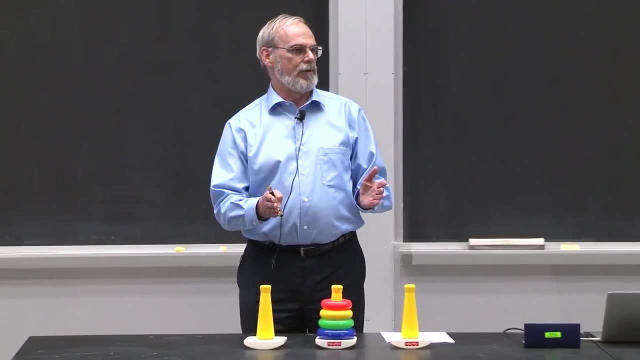 of 1.. I call fact again now, with n bound to 1.. And fortunately now that clause is true And it says return 1.. Oops, sorry, before I do So, there's the base case And it may seem apparent to you, but this is important. 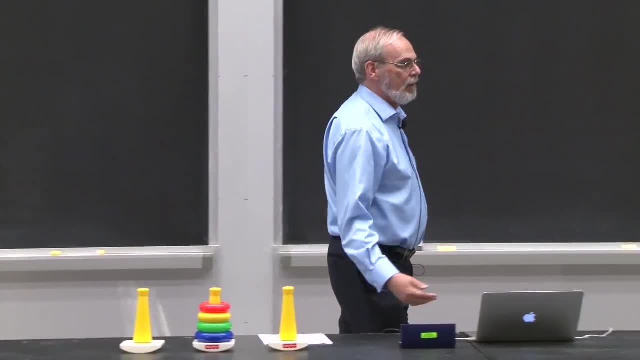 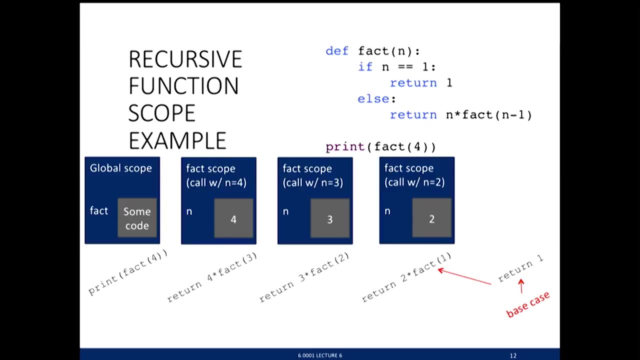 I'm unwinding this till I get to something that can stop the computation. Now I'm simply going to gather the computation up, because it says: return 1.. Who asked for it? Well, that called a fact of 1. So that reduces to return. 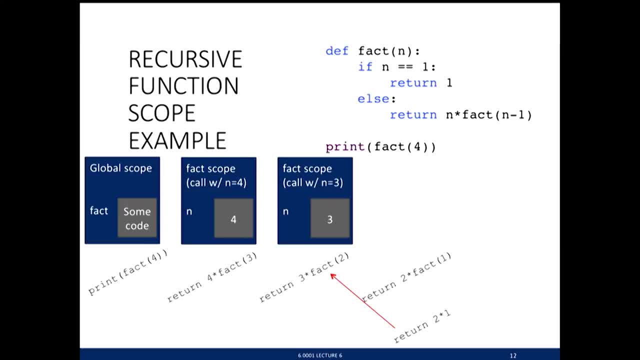 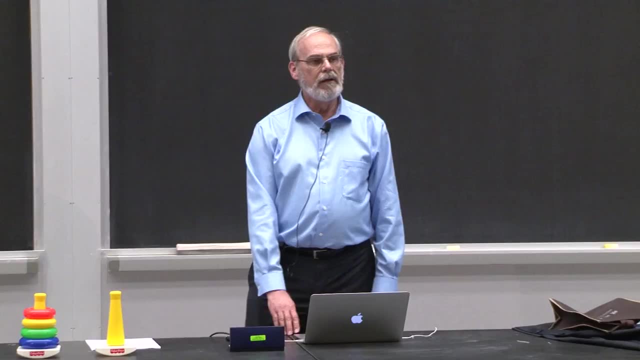 Return 2 times 1.. And who called for that Fact of 2.. That reduces to return of 3 times 2, which reduces to 4 times 6,, which reduces to printing out 24.. So it unwinds it down to a base case and it stops. 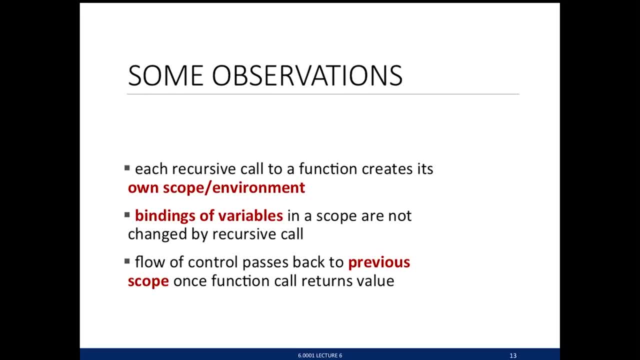 Couple of observations. Notice how each recursive call creates its own frame And, as a consequence, there's no confusion about which value of n I'm using. Also notice In the other frames: n was not changed. We did not mutate it. 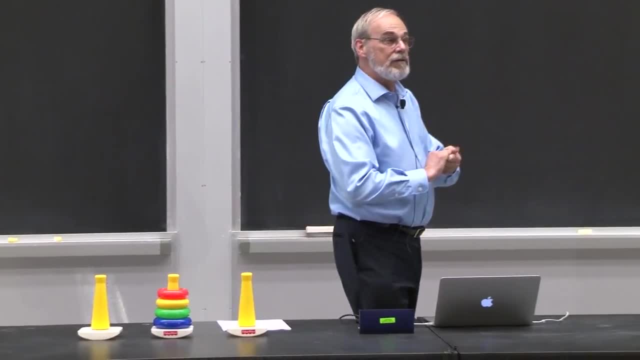 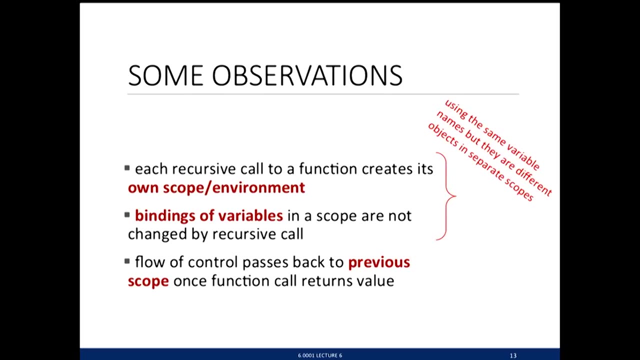 So we're literally creating a local scope for that recursive call, which is exactly what we want. Also, notice how there was a sense of flow of control In computing. fact of something that reduces to returning n times. fact of n minus 1.. 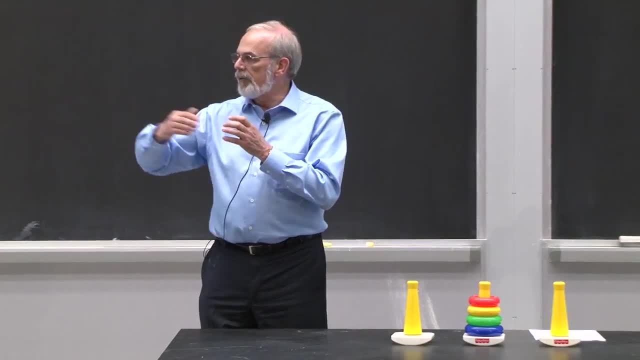 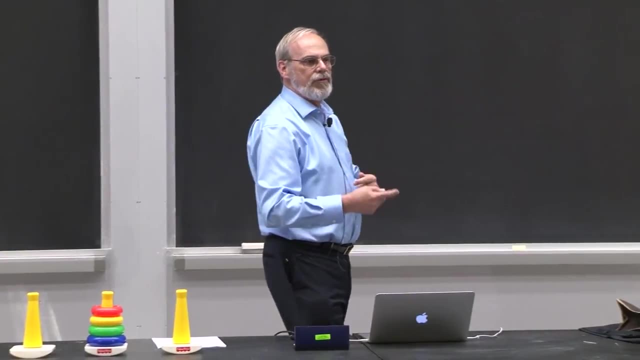 And that creates a new scope, And that will simply keep unwinding until I get to something that can return a value, And then I gather all those frames back up. So there's a natural flow of control here, But, most importantly, there's no confusion. 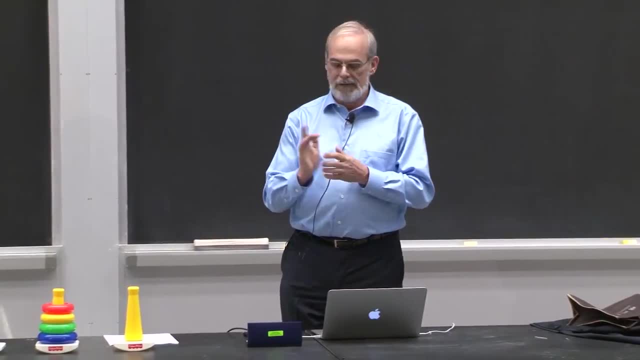 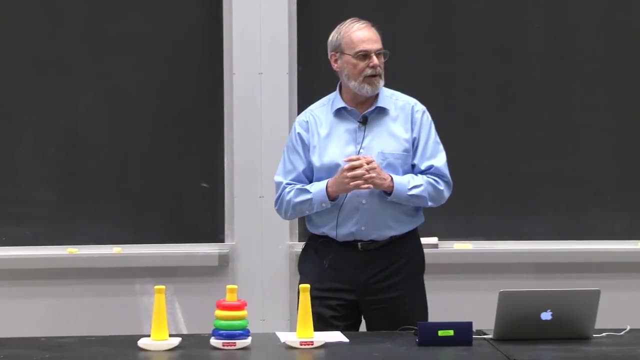 about which variable I'm using when I'm looking for a value of n, Because this is often a place where things get a little confusing. I want to do one more example, But let me first show you side by side the two different versions of factorial. 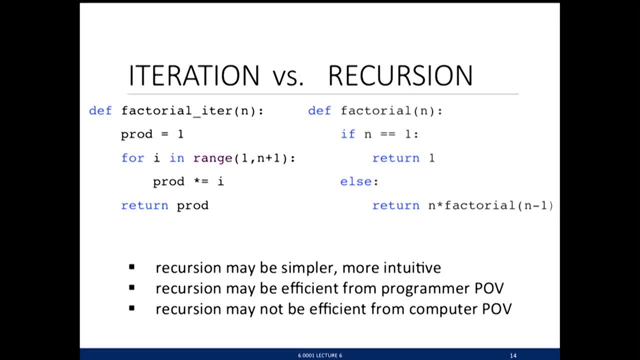 Actually I lied slightly. We didn't show this one earlier, But there's factorial. if I wanted to do it iteratively, I'd set up some initial variable to 1. And then I'd just run through a loop, for example from 1 up. 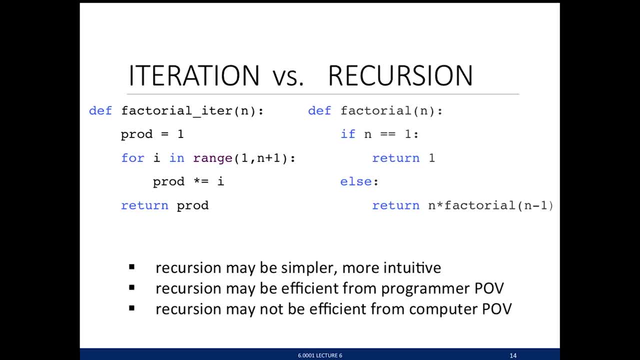 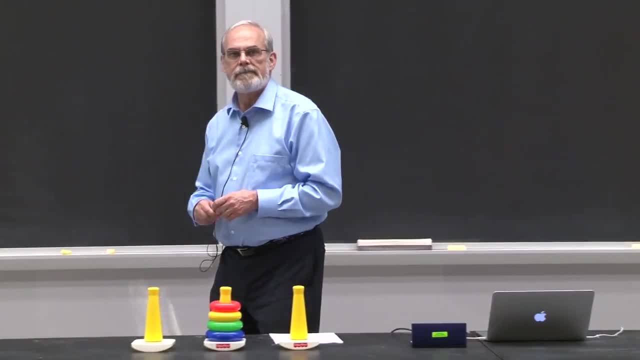 to just below n minus 1, or 1 up to n Or 1 up to n, multiplying it and putting it back into return product. Which one do you like more? You can't say neither, You have to pick one. 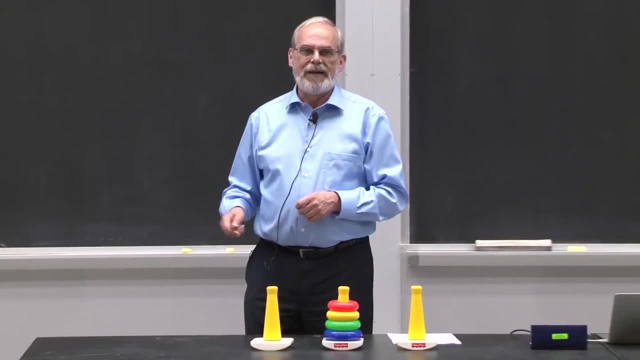 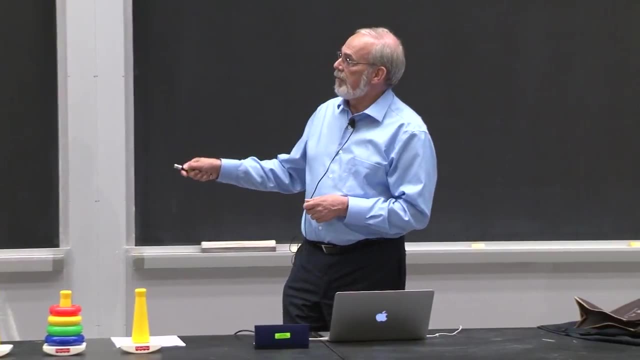 Show of hands. how many of you like this one? Some hesitant ones? How many prefer this one? Yeah, That's my view. I'm biased, But I really like the recursive one. It is crisper to look at. You can see what it's doing. 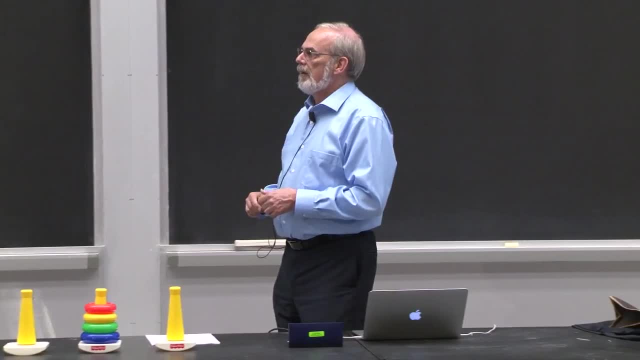 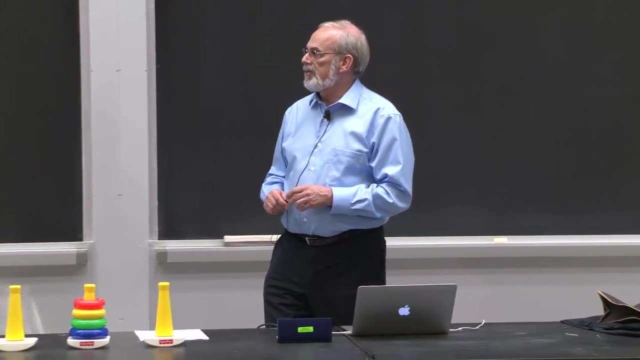 I'm reducing this problem to a simpler version of that problem. Pick your own version, But I would argue that the recursive version is more intuitive to understand. From a programmer's perspective, it's actually often more efficient to write because I don't have to think about interior variables. 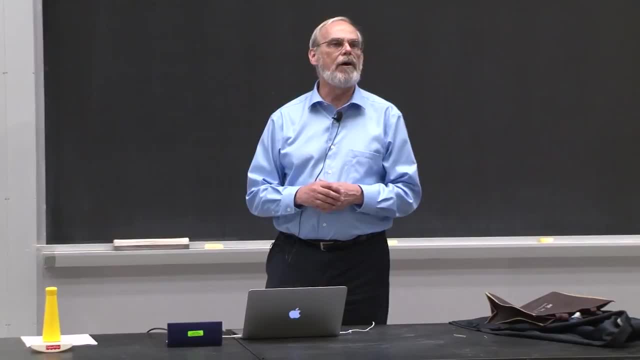 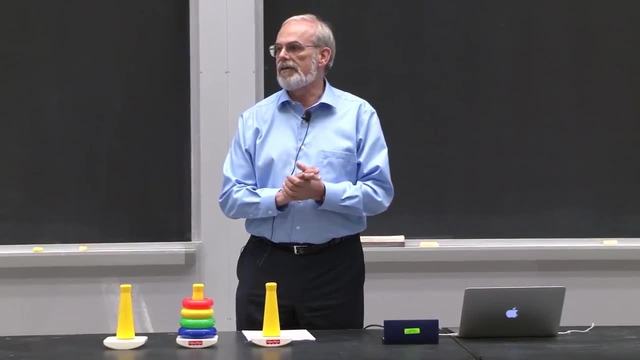 Depending on the machine, it may not be as efficient when you call it, Because in the recursive version I've got to set up that set of frames And some versions of these languages are actually very efficient about it, Some of them a little less so. 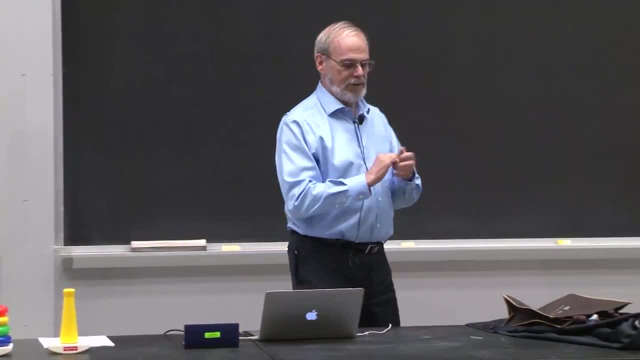 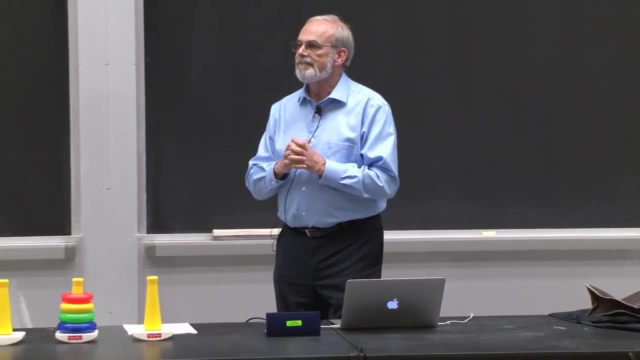 But given the speed of computers today, who cares? as long as it actually just does the computation, All right. One more example: How do we really know our recursive code works? Well, we just did a simulation. But let's look at it one more way. 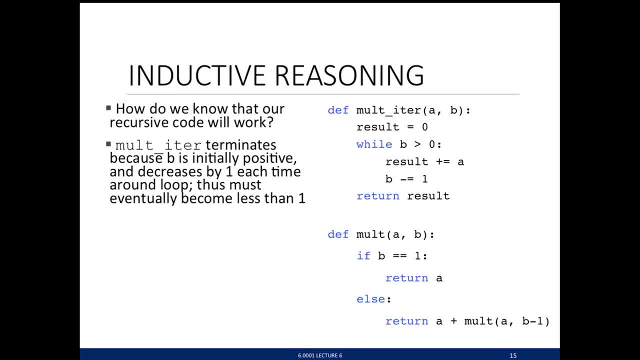 The iterative version. what can I say about it? Well, I know it's going to terminate. because b is initially positive- assuming I gave it an appropriate value- It decreases by 1 every time around this loop. At some point it has to get less than 1.. 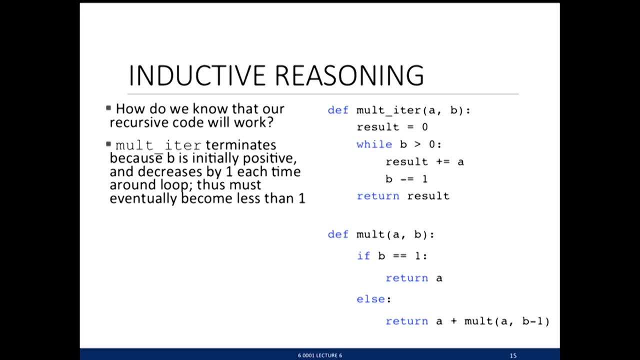 It's going to stop, So I can conclude it's always going to terminate. What about the recursive version? Well, if I call it with b equal to 1, I'm done. If I call it with b greater than 1,. 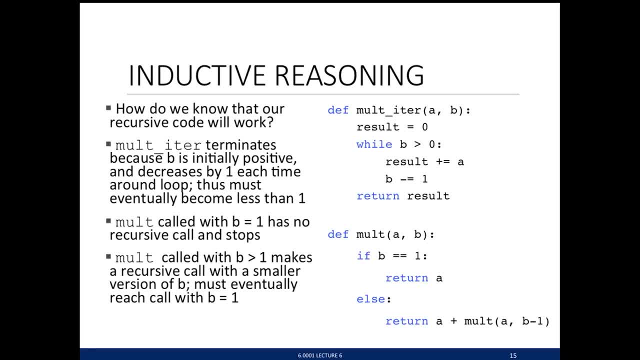 again, it's going to reduce it by 1 on the recursive call, which means on each recursive call it's going to reduce it. Eventually it gets down to a place- assuming I gave it a positive integer- where b is equal to 1.. 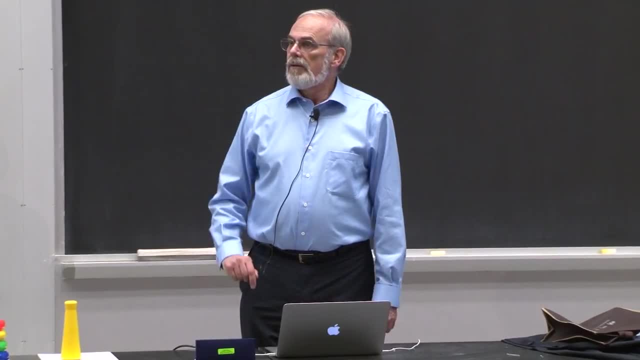 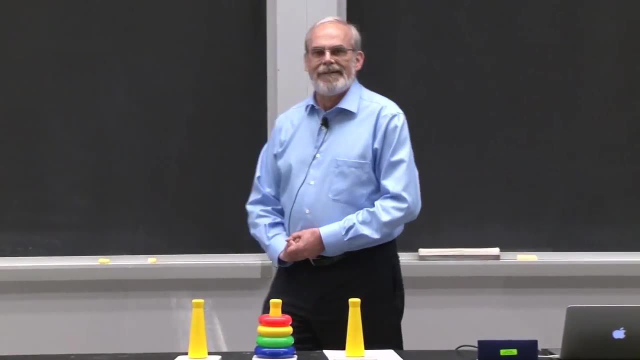 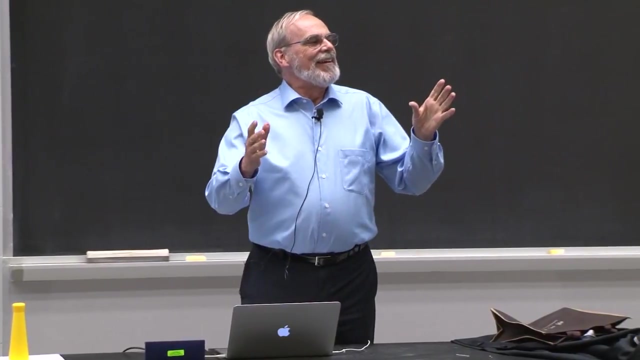 So it'll stop, which is good. What we just did was we used a great tool from math, second best department at MIT. Wow, I didn't even get any hisses on that one, John. All right, And I'm now in trouble with the head of the math department. 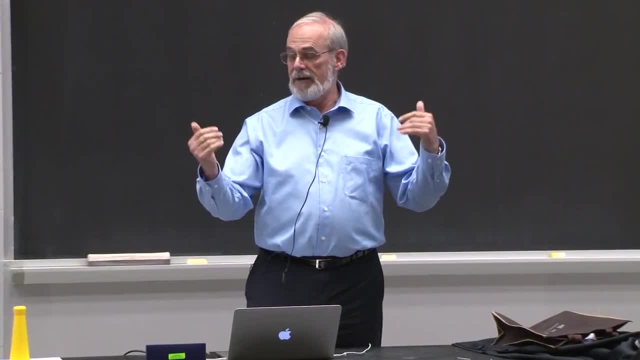 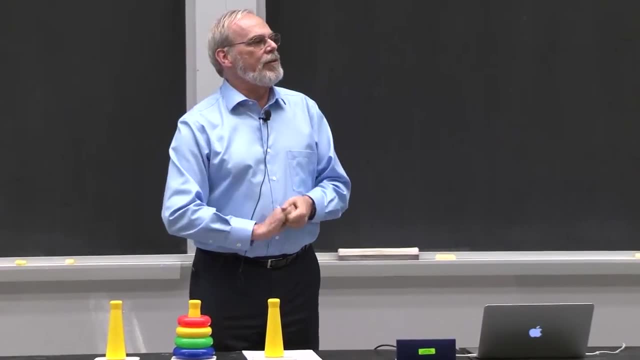 So now that I got your attention- and yes, all computer science jokes are bad and mine are really bad, but I'm tenured, You cannot do a damn thing about it- Let's look at mathematical induction, which turns out to be a tool that lets us think about programs. 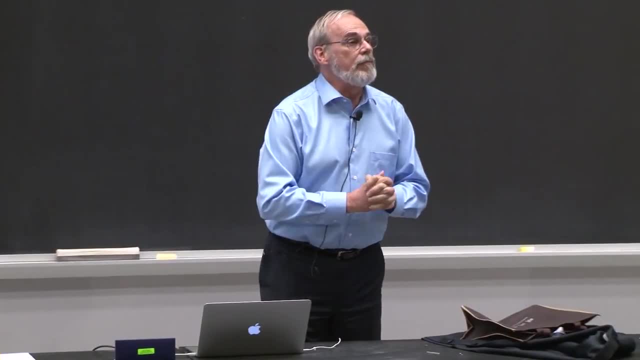 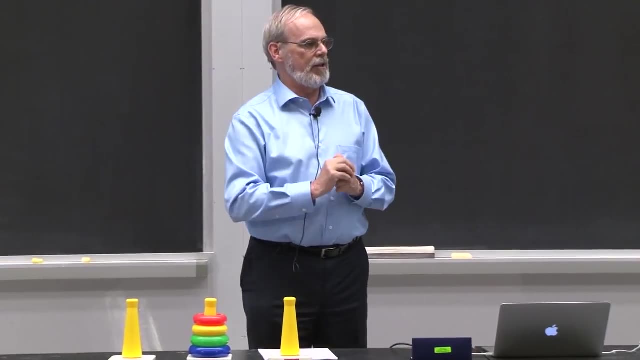 in a really nice way. If you haven't seen this, here's the idea of mathematical induction, If I want to prove a statement, and we refer to it as being indexed on the integers. In other words, it's some mathematical statement. 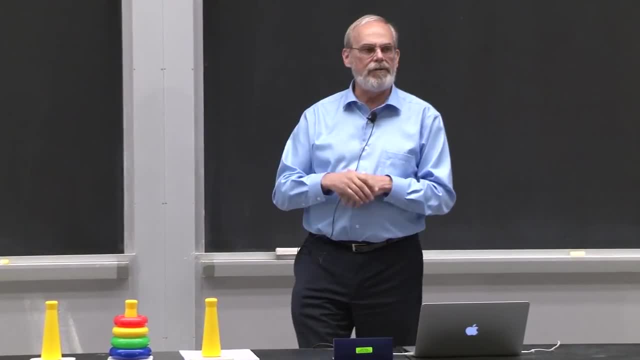 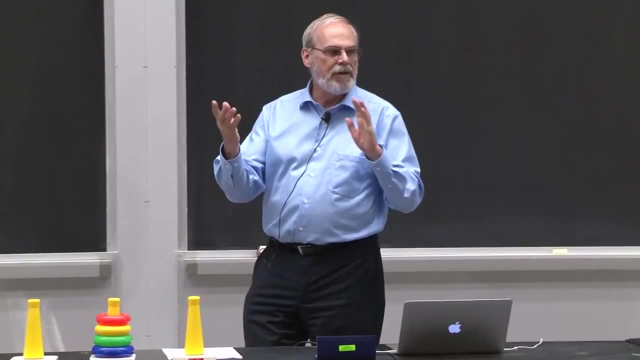 that runs over integers. If I want to prove it's true for all values of those integers, mathematically, I do it by simply proving it's true for the smallest value of n. Typically, n is equal to 0 or 1.. 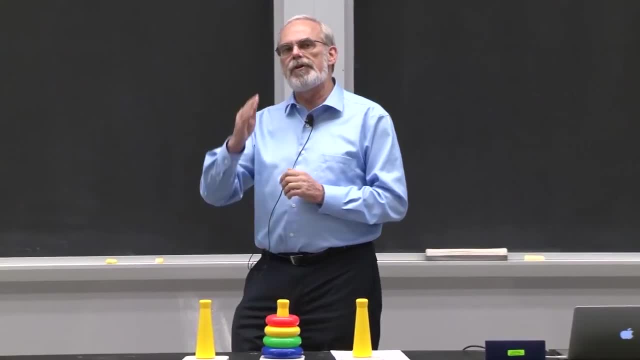 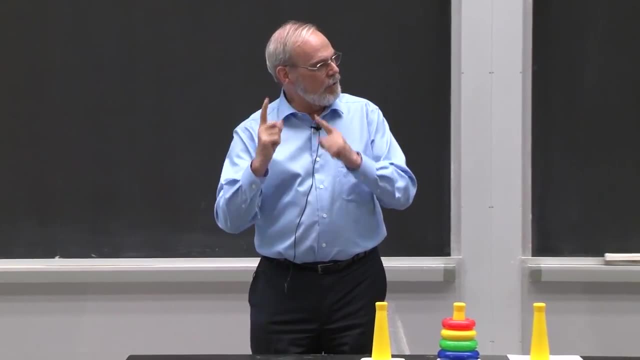 And then I do an interesting thing. I say I need to prove that if it's true for an arbitrary value of n, I'm just going to prove that it's also then true for n plus 1.. And if I can do those two things, I can then conclude: 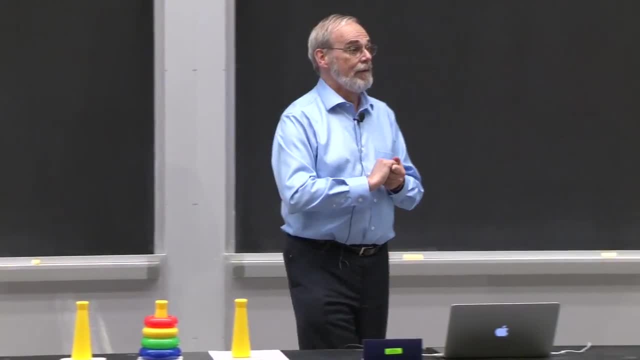 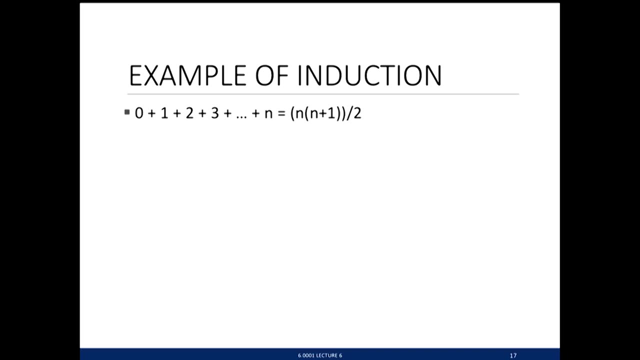 for an infinite number, For an infinite number of values of n. it's always true. I'm going to relate it back to programming in a second, but let me show you a simple example of this, one that you may have seen If I add the integers from 0 up to n, or even from 1 up to n. 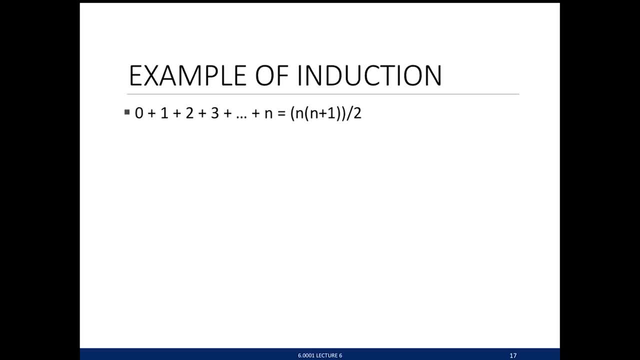 I claim that's the same as n times n, plus 1 over 2.. So 1,, 2, 3,, that's 6,. right, And that's exactly right. 3 times 4, which is divided by 2, which gives me out 6.. 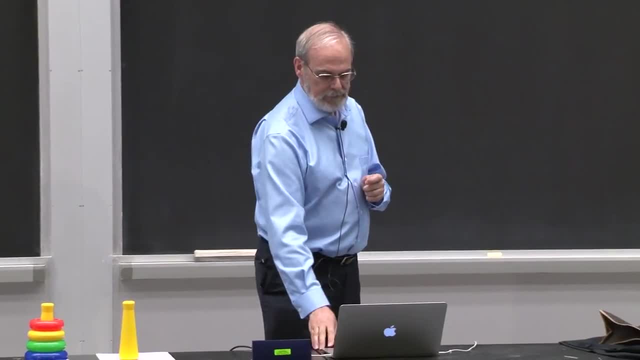 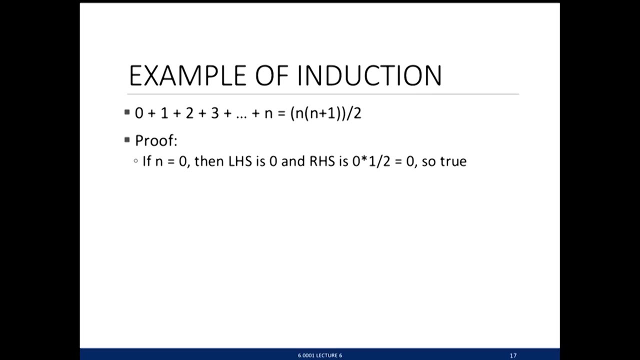 How would I prove this? Well, by induction. I need to do the simple cases. If n is equal to 0,, well then this side is just 0. And that's 0 times 1, which is 0 divided by true. 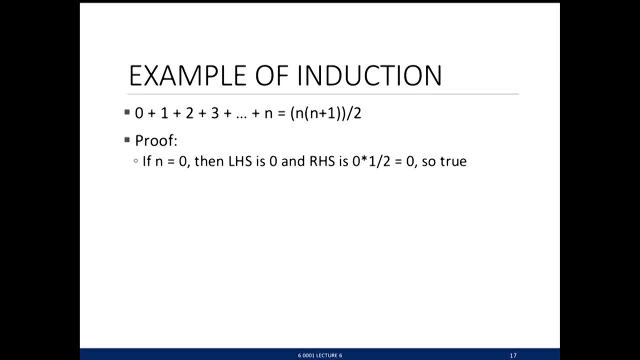 So 0 equals 0.. It's true. And now the inductive step. I'm going to assume it's true for some k- I should have picked n, but for some k. And then what I need to show is: it's true for k plus 1.. 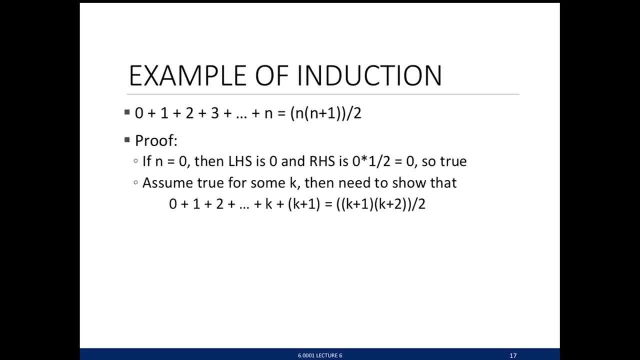 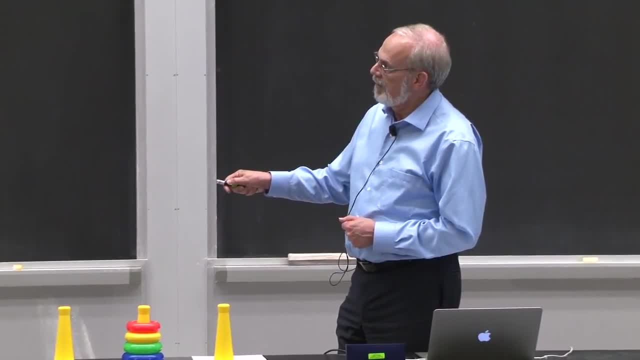 Well, there's the left-hand side, And I want to show that this is equal to that, And I'm going to do it by using exactly this recursive idea, Because, what do I know? I know that this sum in here, I'm assuming, is true. 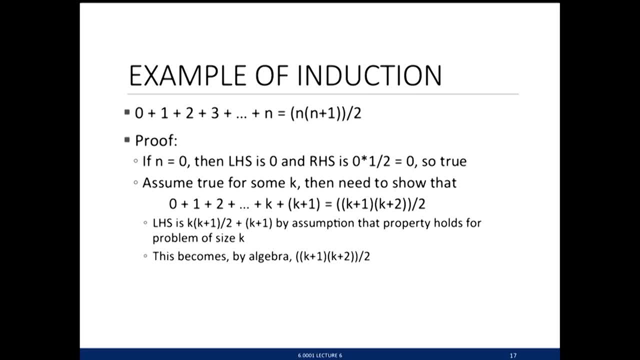 And so that says that the left-hand side, the first portion of it, is just k times k plus 1 over 2.. That's the definition of the thing I'm assuming is true. To that I'm going to add k plus 1.. 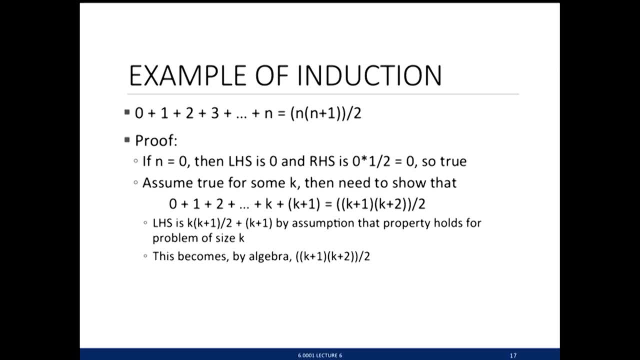 Well, you can do the algebra right. That's k plus 1, all times k over 2 plus 1, which is k plus 2 over 2.. Oh cool, It's exactly that. OK. Having done that, I can now conclude. 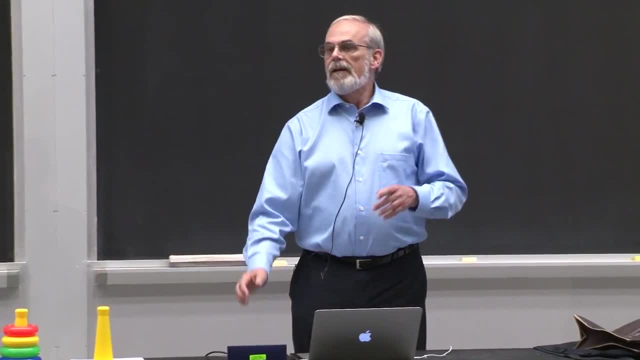 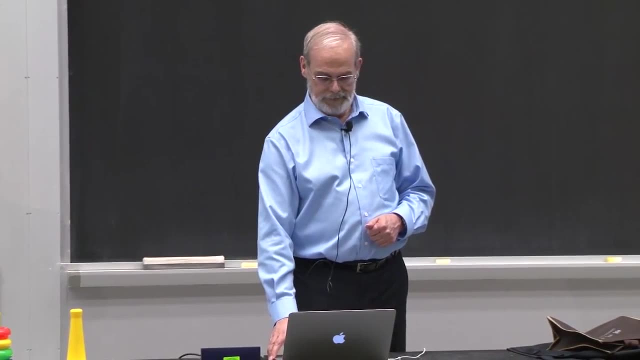 this is true for all values of n. What does it have to do with programming? That's exactly what we're doing when we think about recursive code. We're saying: show that it's true for the base case. And then what I'm essentially assuming. 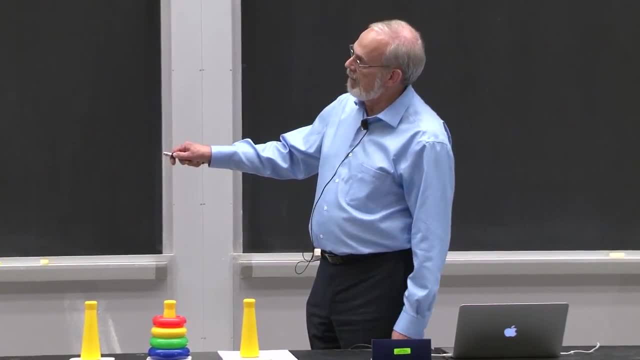 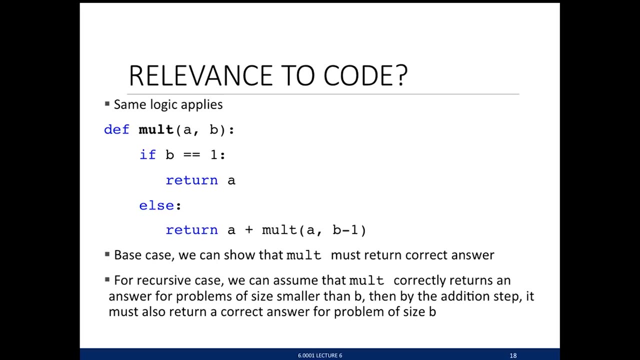 is that if it works for values smaller than b, then does the code return the right answer for b? And the answer is absolutely it does, And I'm using induction to deduce that in fact my code does the right thing. 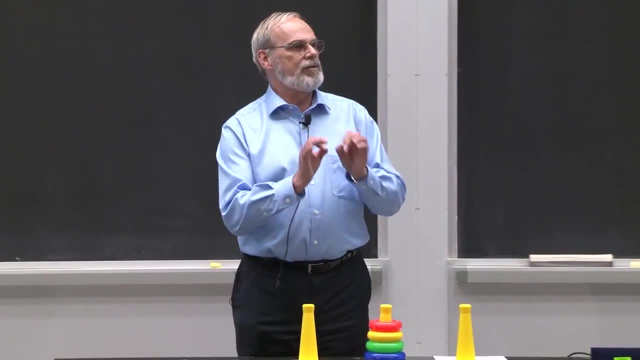 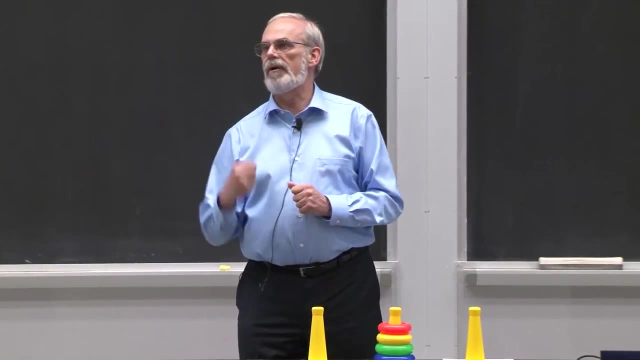 Why am I torturing you with this? Because this is the way I want you to think about recursion. When I'm going to break a problem down into a smaller version of the same problem, I can assume that the smaller version gives me the answer. 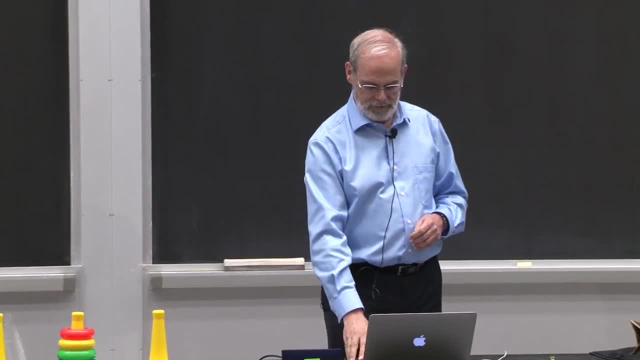 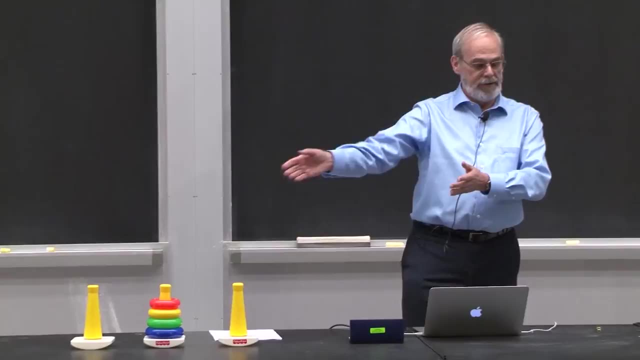 All I have to do is make sure that what I combine together gives me out the right result. OK, You may be wondering what I'm doing with these wonderful high-tech toys down here. I want to show you another example of recursion. So far, we've seen this. 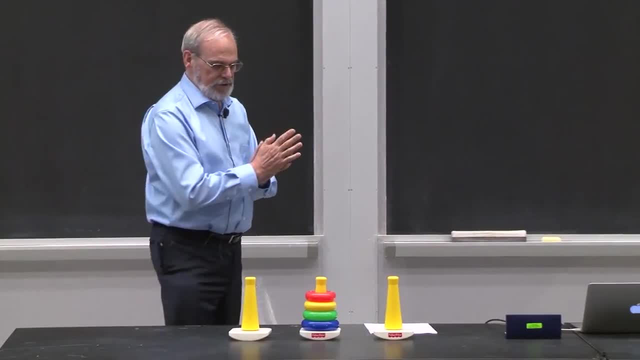 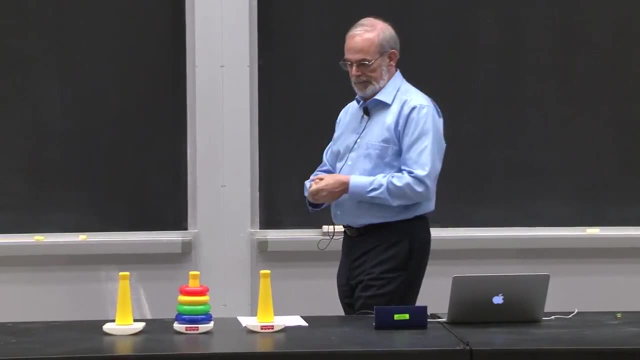 We've seen simple things that just have one base case, And this is a mythical story called the Towers of Hanoi, And the story, as I heard it, is: there's a temple somewhere in Hanoi with three tall spikes and 64 jewel-encrusted golden disks, all of a different size. 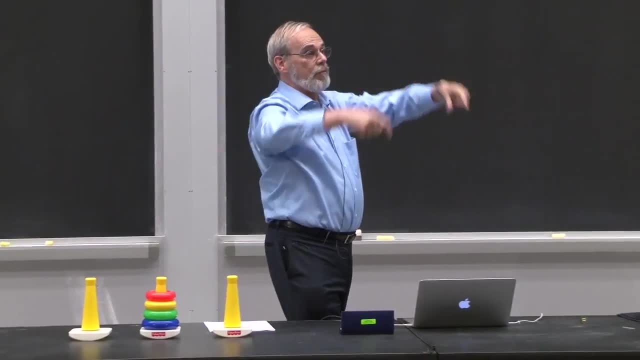 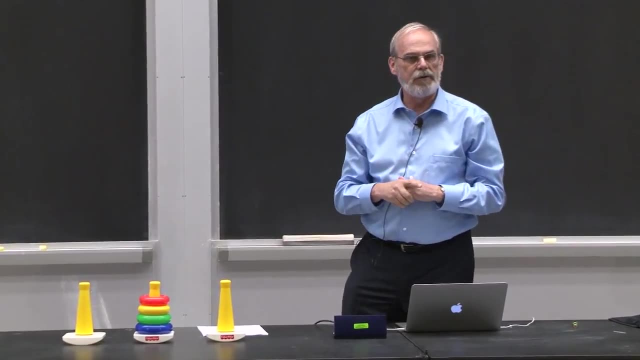 They all started out on one spike with the property that they were ordered from smallest down to largest. And there are priests in this temple who are moving the disks one at a time, one per second, And their goal is to move the entire stack from one spike. 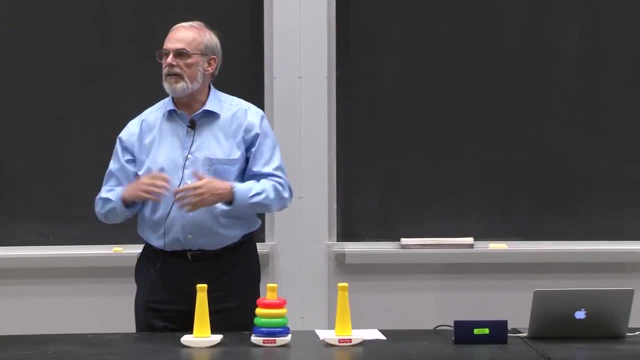 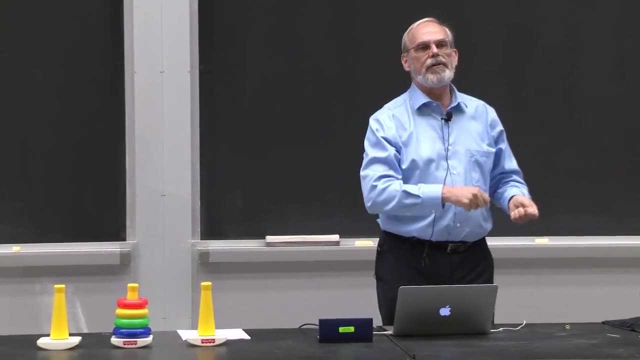 to another spike, And when they do, nirvana is achieved and we all get a really great life. We'll talk separately about how long it is going to take, because there's one trick to it: They can never cover a smaller disk with a larger disk. 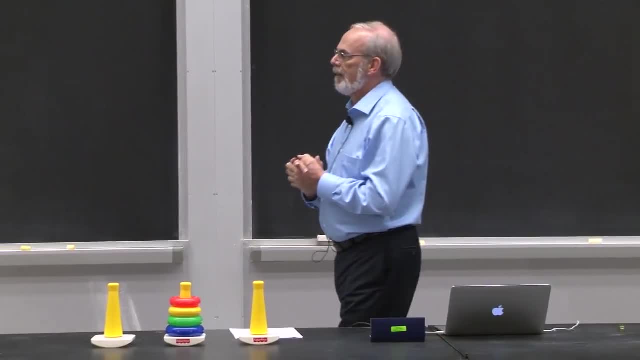 as they're doing it. So they got a third disk as a temporary thing And I want to show you how to solve this problem, because you're going to write code with my help in a second, or I'm going to write code with your help in a second. 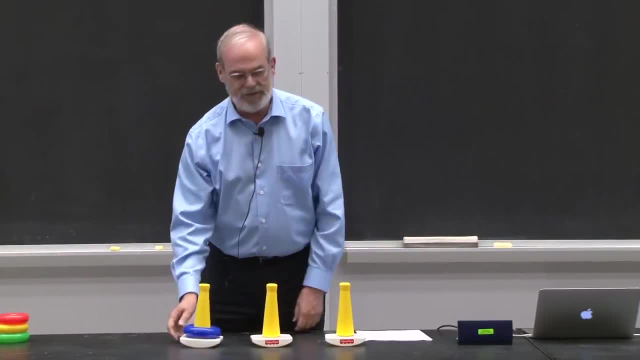 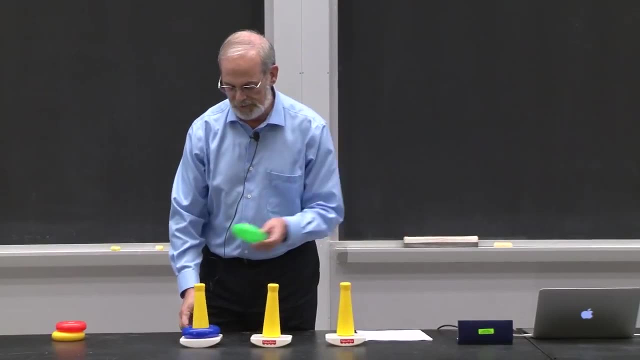 to solve it. So let's look at it. So watch carefully. Moving a disk a size 1, well, that's pretty easy, right. Moving a disk a size 2, well, just put this one on the spare one while you move it over. 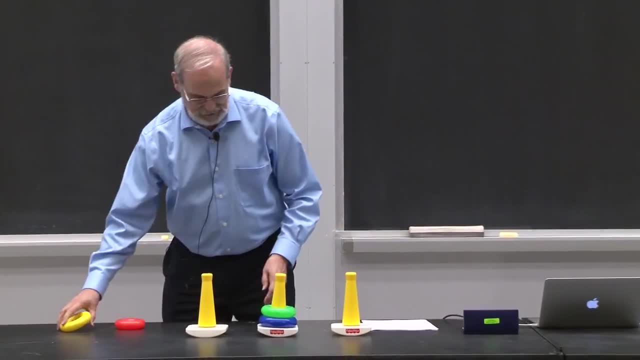 so you don't cover it up. That's easy Moving a disk a size 3, got to be a little more careful. You can't cover up a smaller one with a larger one, so you have to really think about where you're putting it. 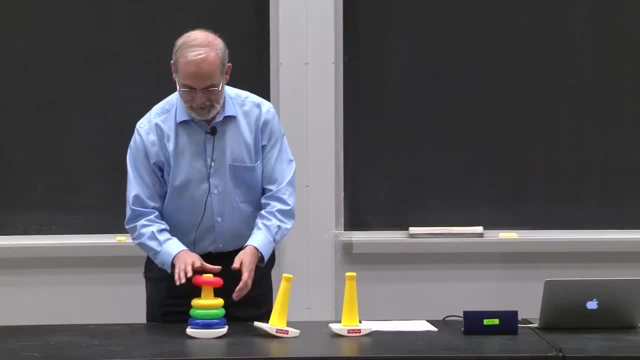 It would help if these things didn't juggle. And there you go, You got it done. All right, you're watching, Got to do 4.. To do 4, again, you've got to be really careful not to cover. 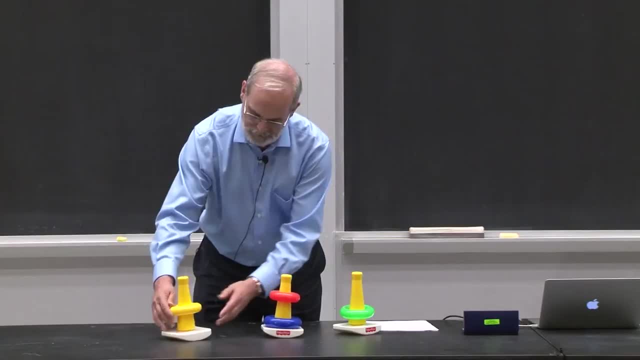 things up. as you do this, You want to get the bottom one eventually exposed, and so you're going to pull that one over there. If you do the patter really well, you won't notice if I make a serious mistake as I'm doing this, which I just did. 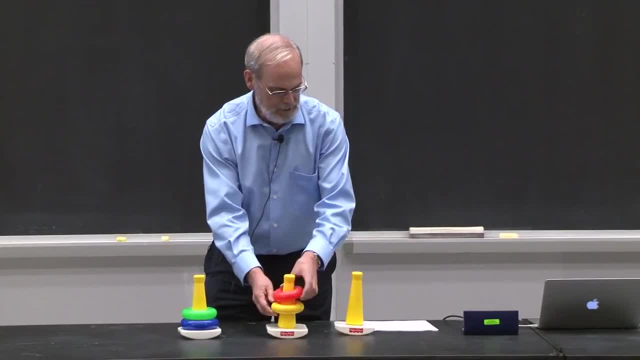 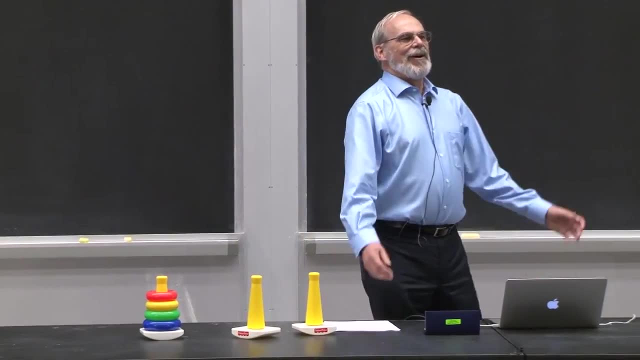 But I want to recover from that and do it that way, to put this one over here And that one goes there, And if I did this in Harvard Square I could make money There. you go right. OK, got the solution. 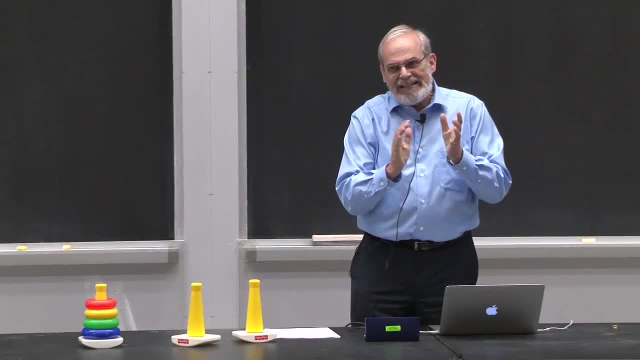 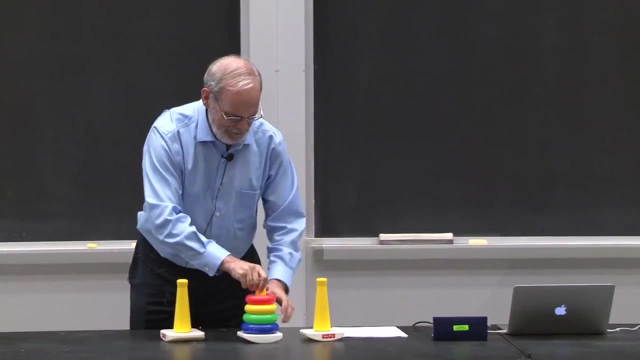 See how to solve it. Could you write code for this? Maybe not. That's on quiz. Thanks, John. don't tell them it's on the quiz, damn, All right. I'm going to claim, though, that in fact there's. 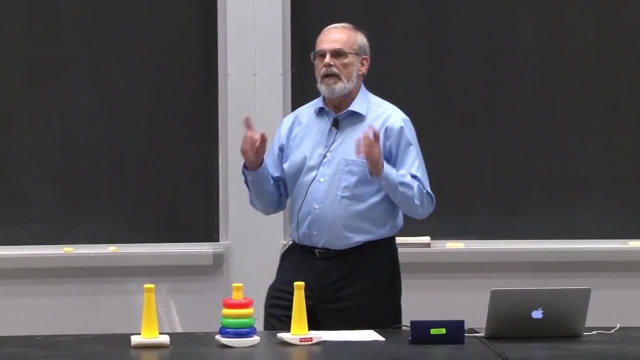 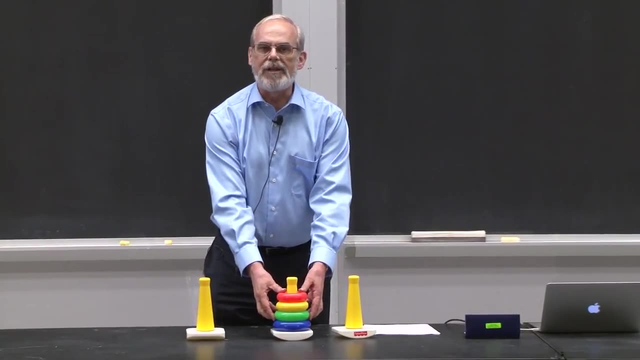 a beautiful recursive solution, And here's the way to think about it. recursively, I want to move a tower of size n. I'm going to assume I can move smaller towers, and then it's really easy. What do I do? I take a stack of size n minus 1,. 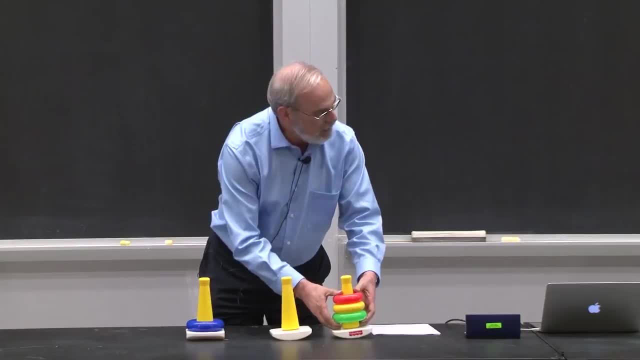 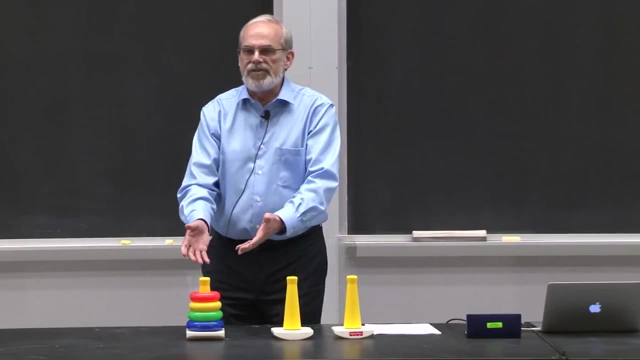 I move it onto the spare one, I move the bottom one over and then I move a stack of size n minus 1 to there. Beautiful Recursive solution. And how do I move the smaller stack? Just the same way I just. 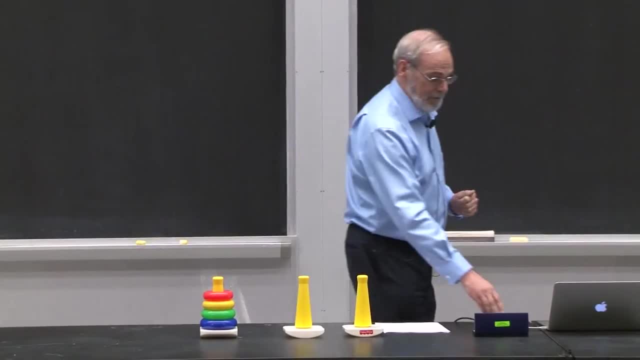 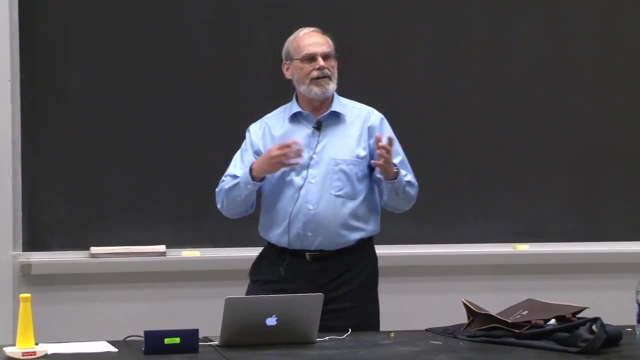 Unwind it Simple And in fact the code follows exactly that. OK, I do a little logit domain up here to try and get your attention. But notice, by doing that, what did I do? I asked you to think about it recursively. 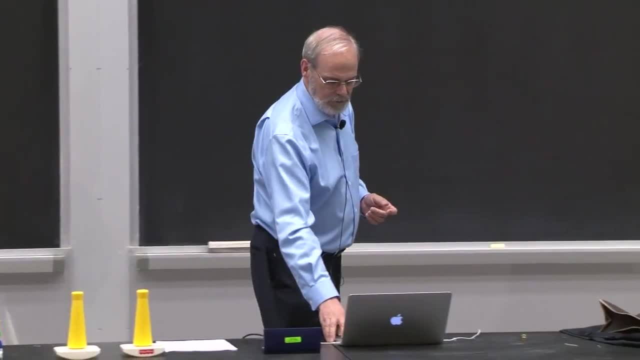 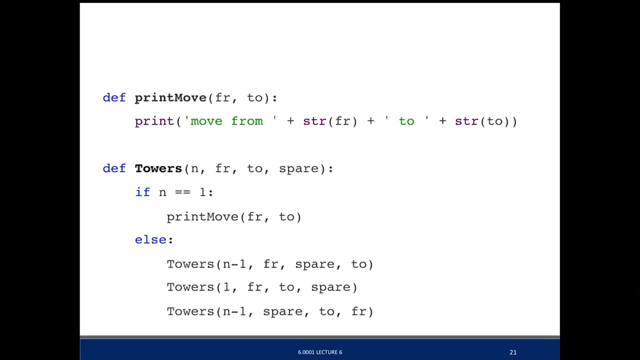 The recursive solution. when you see it is in fact very straightforward, And there's the code: Dead trivial. Well, dead trivial is unfair, But it's very simple, right? I simply write something, So let me describe it. 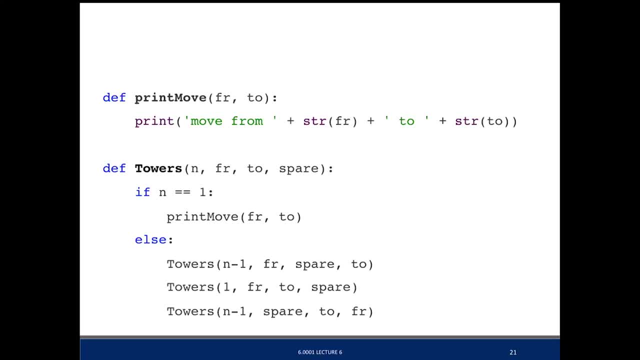 I need to say How big a tower am I moving, And I'm going to label the three stacks a from, a to and a spare. I have a little procedure that just prints out the move for me, And then what's the solution? 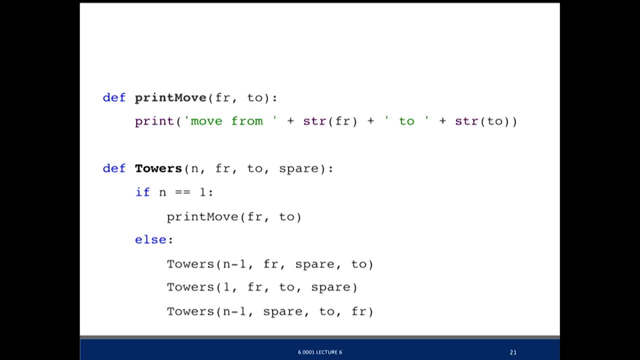 If it's just a stack of size 1, just print the move. Take it from from to 2.. Otherwise, move a tower of size n minus 1 from the from spot to the spare spot. Then move what's left- a tower of size 1, from from to 2.. 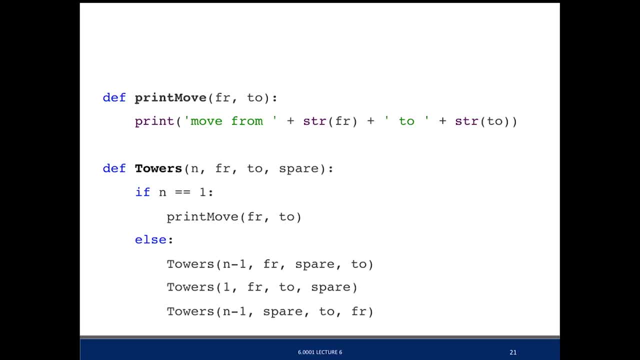 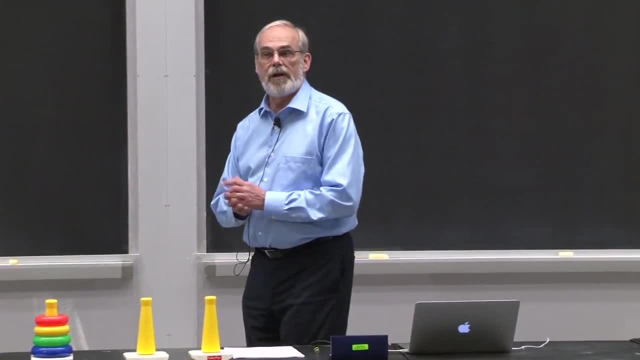 And then take that thing I stuck on spare And move it over to 2.. And I'm done In the code that we handed out. you'll see this code. You can run it. I'm not going to print it out. 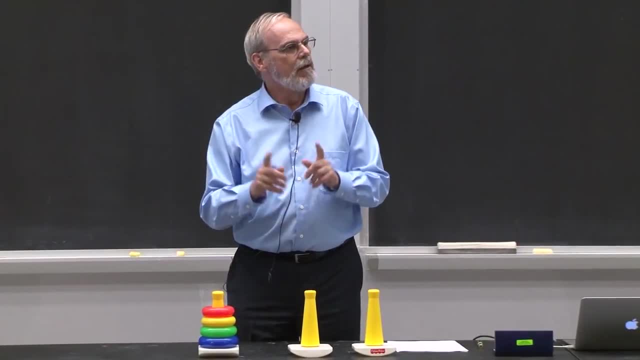 Because if I did use it, it's going to say, OK, it looks like it does the right kind of thing. Look at the code. Nice and easy, And that's what we'd like you to do when you're given a problem. 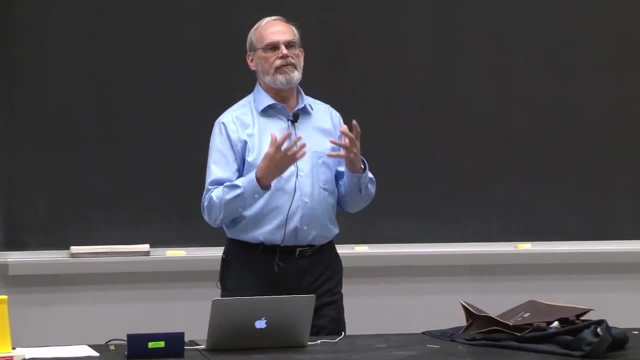 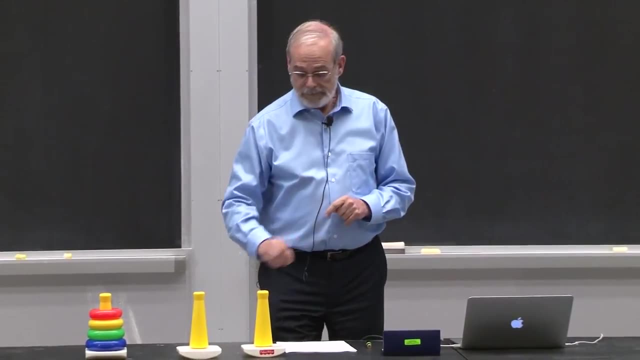 We ask you to think about it recursively. How do I solve this with a smaller version of the same problem, And then how do I use that to build the larger solution? This case is a little different. You could argue that this is not really a recursive call here. 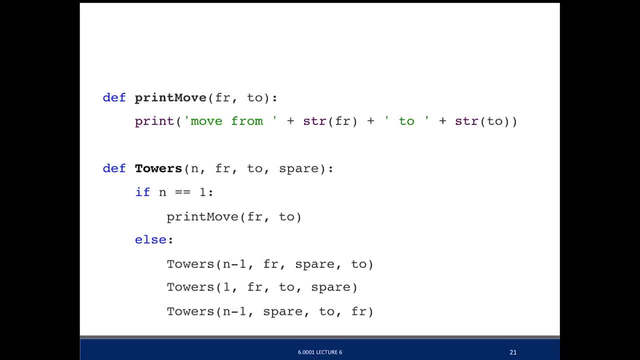 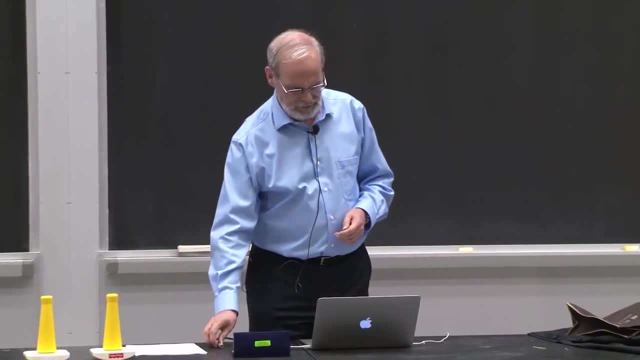 It's just moving the bottom one. I could have done that directly, But I've got two recursive calls in the body here I have to move a smaller stack twice. We're going to come back to that in a little bit. Let me show you one other example of recursion: that. 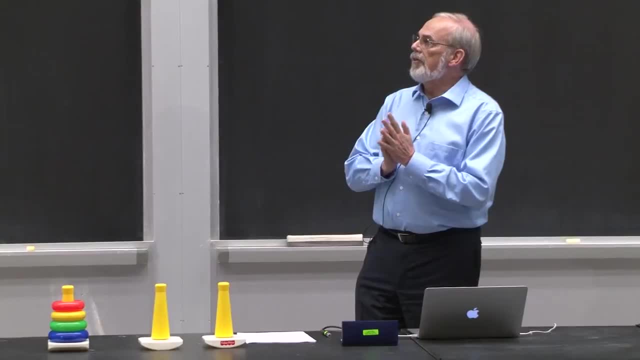 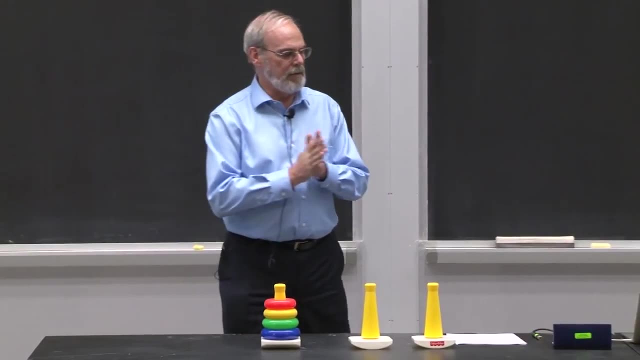 runs a little bit differently. In this case it's going to have multiple base cases, And this is another very old problem. It's called the Fibonacci numbers. It's based on something from several centuries ago, when a gentleman named Leonardo of Pisa, also known- 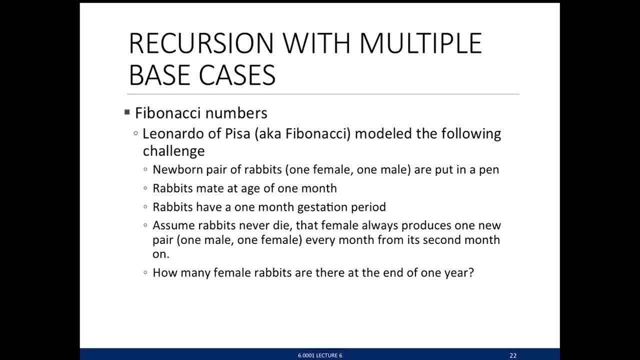 as Fibonacci asked the following challenge. He said: I'm going to put a newborn pair of rabbits, one male and one female, into an enclosure, a pen of some sort, And those rabbits have the following properties: They mate at age one month, so they take a month to mature. 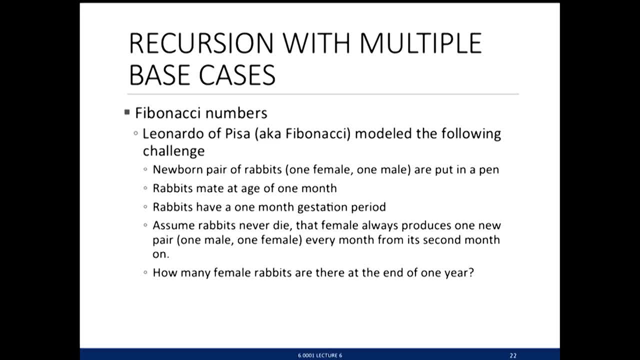 After a one-month gestation period they produce another pair of rabbits, a male and a female, And he says: I'm going to assume that the rabbits never die. So each month Mature females are going to produce another pair, And his question was: how many female rabbits? 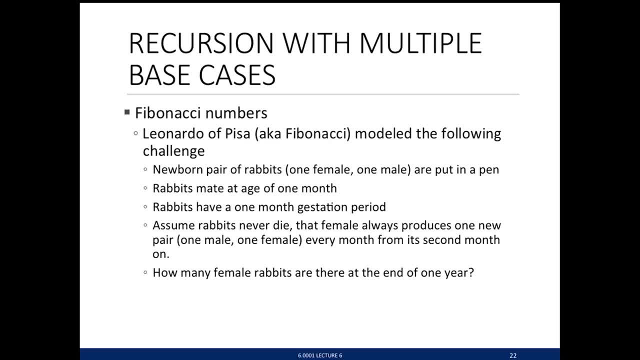 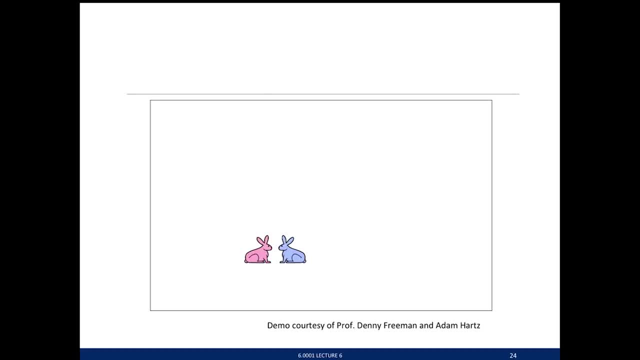 are there at the end of a year or two years or three years. So the idea is I start off with two immature rabbits. After one month they've matured, which means after another month they will have produced a new pair. 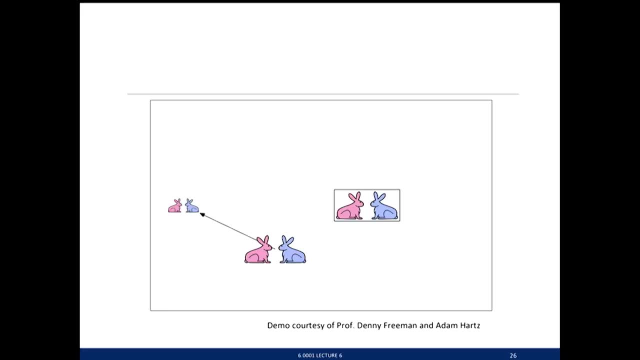 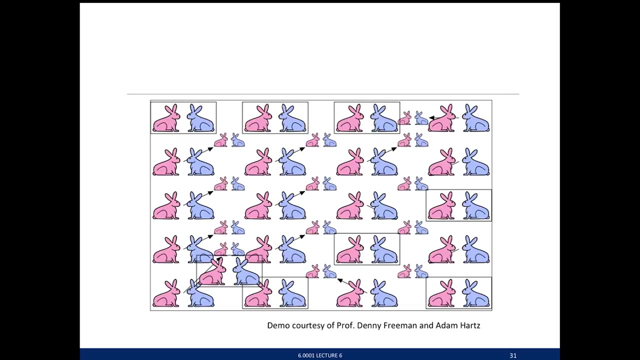 After another month that mature pair has produced another pair And the immature pair has matured. which means after another month those two mature pairs are going to produce offspring And that immature pair has matured. And you get the idea. And after several months you get to Australia. 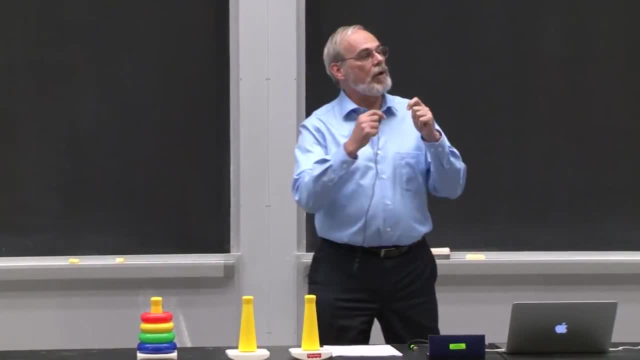 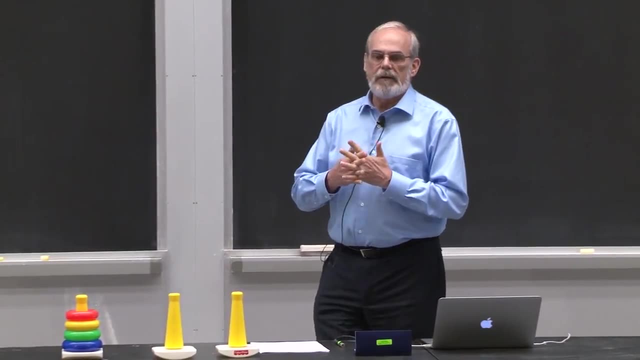 You can also see this is going to be interesting to think about. how do you compute this? But what I want you to see is the recursive solution to it. So how could we capture this? Well, here's another way of thinking about it. 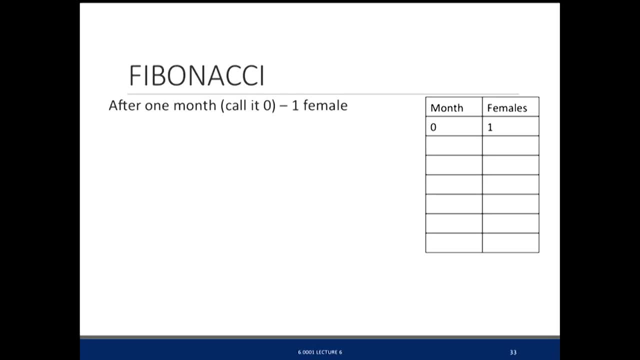 After the first month- and I know we're going to do this funny thing: we're going to index at zero, So call it month zero- There is one female which is immature After the second month. that female is mature and now pregnant, which? 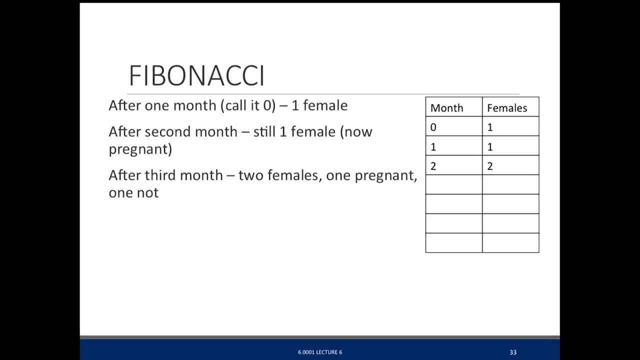 means after the third month it has produced an offspring And, more generally, at the nth month after we get past the first few cases. what do we have? Any female that was there two months ago has produced an offspring because it's. 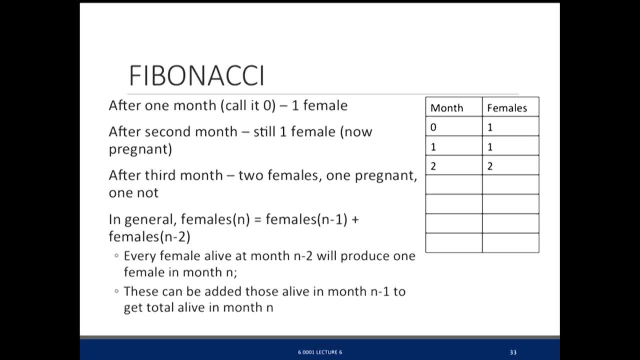 taken at least one month to mature, if it hasn't already been mature, and then it's going to produce an offspring, And any female that was around last month is still around, because they never die off. So this is a little different. 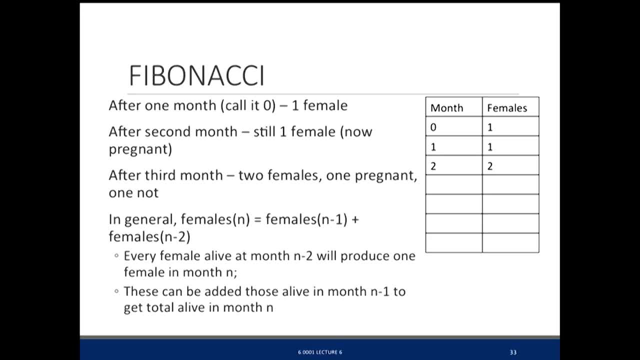 This is now the number of females at month n is the number of females at month n minus 1 plus the number of females at month n minus 2.. So two recursive calls, but with different arguments, Different from powers of Hanoi, where 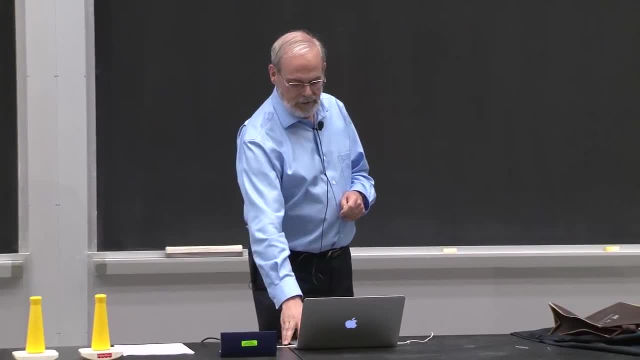 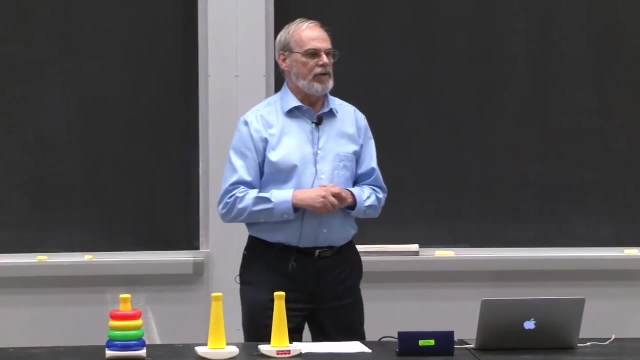 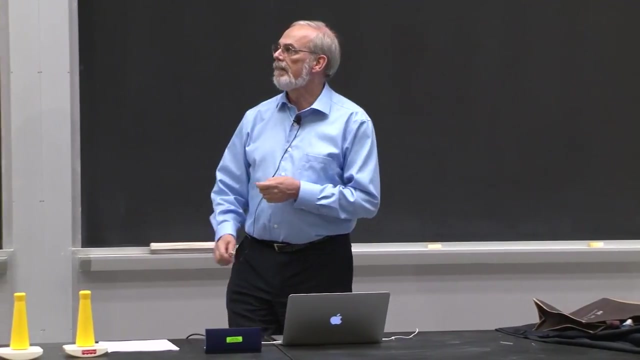 there were two recursive calls, but with the same size problem. So now I need two base cases: one for when n is equal to 0,, one for when n is equal to 1.. And then I've got that recursive case, And so there's a nice little piece of code. 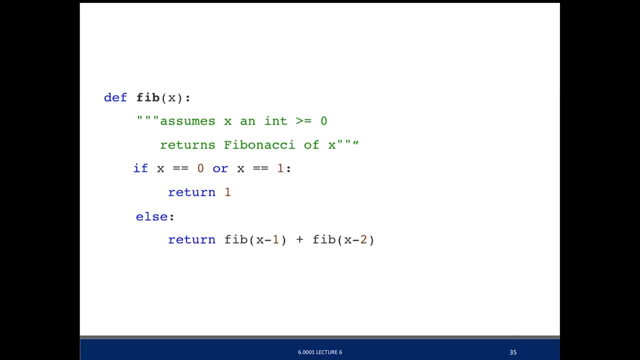 Fibonacci. I'm going to assume x is an integer greater than or equal to 0.. I'm going to return fibonacci of x And you can see now it says: if either x is equal to 0 or x is equal to 1, I'm going to return 1.. 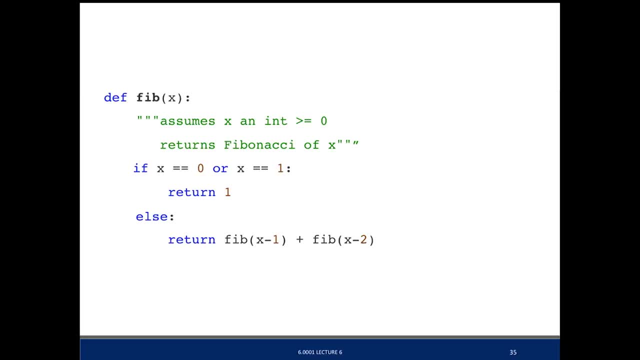 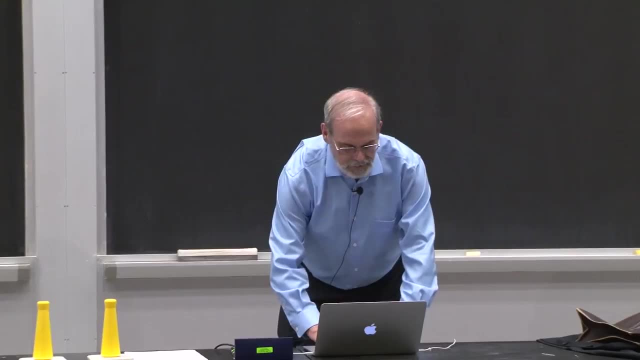 Otherwise I reduce it to 2.5.. Simpler versions of the problem, but with different arguments, And I add them up. OK, And if we go look at this, we can actually run this. I can find my code, which is right there. 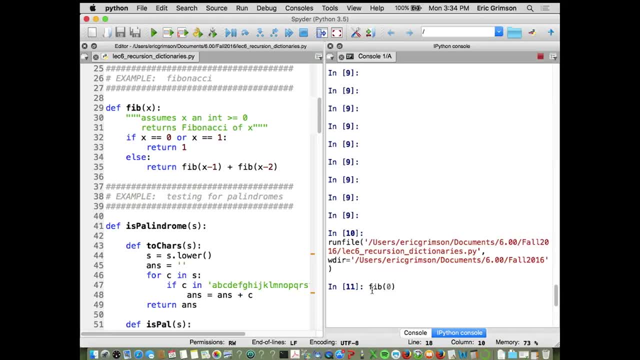 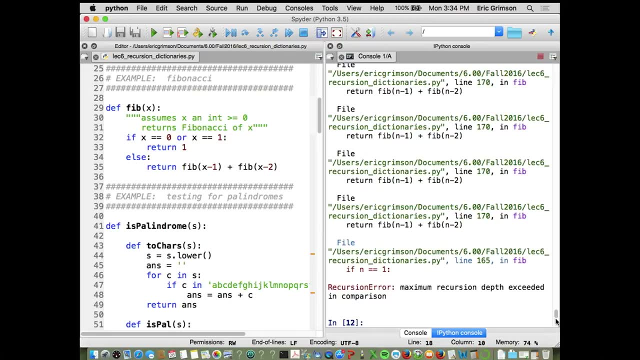 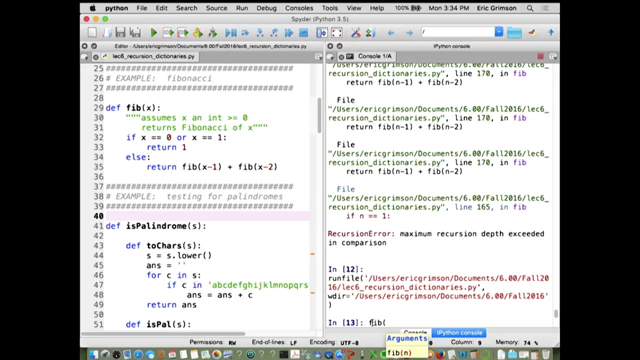 So we can, for example, check it by saying fib of 0. And I just hit a bug which I don't see. Let me try it again. I'll try it one more time with fib of 0.. Darn. 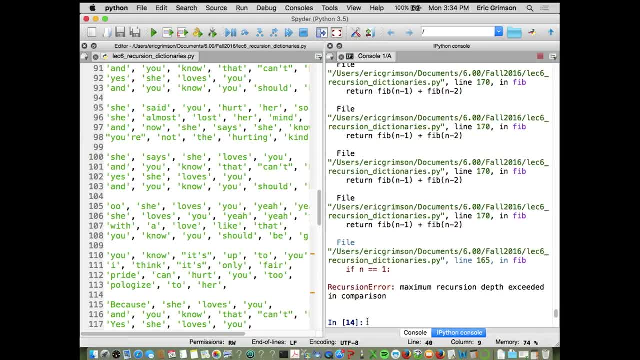 I'm going to let me try it again. Just one more time. Let me try it again. I've got two different versions of fib in here. That's what I've got going on, So let me do it again. Let's do fib of 1.. 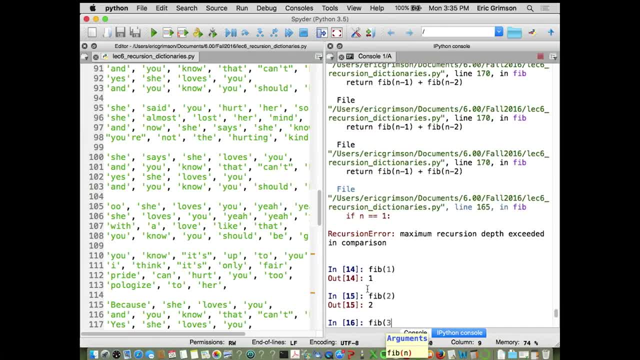 There we go. Fib of 2,, which is 2.. Fib of 3,, which is 3.. And fib of 4,, which should add the previous two, which gives me 5.. There we go. Sorry about that. 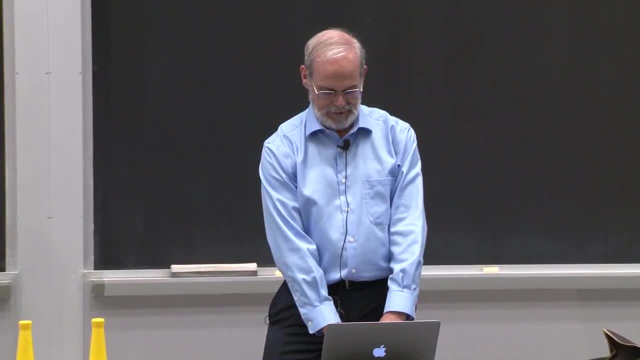 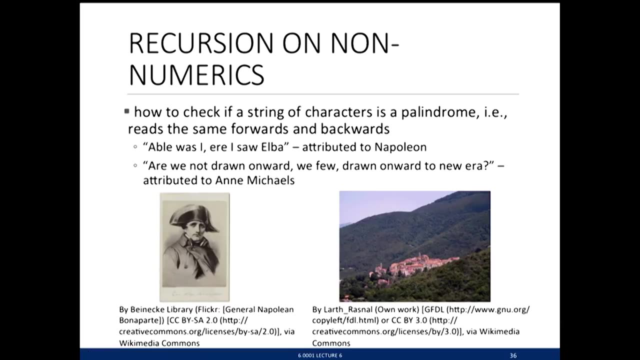 I have two versions of fib in my file, which is why it complained at me and which is why you should always read the error instructions, because it tells you what you did wrong. Let's go on and look at one more example of doing recursion. 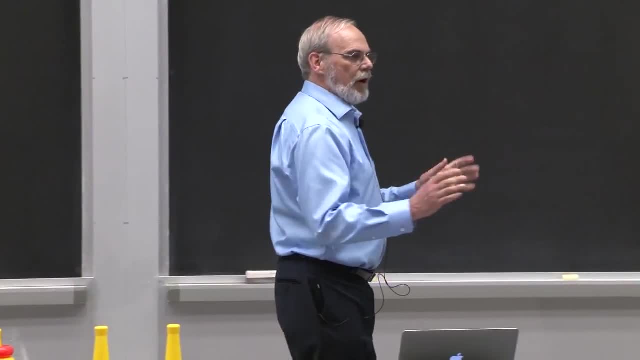 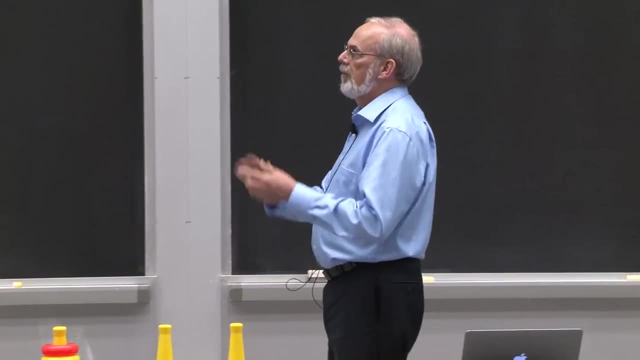 Then we're going to do dictionaries and then we're going to pull it all together. So far we've been doing recursion on numerical things. We can do it on non-numerical things. So a nice way of thinking about this is: how would I tell if a string of characters is a palindrome? 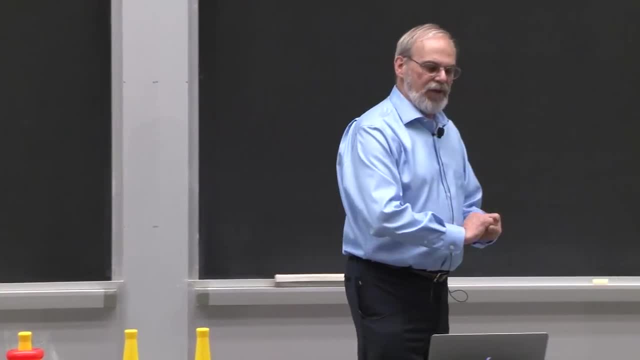 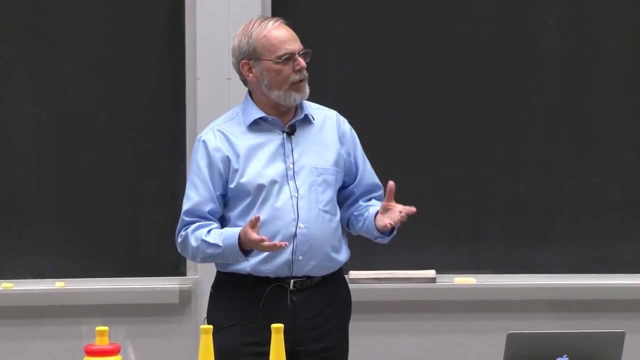 Meaning. it reads the same backwards and forwards. Probably the most famous palindrome is attributed to Napoleon Able was I ere I saw Elba. Given that Napoleon was French, I really doubt he said able was I ere I saw Elba, But it's a great palindrome. 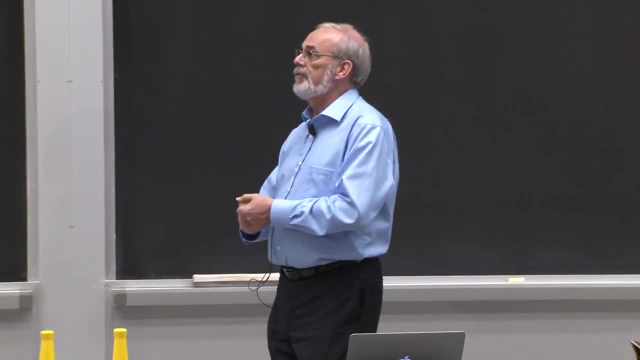 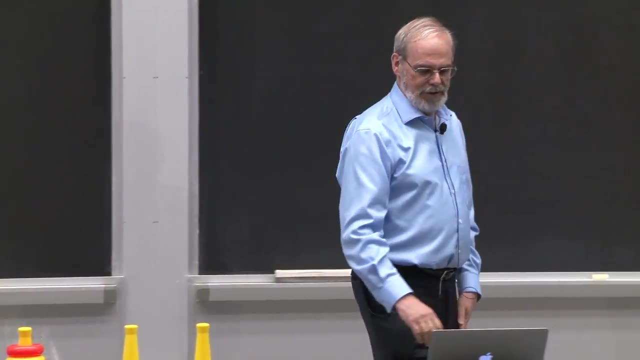 Another one attributed to Anne Michaels: Are we not drawn onward? we few drawn onward to a new era Reads the same backwards and forwards. It's fun to think about. how do you create the palindromes? I want to write code to solve this. 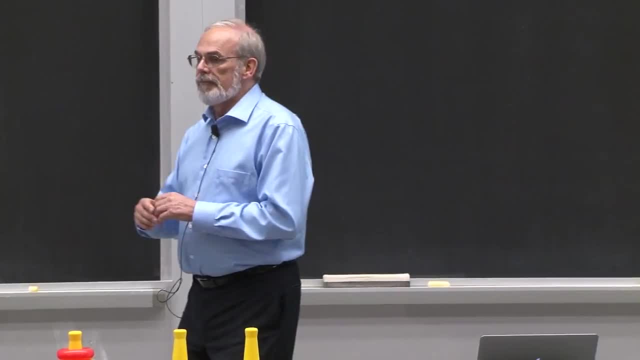 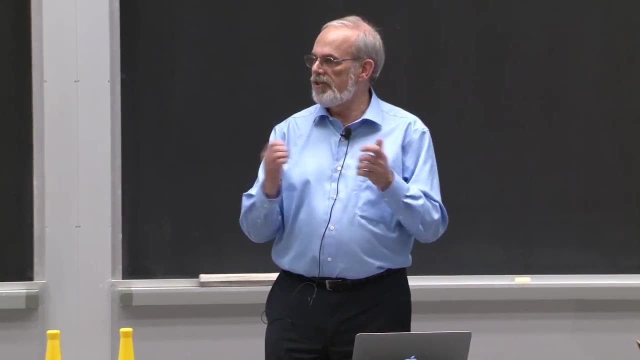 Again, I want to think about it recursively. So here's what I'm going to do. I'm first going to take a string of characters, reduce them all to lowercase and strip out spaces and punctuation. I just want the characters. And once I got that, I want to say: 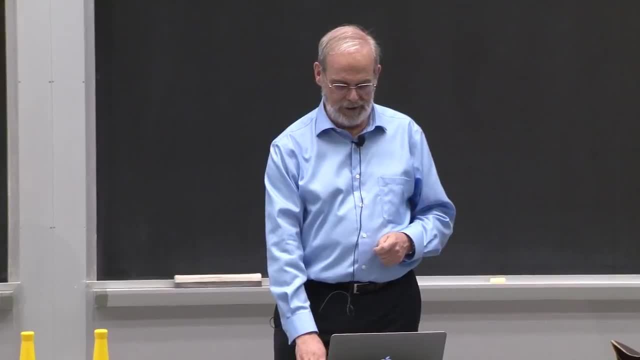 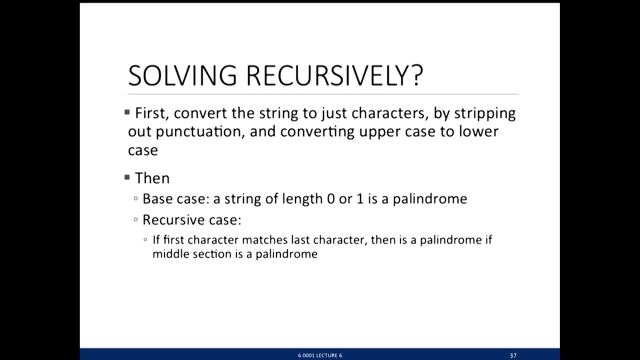 is that string, that list of characters or that collection of characters? I should say a palindrome And I'm going to think about it recursively And that's actually pretty easy. If it's either 0 or 1 long, it's a palindrome. 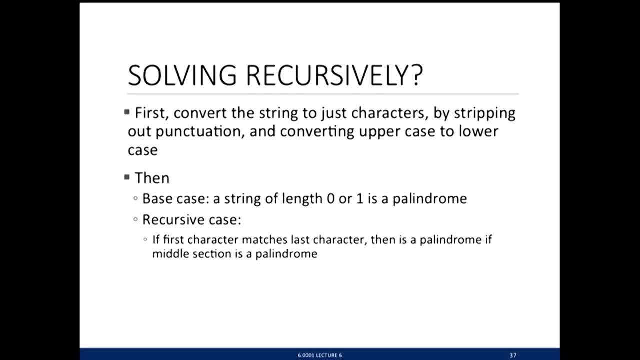 Otherwise you could think about having an index at each end of this thing and sort of counting into the middle. But it's much easier to say: take the two at the end. If they're the same, then check to see. what's left in the middle is a palindrome. 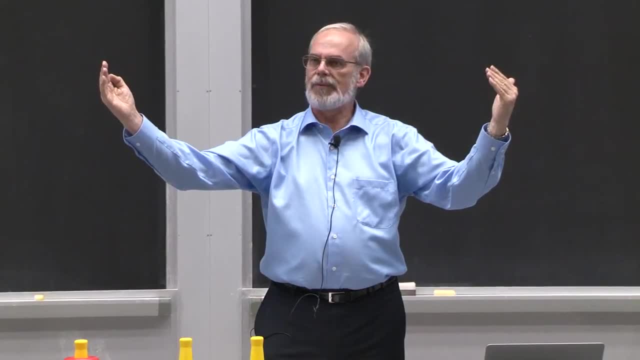 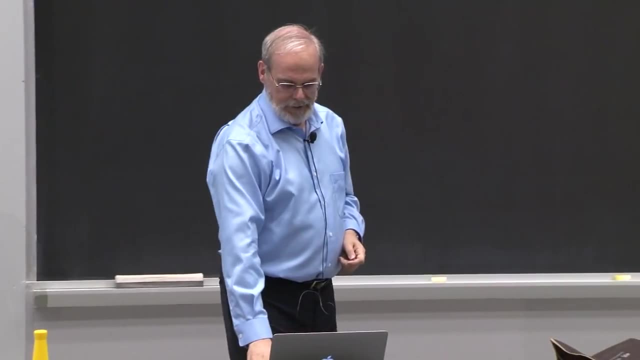 And if those two properties are true, I'm done. And notice what I just did. I nicely reduced a bigger problem to a slightly smaller problem. It's exactly what I want to do, OK, So what it says to check is this: 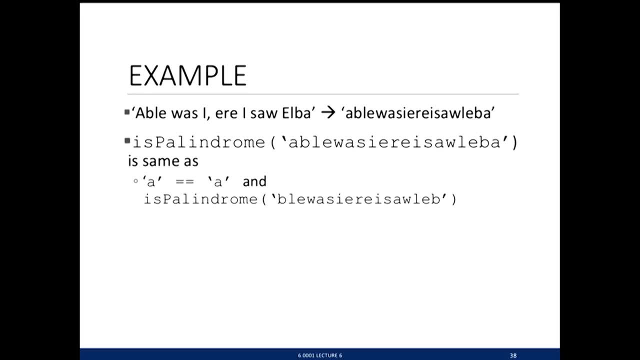 I'm going to reduce it to just the string of characters And then I'm going to check that's a palindrome by pulling those two off and checking to see they're the same, and then checking to see if the middle is itself a palindrome. 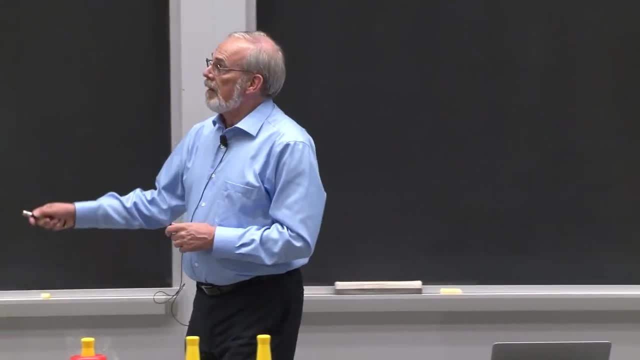 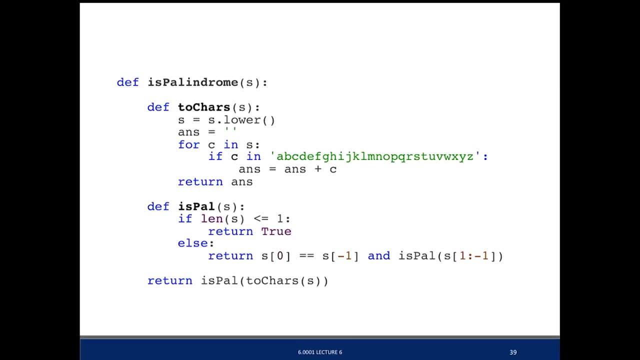 OK, How would I write it? I'm going to create it. The procedure up here is palindrome. I'm going to have inside of it two internal procedures that do the work for me. The first one is simply going to reduce this to all lowercase. 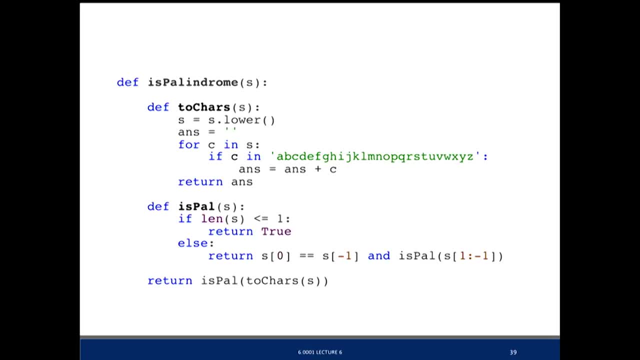 with no spaces And notice what I can do. Because s is a string of characters, I can use the built-in string method lower. So there's that dot notation slower. It says: apply the method lower to a string. I need an open and close paren to actually call. 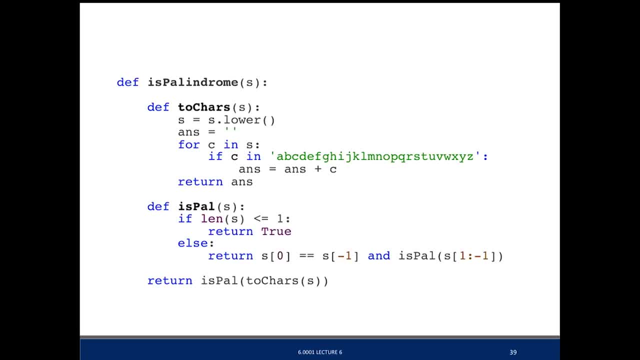 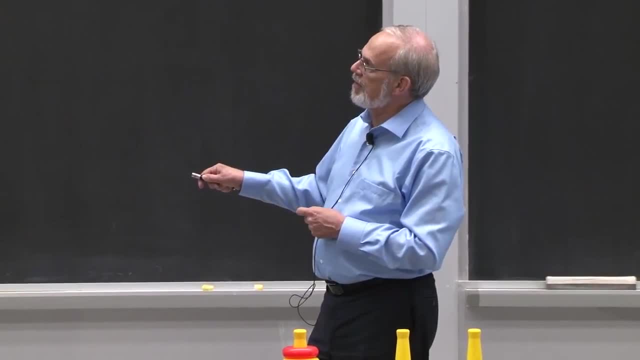 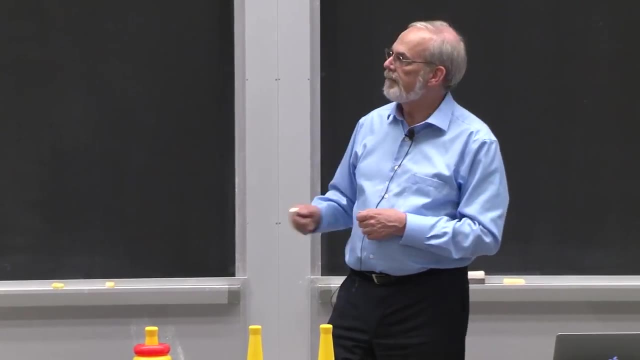 that procedure And that will mutate s to just be all lowercase. And then I'm going to run a little loop. I'll set up answer or ans to be an empty string And then for everything inside that mutated string I'll simply say if it's inside this string, if it's a letter, 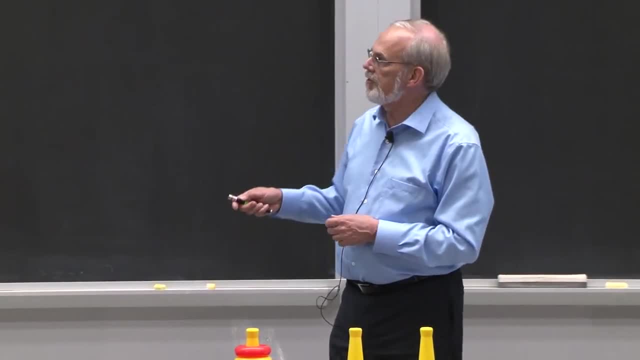 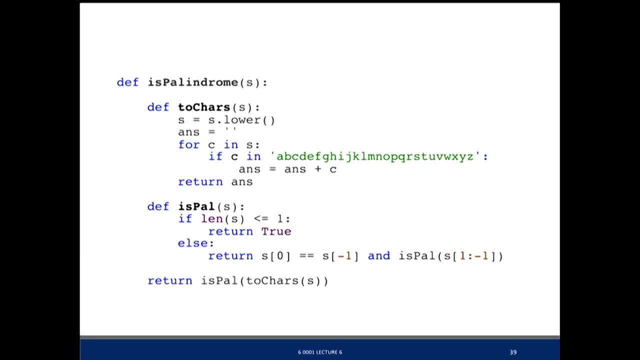 add it into answer. If it's a space or a comma or something else, I'll ignore it And when I'm done, just return answer Strips it down to lowercase And then I'm going to pass that into isPal, which simply says: 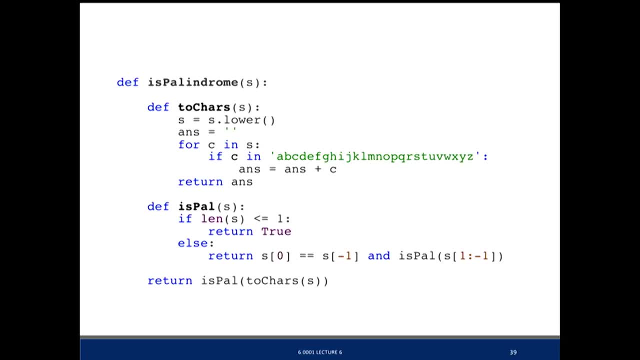 if this is either 0 or 1 long, it's a palindrome Return. true. Otherwise, check to see that the first and last element of the string are the same. Notice the indexing to get into the last element And similarly just slice into the string. 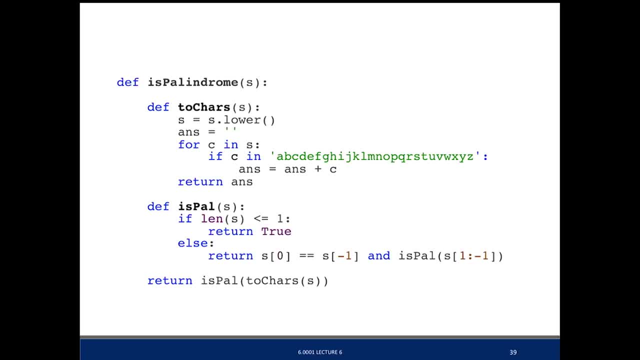 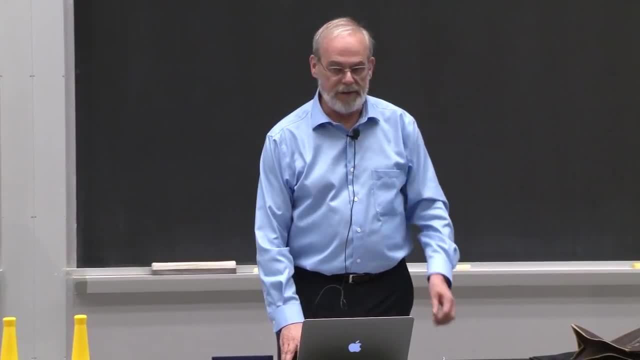 ignoring the first and last element, and ask: is that a palindrome? And then just call it And that'll do it. And again, there's a nice example of that in the code. I'm not going to run it, I'll let you just go look at it. 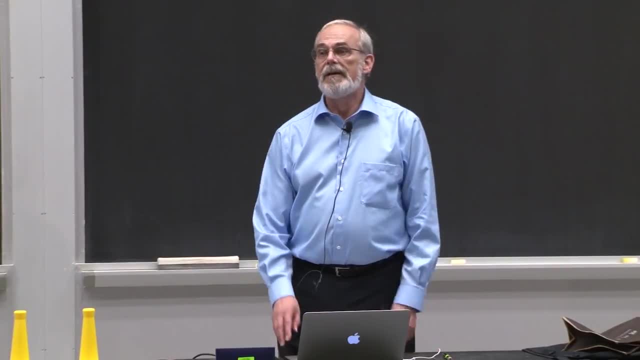 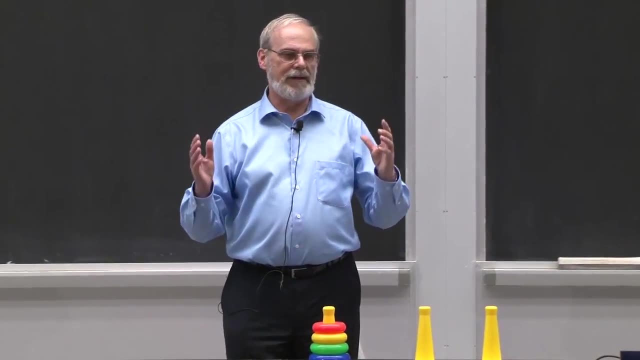 But it will actually pull out something that checks: Is this a palindrome? Notice again what I'm doing here. I'm doing divide and conquer. I'm taking a problem, reducing it. I keep saying this to a simpler version of the same problem. 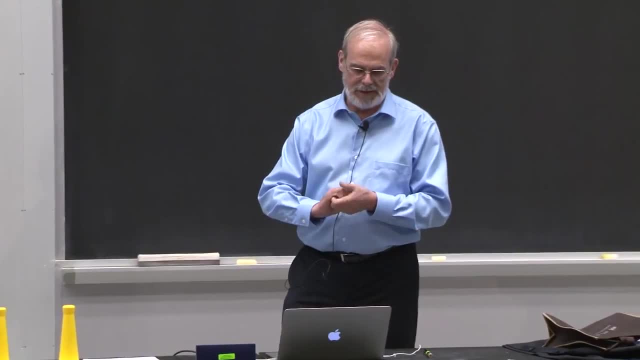 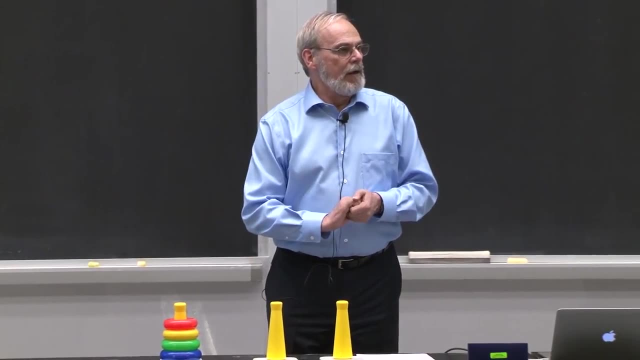 Keep unwinding it till I get down to something I can solve directly in my base case and I'm done. And that's really the heart of thinking about recursive solutions to problems. I would hope that one of the things you remember, besides my really lousy patter up here. 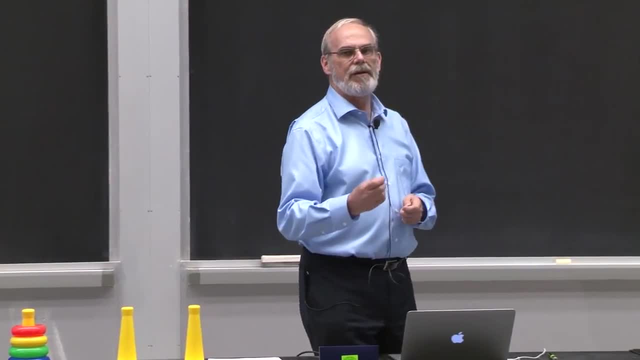 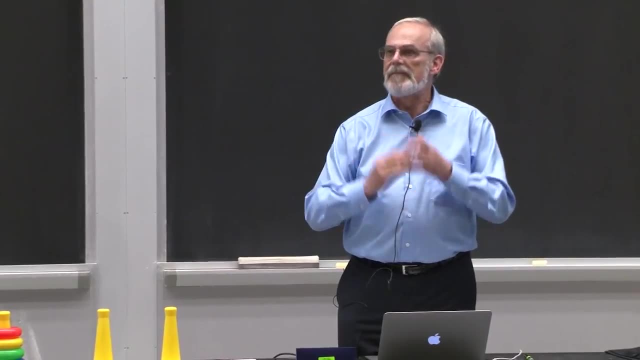 is the idea of towers, And I think that's a really good example of that in Hanoi, because to me it's one of the nicest examples of a problem that would be hard to solve iteratively, But when you see the recursive solution, 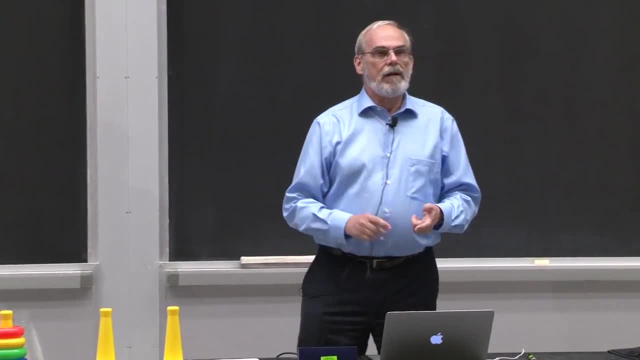 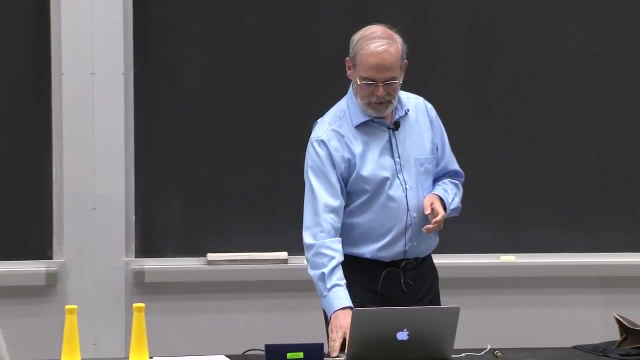 it's pretty straightforward. Keep that in mind as you think about doing recursion. OK, Let's switch gears and let's talk very briefly about another kind of data type called a dictionary, And the idea of a dictionary I'm going to motivate with a simple example. 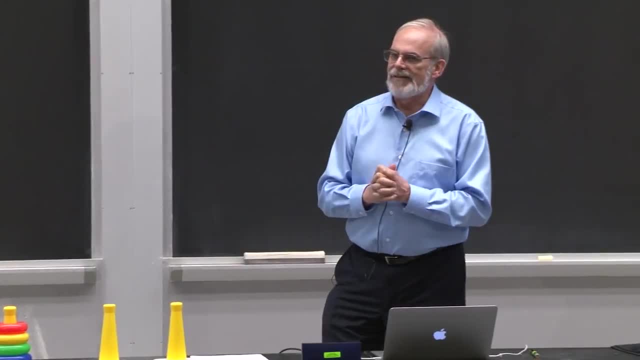 There's a quiz coming up on Thursday- I know you don't want to hear that, but there is- which means there's a list of grades, And so imagine I wanted to build a little database just to keep track of grades of students. 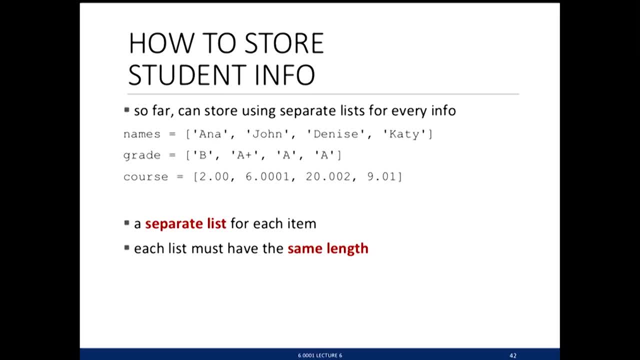 So one of the ways I could do it is I could create a list with the names of the students. I could create another list with their grades and a third list with the actual subject or course from which they got that grade. Keep a separate list for each one of them. 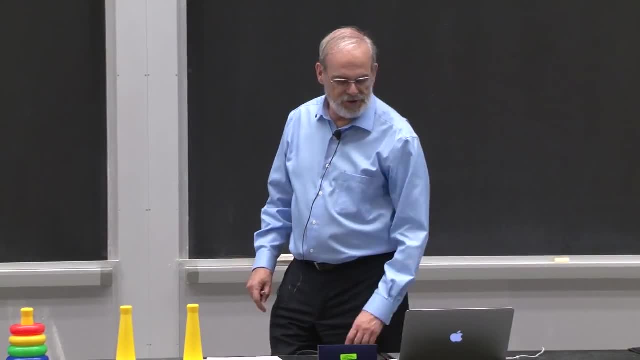 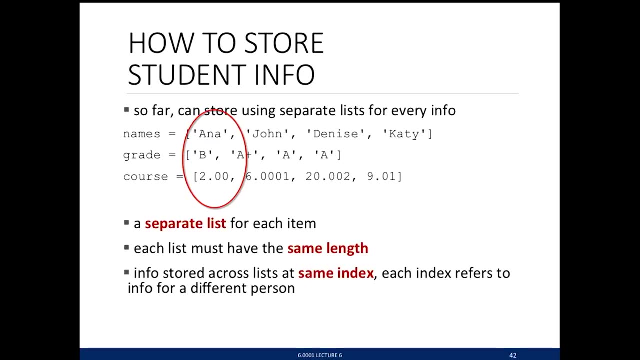 Keep them of the same length And in essence, what I'm doing here is I'm storing information at the same index in each list. So Anna, who's going to have to take the class again, gets a B. John, who's created the class, gets an A plus. 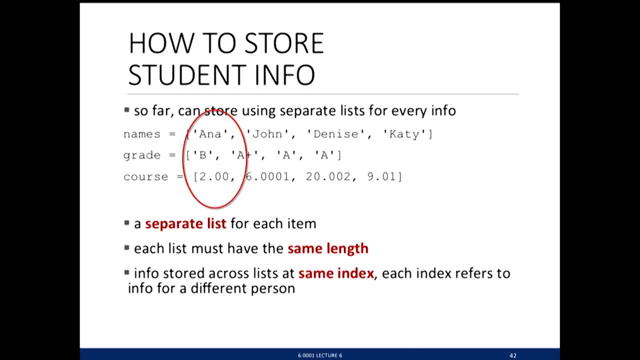 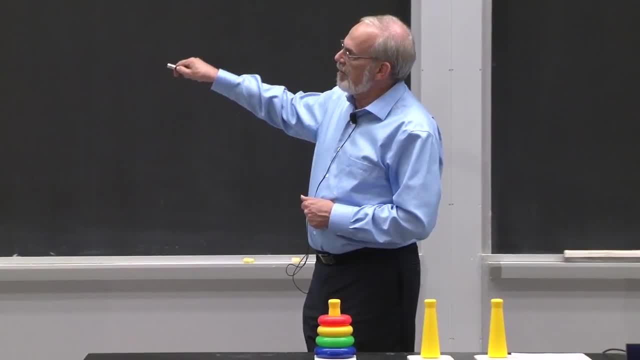 Sorry, Anna John's had a longer time at it. All right, Bad jokes aside, what I'm doing is, I could imagine, just creating lists. I could create lists of lists, but a simple way is to do lists where basically at each index. 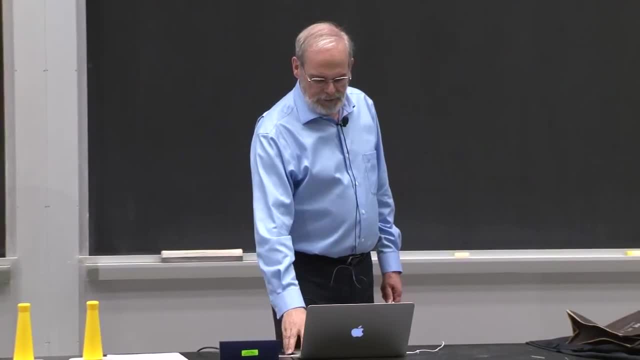 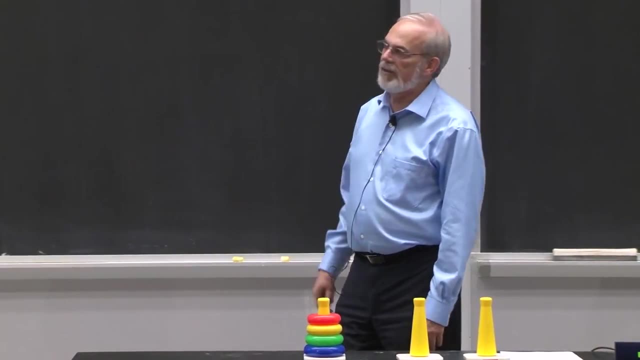 I've got associated information. It's a simple way to deal with it. Getting a grade out takes a little bit of work because if I want to get the grade associated with a particular student, what would I do? What would I do? 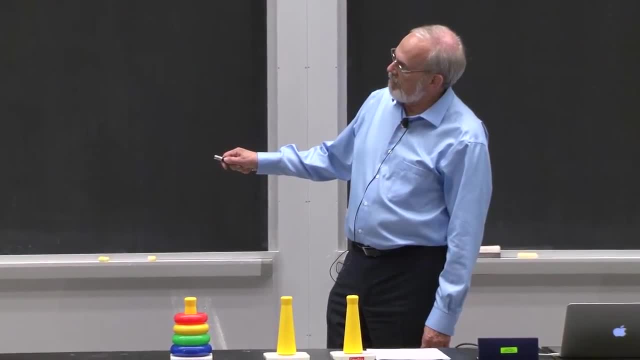 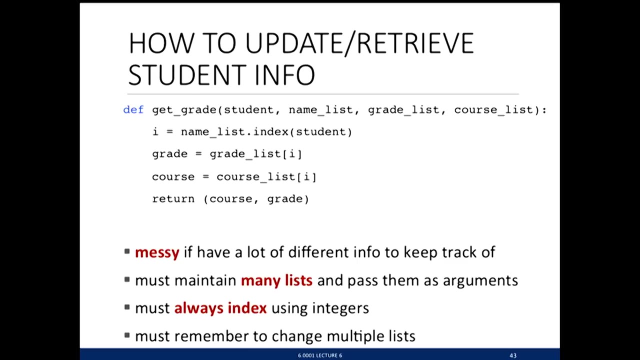 I would go into the name list and use the method index, which you've seen before. Again, notice the dot notation. It says this is a list. Use the index method, Call it on student And whatever the value of student is. 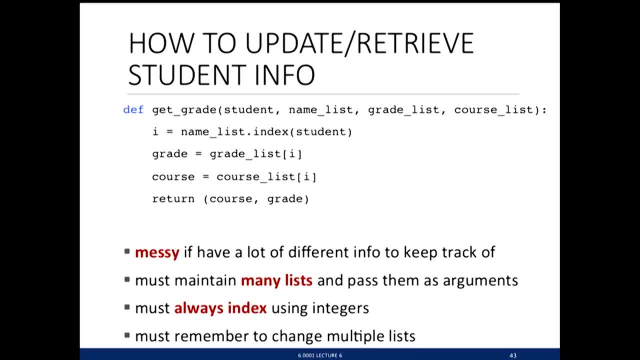 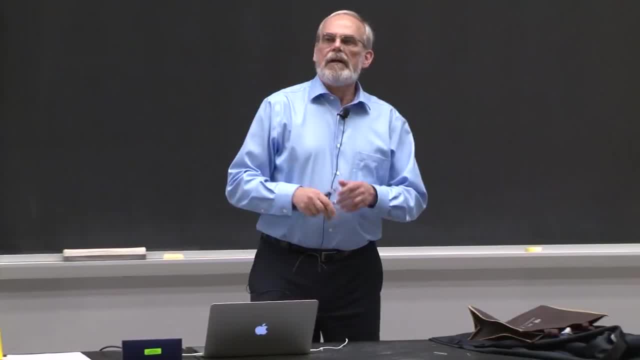 it will find that in the list. return the index at that point And then I can use that to go in and get the grade in the course and return something out. Simple way to do it, but a little ugly because, among other things, I've got things stored. 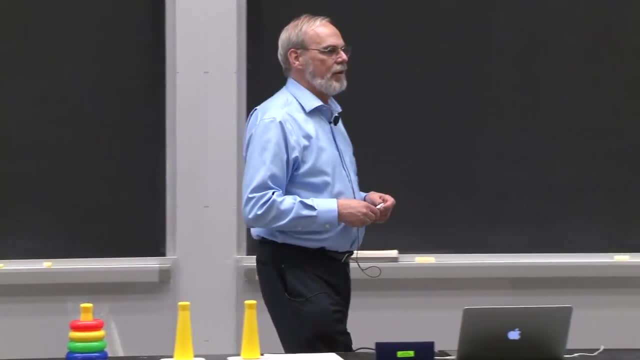 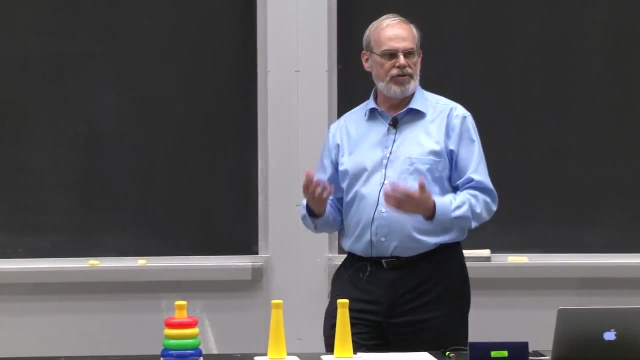 in different places in the list. I've got to think about if I'm going to add something to the list. I've got to put them in the same spot in the list. I've got to remember to always index using integers, which is what we know how to do with lists, at least so far. 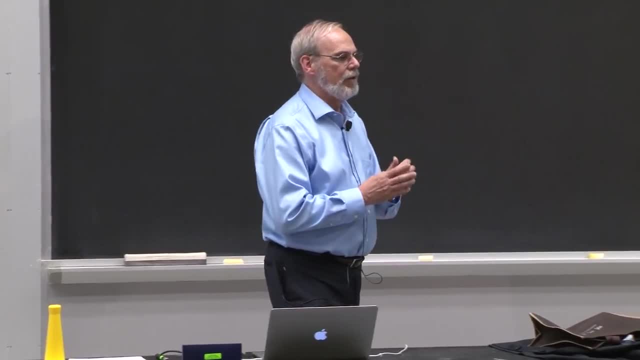 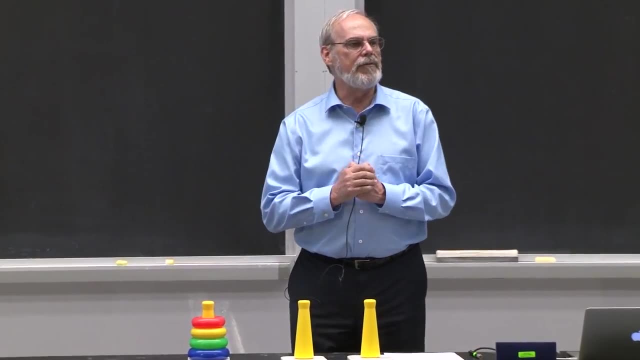 It would be nice if I had a better way to do it, And that's exactly what a dictionary is going to provide for me. So, rather than indexing on integers, I'd like to index directly on the item of interest. I'd like to say: where's Anna's record? 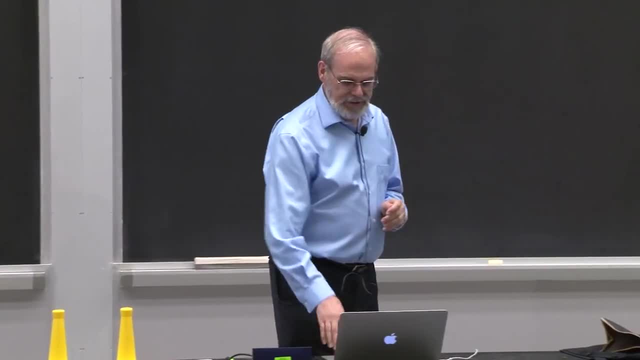 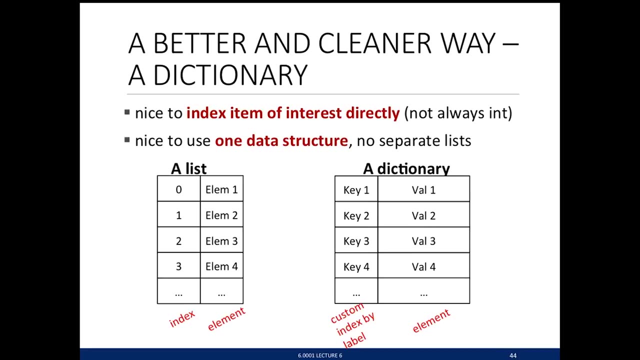 And find that in one data structure. And so, whereas a list is indexed by integers and has elements associated with it, a dictionary is going to combine a key or, if you like, a name of some sort with an actual value, And we're going to index just by the name or the label. 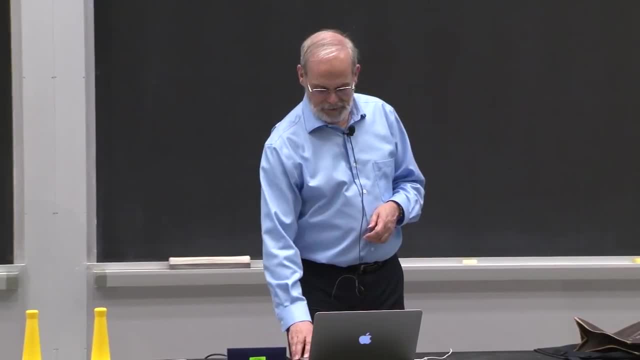 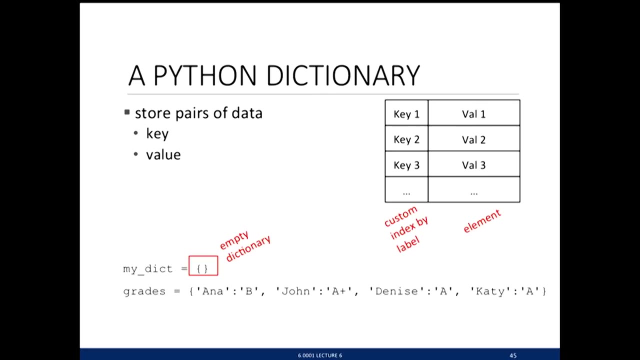 as we go into it. So let me show you some examples. First of all, to create a dictionary, I use curly braces- open-close curly brace. So an empty dictionary would be simply that call If I want to create an actual dictionary. 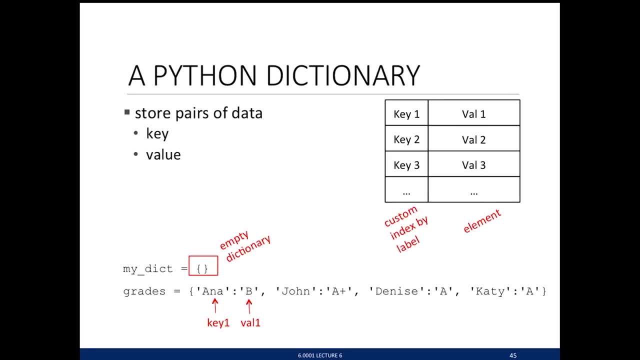 before I insert things into it, I use a little bit of a funky notation. It is a key or a label, a colon and then a value, In this case the string Anna and the string B, followed by a comma which separates it. 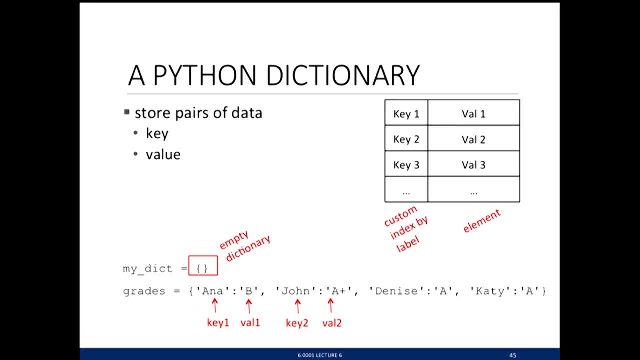 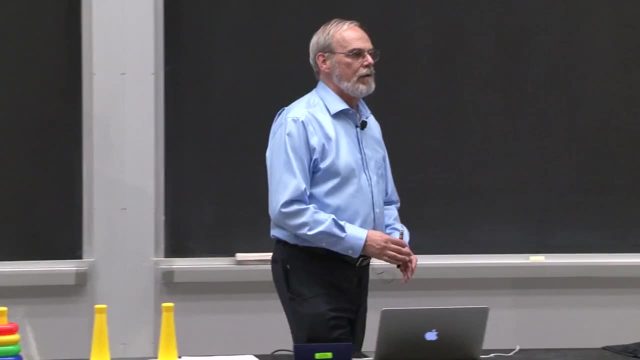 from the next pairing of a key and a label or a key and a value, and so on. And so if I do this, what it does in my dictionary is it creates pairings of those labels And I can do that with the values I associated with them. 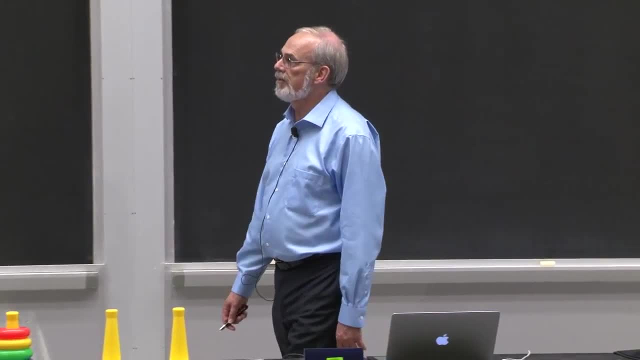 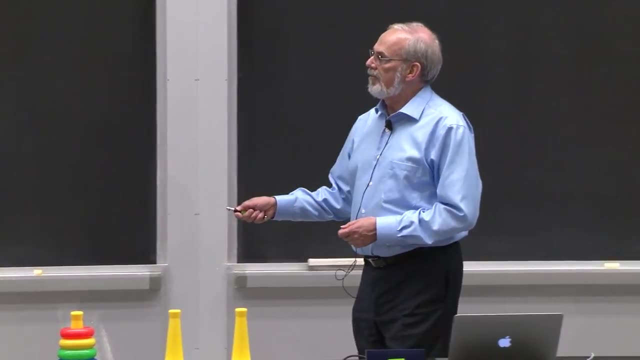 OK, these are pretty simple, But in fact there's lots of nice things we can do with it. So, once we've got them, indexing now is similar to a list, but not done by a number. It's done by a value. 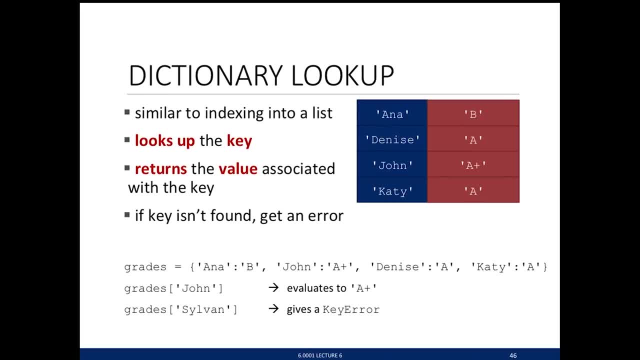 So if that's my key, I can say what's John's grade. Notice the call It's grades, which is my dictionary. Open-close square brackets with the label John And what it does. it goes in and finds that in the dictionary. 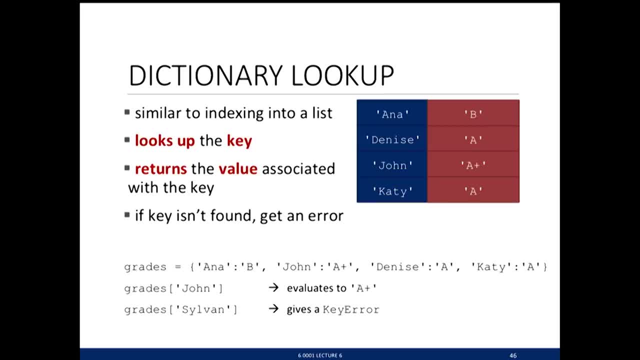 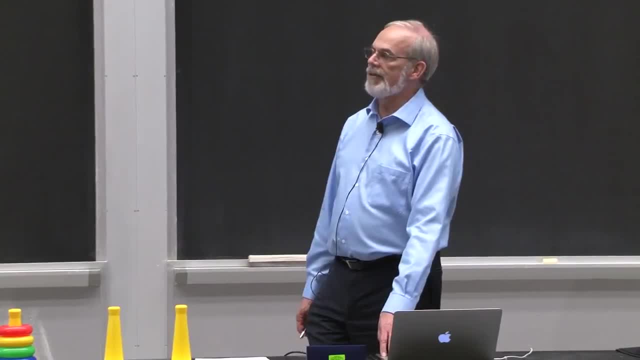 what's associated with it. If I ask for something not in the dictionary, it's going to give me a key error. Other things we can do with dictionaries: We can add entries, just like we would do with lists. Grades is a dictionary. 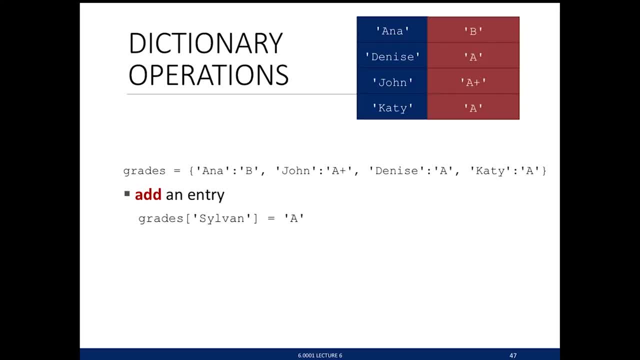 And in open and close square brackets I put in a new label and a value And that adds that to the dictionary. I can test if something's in the dictionary by simply saying, is this label in grades, And it simply checks all of the labels or the keys. 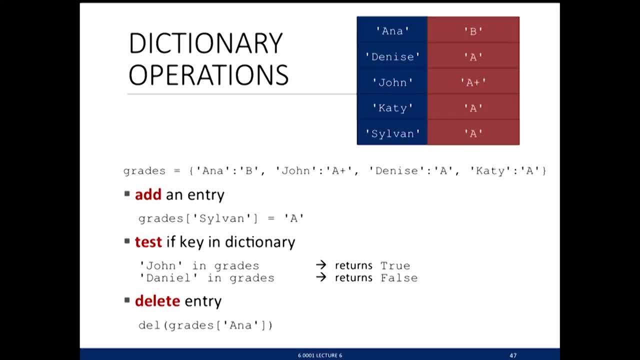 for the dictionary to see if it's there And if it's not, returns false. I can remove entries. Del something. we've seen before. a very generic thing: It will delete something And in this case it says in the dictionary: grades. 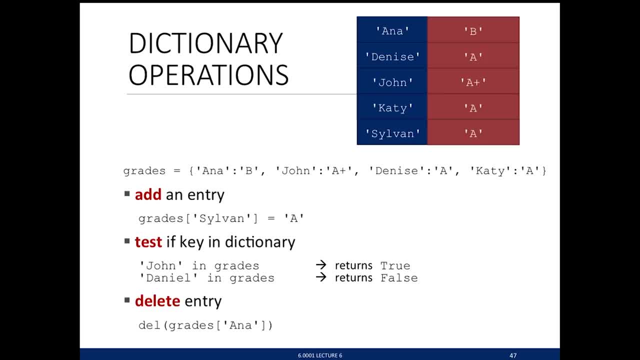 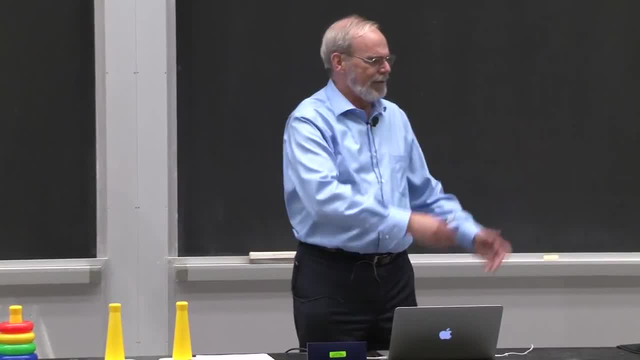 find the entry associated with that key. Sorry, Anna, you're about to be flushed. Remove it. She's only getting a B in the class and she teaches it. We've got to do something about this, right? OK, so I can add things. 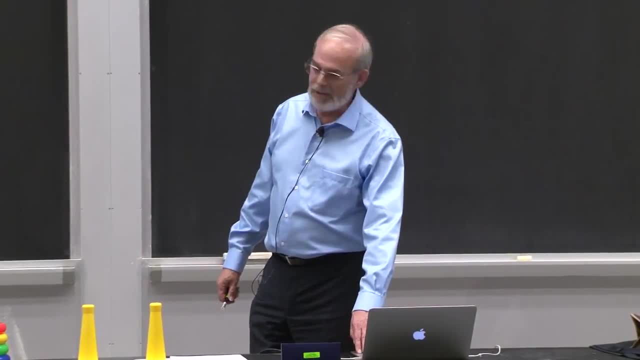 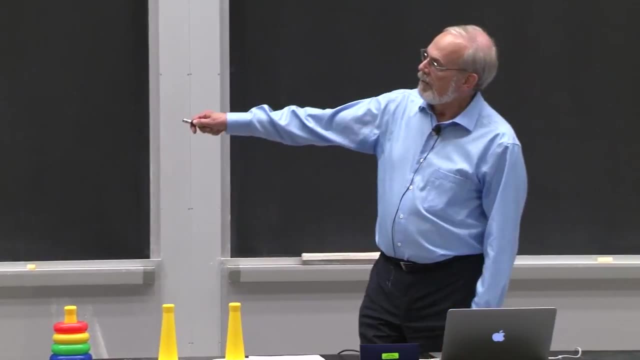 I can delete things. I can test if things are there. Let me show you a couple of other things about dictionaries. I can ask for all of the keys in the dictionary. Notice the format There's: that dot notation Grades is a dictionary. 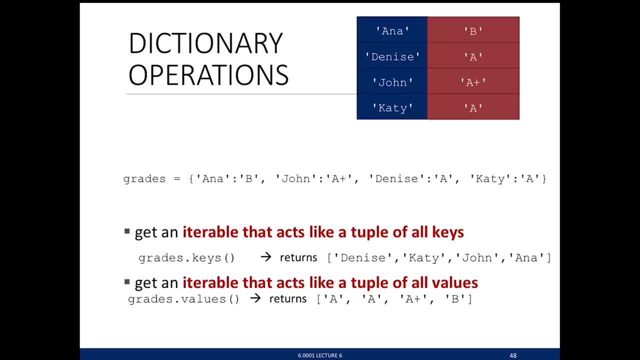 It says: use the keys method associated with this data structure dictionaries. Open, close actually calls it, And it gives me back a collection of all the keys In sum. Arbitrary order- I'm going to use a funny term here which I'm not. 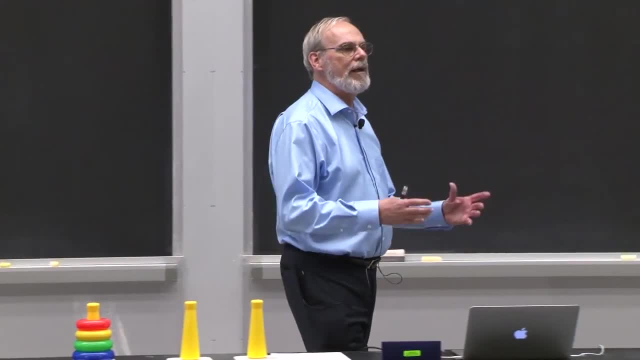 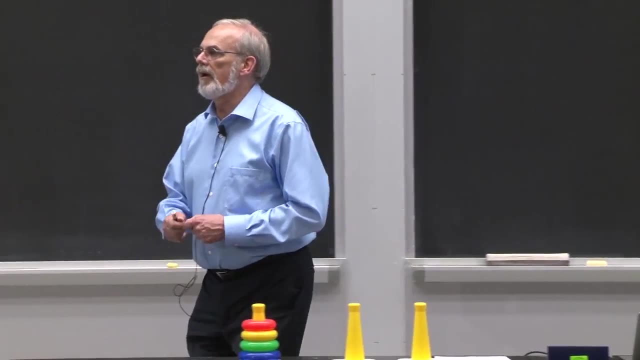 certain we've seen so far. It returns something we call an iterable. It's like range. Think of it as giving us back the equivalent of a list. It's not actually a list, but it's something we can walk down, which is exactly why I can then. 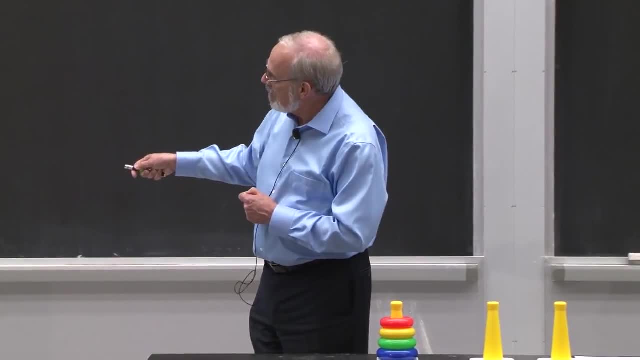 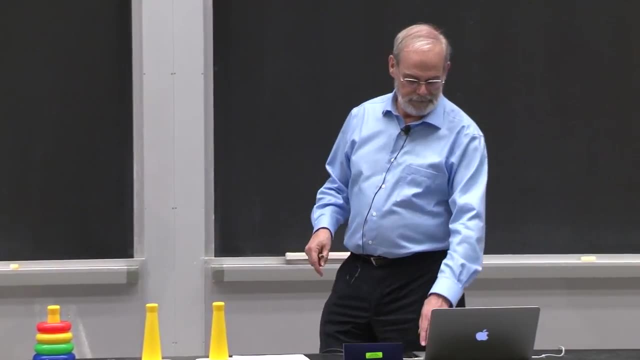 say, is something in a dictionary, Because it returns this set of keys and I can test to see if something's in there. I can similarly get all of the values if I wanted to look at them, giving us out two iterables. 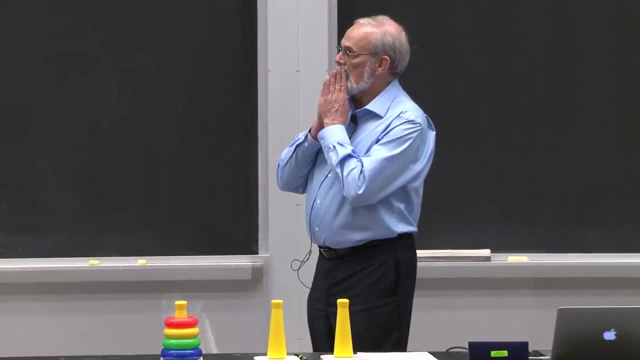 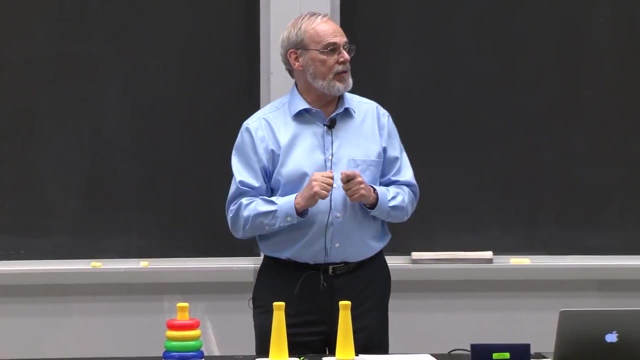 Here are the key things to keep in mind about dictionaries. The values can be anything, any type, mutable, immutable- They could be duplicates. That actually makes sense. I could have the same value associated, for example, the same grade associated, with different people. 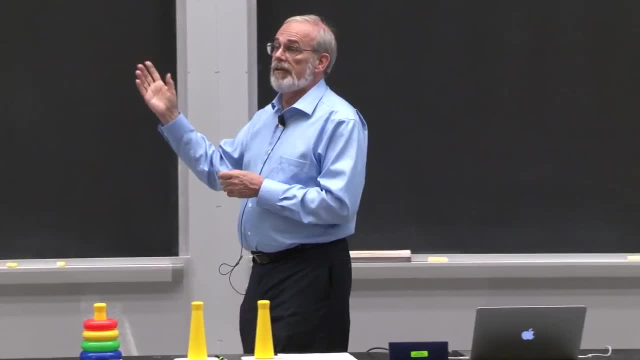 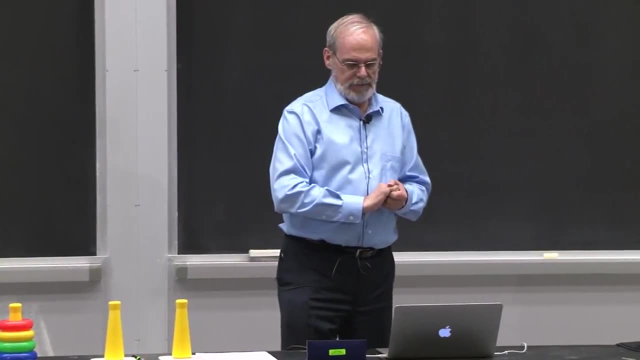 That's perfectly fine. The values could be lists, They could be other data structures, They could even be other dictionaries. They can be anything which is great. The keys, the first part of it: a little more structure. They need to be unique. 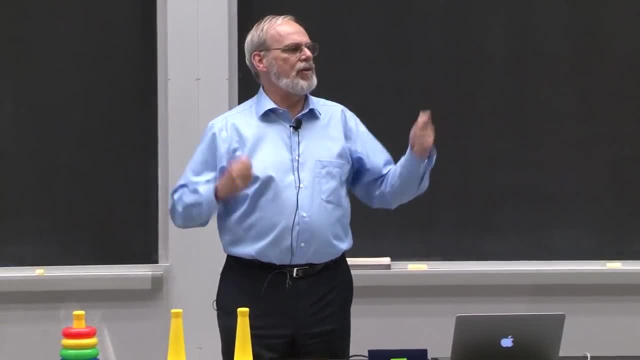 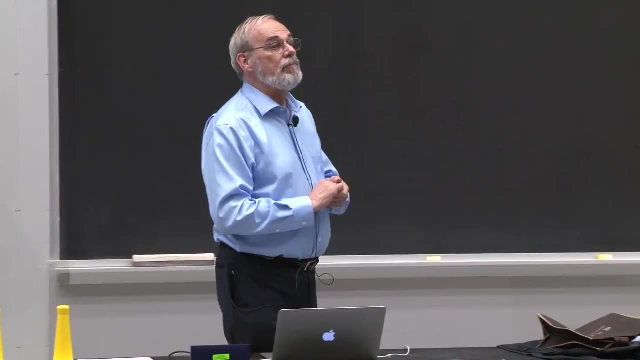 Well duh, that makes sense. If I have the same key in two places in the dictionary, when I go to look it up, how am I going to know which one I want? So it needs to be unique And they also need to be immutable. which also makes sense. If I'm storing something in a key in the dictionary and I can go and change the value of the key, how am I going to remember what I was looking for? So they can only be things like ints, floats, strings, tuples. 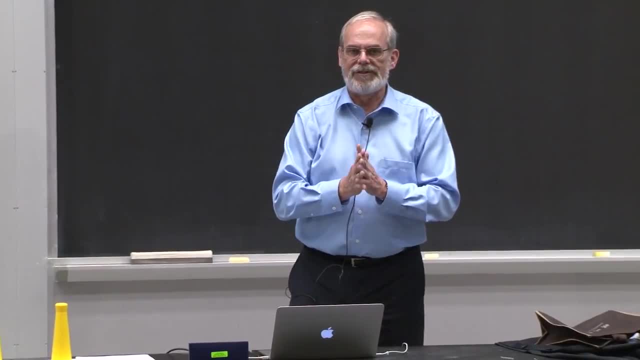 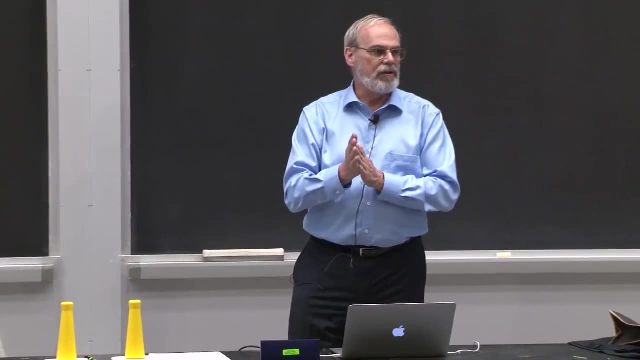 booleans. I don't recommend using floats because you need to make sure it's exactly the same float and that's sometimes a little bit challenging, But nonetheless, you can have any immutable type as your key And notice that there's no order to the keys or the values. 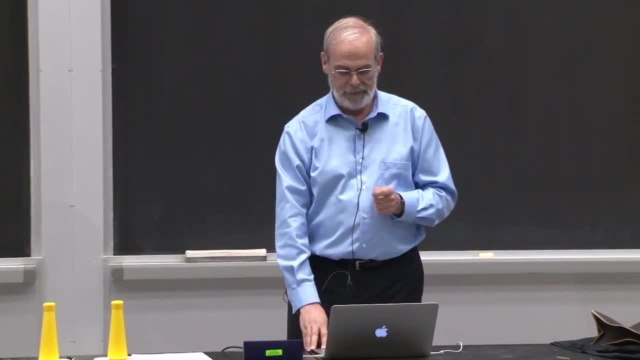 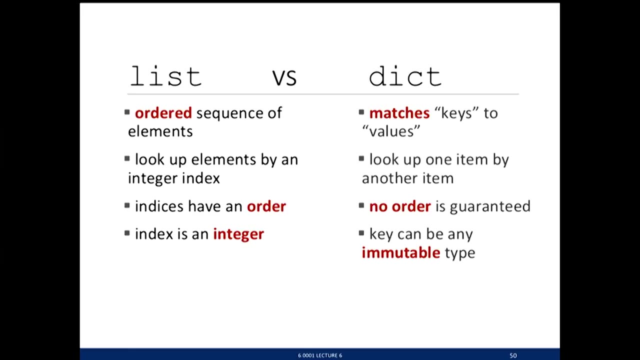 They are simply stored arbitrarily by Python, as it puts them in, And so if I compare these two lists are ordered sequences indexed by integers. I look them up by integer index and the indices have to have an order. as a consequence, Dictionaries are this nice generalization. 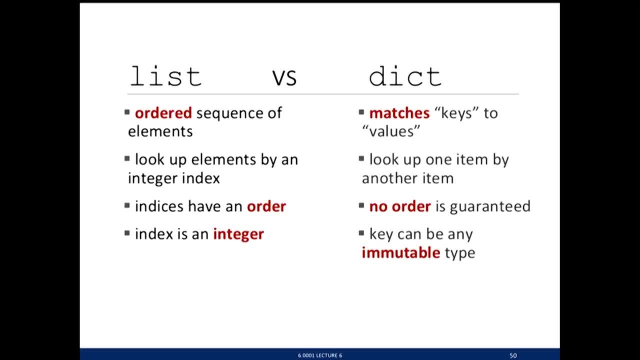 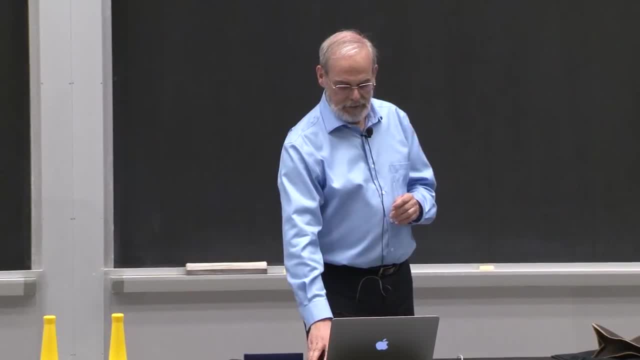 Arbitrarily match keys to values. I simply look up one item by looking up things under the appropriate key. All I require is that the keys have to be immutable. OK, I want to do two last things. We've got seven minutes to go here. 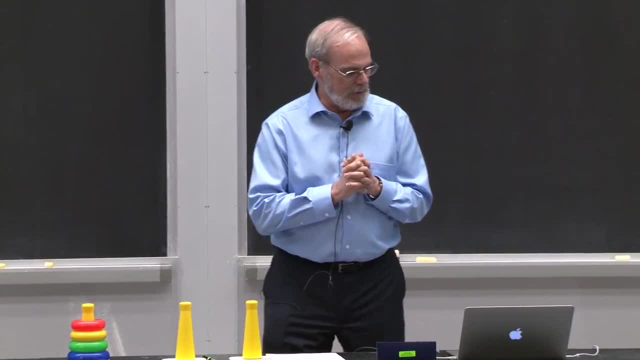 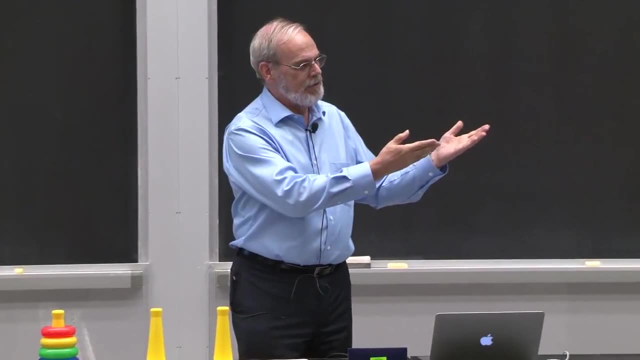 I want to show you an example of using dictionaries And I'm going to do this with a little bit more interesting- I hope- example. I'm going to analyze song lyrics. Now I'm going to show you. you can already tell the difference between my age and Anna's age. 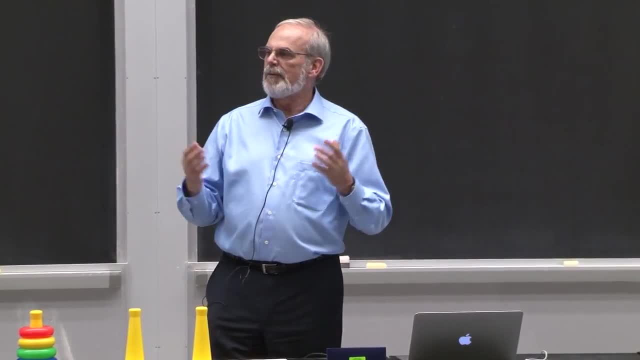 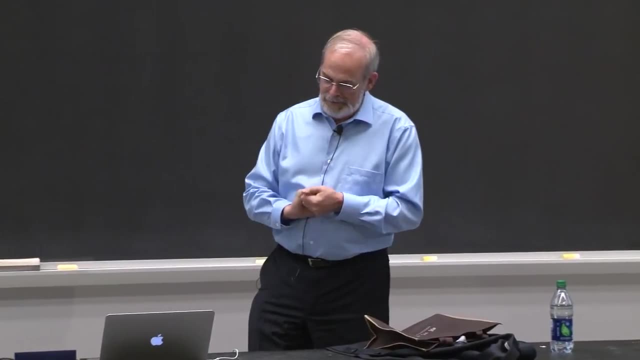 She used Taylor Swift and Justin Bieber. I'm going to use the Beatles. That's more my generation. Most of you have never heard of the Beatles, unless you watched Shining Time Station, where you saw Ringo Starr, right? OK, what I'm going to do is I want. 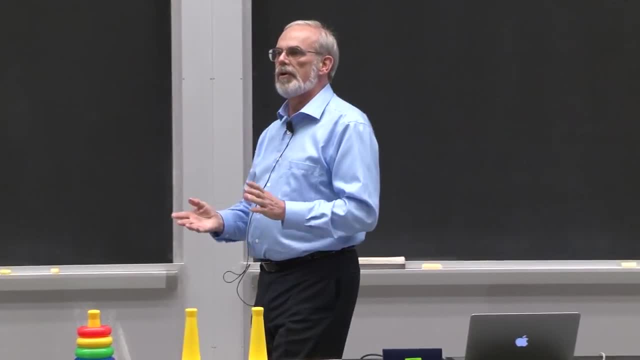 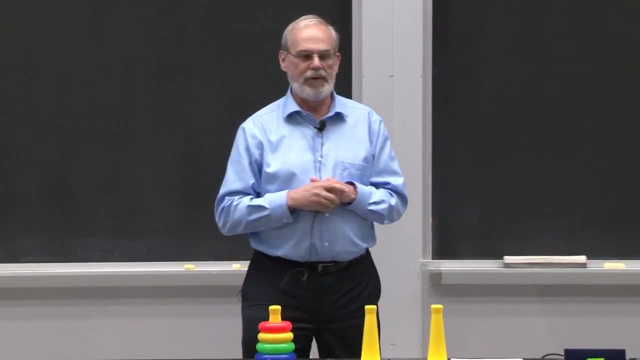 to write a little set of procedures that record the frequencies of words in a song lyric. So I'm going to match strings or words to integers: How many times did that word appear in the song lyric? And then I'm going to ask: can I easily? 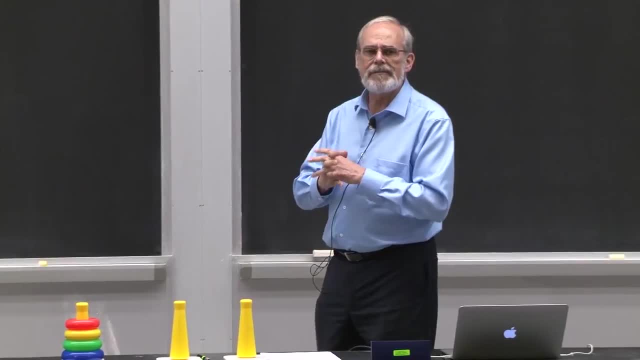 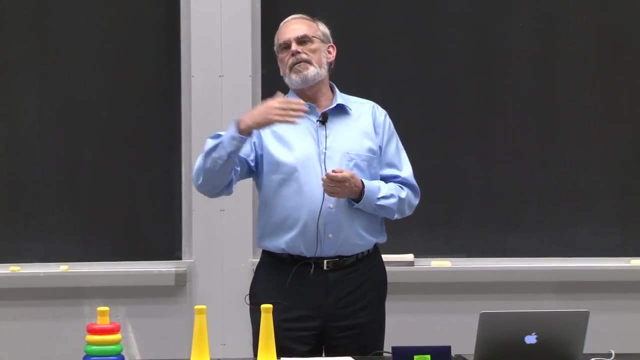 figure out which words occur most often and how many times, And I'm going to gather them together to see what are the most common words in here. And I'm going to do that where I'm going to let a user say I want every word that appears more than some number of times. 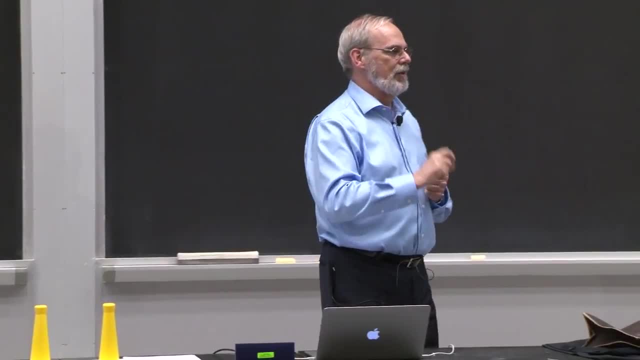 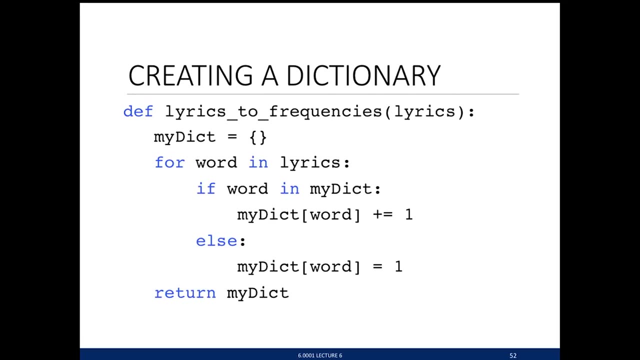 It's a simple example, but I want you to see how mutation of the dictionary gives you a really powerful tool for solving this problem. So let's write the code to do that. It's also in the handout. Here we go: Lyrics to frequencies. 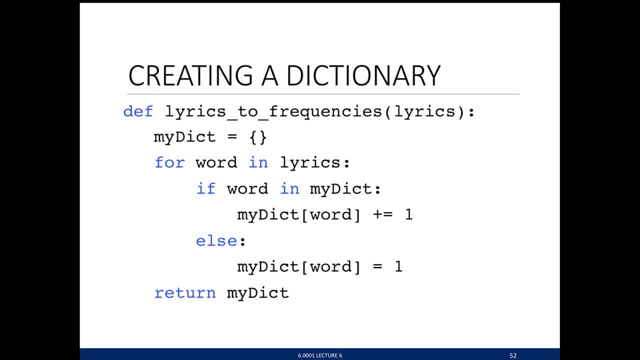 Lyrics is just a list of words strings, So I'm going to set up an empty dictionary. There's that open-close, curly brace And here's what I'm going to do. I'm going to walk through all the words in lyrics. 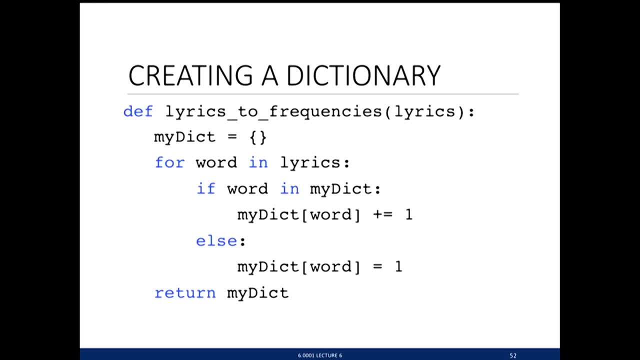 You've seen this before. This is just looping over for every word in lyrics. Notice what I'm going to do. I'm going to simply say so. the first part is: I can easily iterate over the list, But now I'm going to say if the word is in the dictionary. 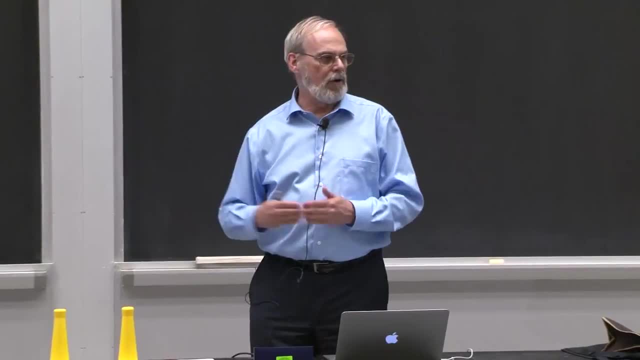 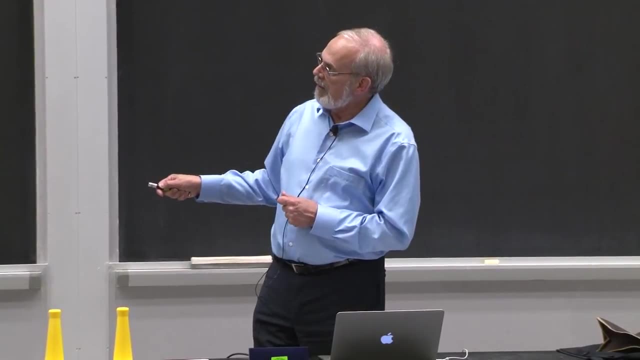 and because the dictionary is iterable, it's simply going to give me back all of the keys. It's simply going to say, in this case, if it's in the dictionary, it's already there. I've got some value associated with it. 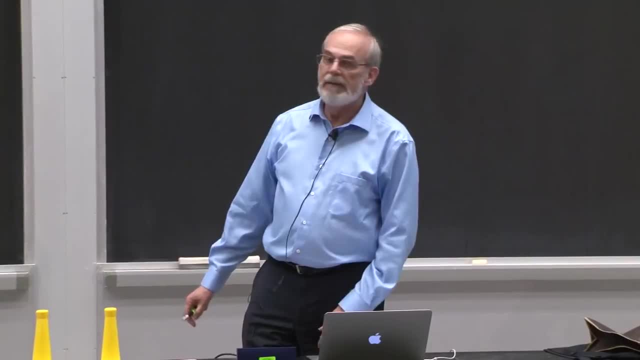 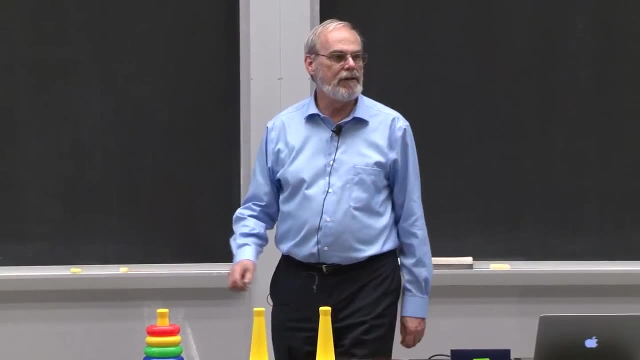 Get the value out, add one to it, put it back in If it's not already in the dictionary. this is the first time I've seen it. just store it into the dictionary And when I'm done, just return the dictionary. 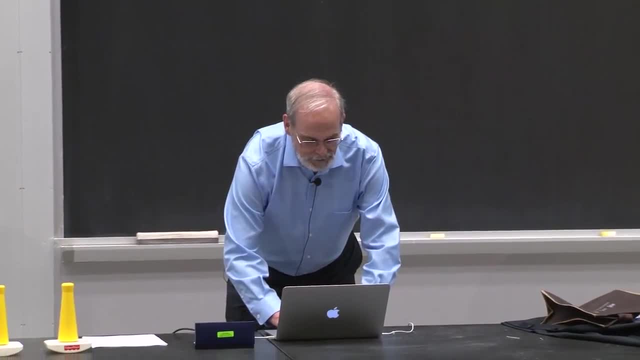 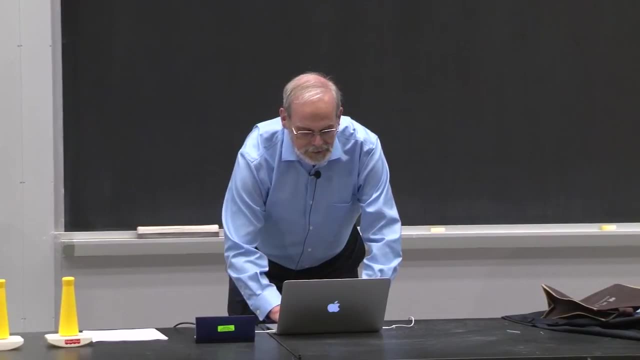 OK, So I'm going to- if I can do this right with my Python, show you an example of this, And I have put in one of the great classic Beatles songs. You might recognize it right there, mostly because it's got a whole lot of repetitions of things. 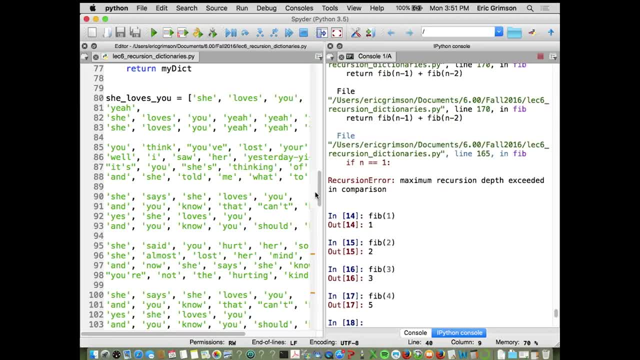 So she loves you, Yeah, yeah, yeah, yeah. I'm sorry Actually they sing it better Than I just did it sarcastically Sorry about that, But I've got she loves you there And here's my code up here: lyrics to frequency: 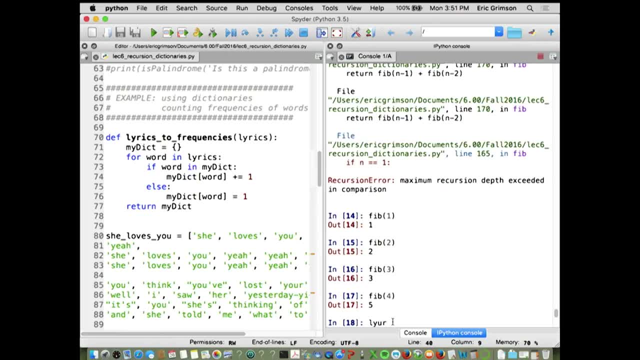 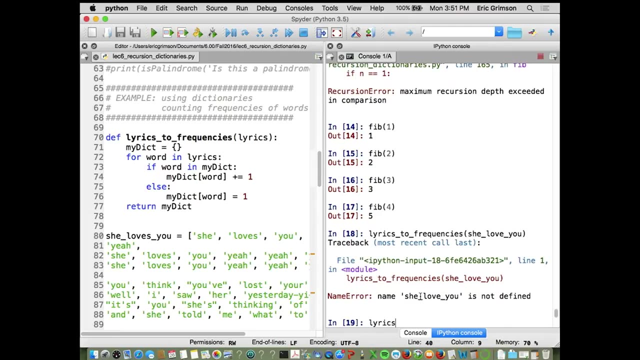 So let's see what happens if we call it And we say lyrics to frequencies of she loves you. And it would help if I can type- All right, we'll try it one more time- Lyrics to frequencies She Loves You. 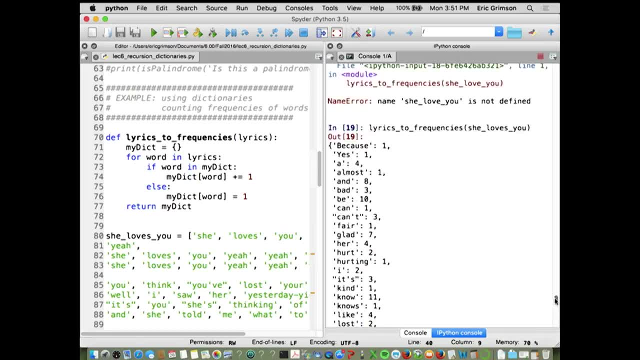 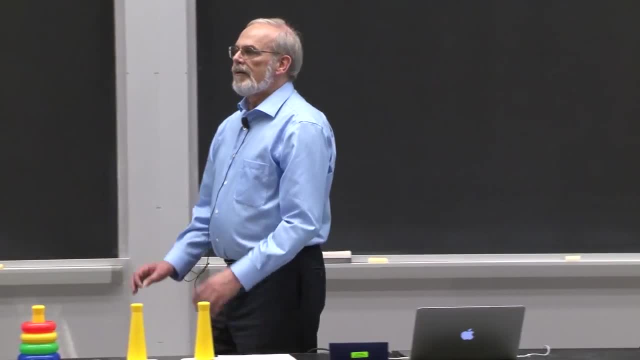 Cool, This gave me back a dictionary. You can see the curly braces And there are all the words that appear in there and the number of times that they appear. What's the order? You don't care, You don't know. What we want to do is to think about how can we analyze it. 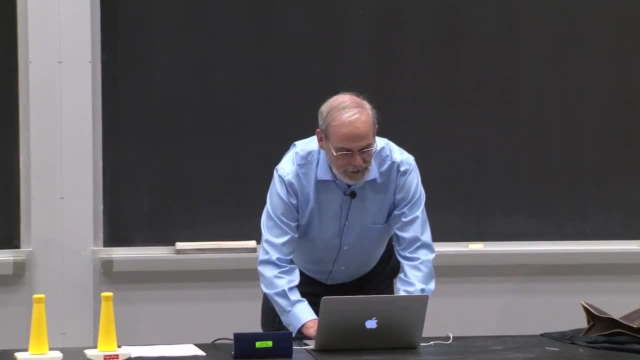 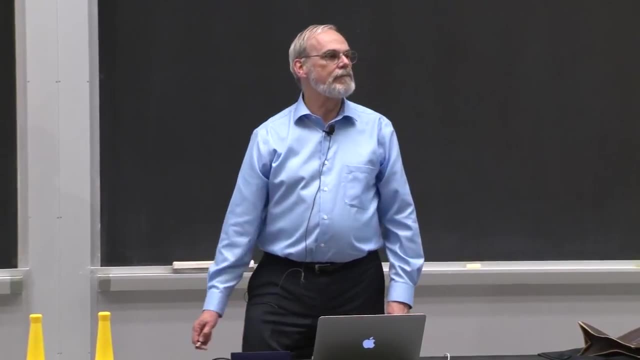 So let's go back and look at the last piece of this, which is OK. I can compute or convert lyrics to frequencies, So here's the next thing I want to do: How do I find the most common words? Well, here's what I'm going to do. 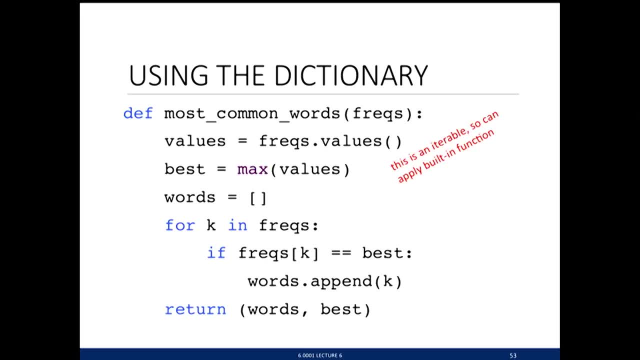 Frequencies is a dictionary, something that I just pulled out, So I can use the values method on it, which returns an iterable. as I said earlier. Again, notice the open- close, because I got to call it. That gives me back an iterable. that is all of the frequencies. 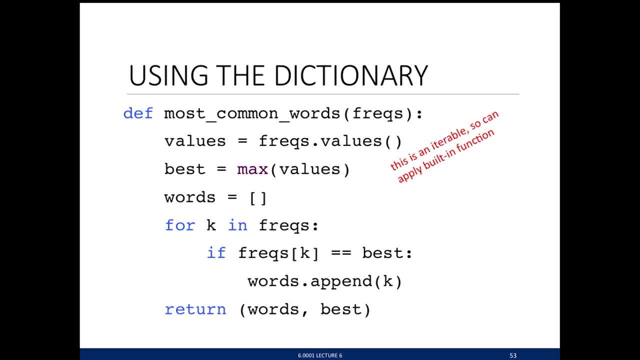 inside of there. Because it's an iterable, I can use max on it And it will take that iterable and give me back the biggest value. I'm going to call that best. I'm going to set up words to be an empty list. 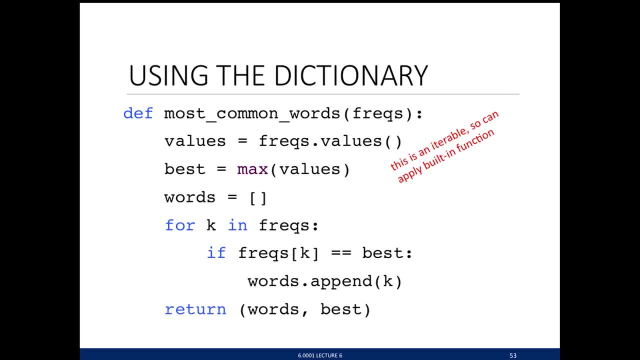 And then I'm just going to walk through all of the entries in the dictionary saying if the value at that entry is equal, to best add that entry into words, Just append it onto the end of the list. And when I'm done, all of that loop. 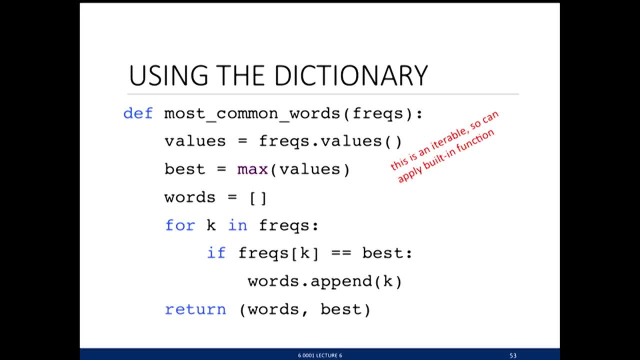 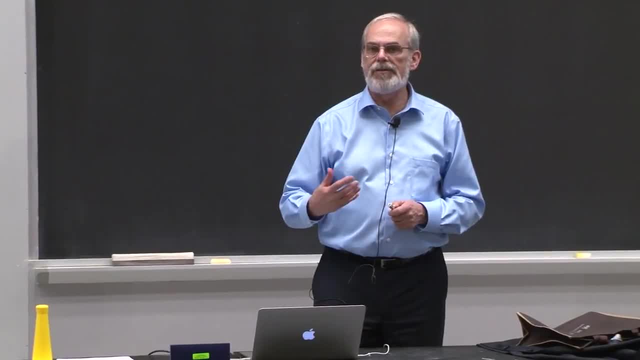 I'm just going to return a tuple of both the collections of words that appeared that many times and how often they appeared. I'm going to show you an example in a second, But notice, I'm simply using the properties of the dictionary. The last thing I want to do, then, is I: 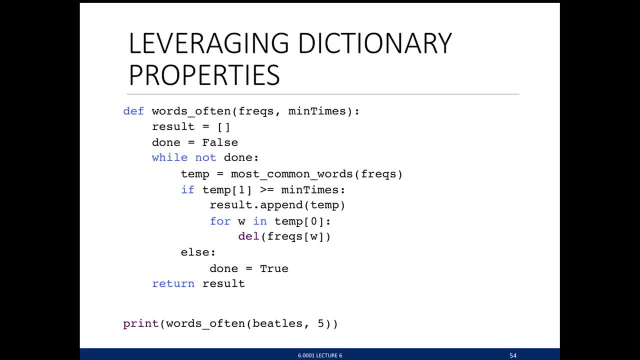 want to see how often the words appear. So I'm going to give it a dictionary and a minimum number of times, And here I'm going to set result up to be an empty list. I'm going to create a flag called false. 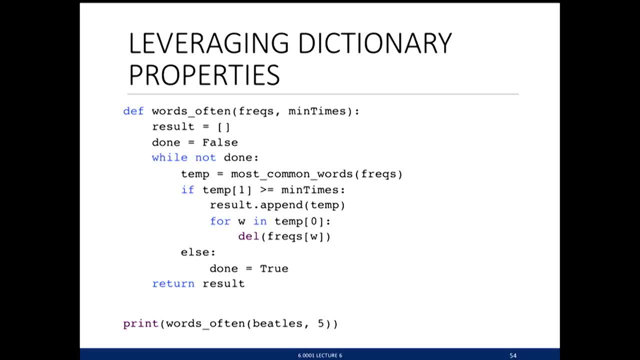 It's going to keep track of when I'm done And as long as I'm not yet done, I'll call that previous procedure. that's going to give me back the most common words and how often they appeared. I check. Remember it was a tuple. 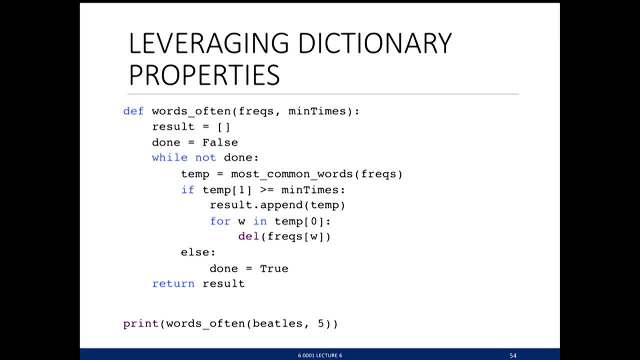 How often did they appear? If it's bigger than the thing I'm looking for, I'll add that. I'll add that into my result, And then the best part is I'm now going to walk through all the words that appeared that many times and just delete them. 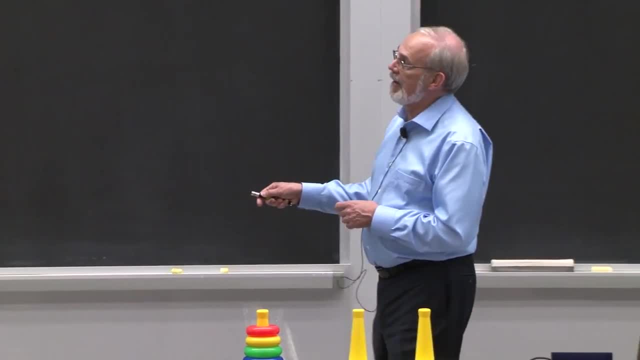 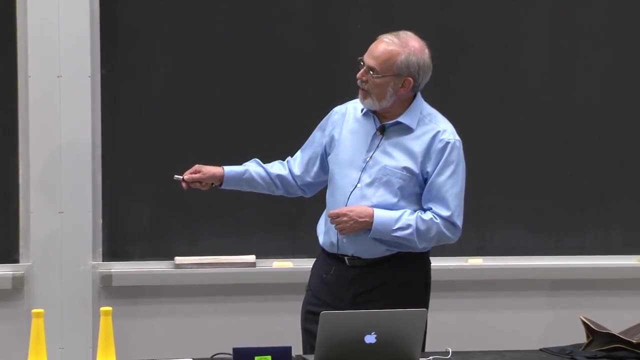 from the dictionary. I can mutate the dictionary And by doing that I can go back around and do this again And it will pull out how many times has this appeared? and keep doing it When I can go all the way through that. 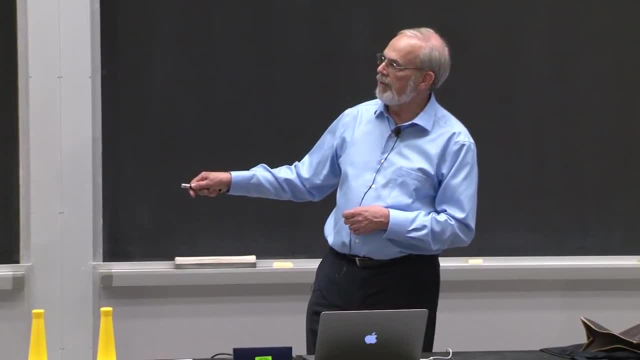 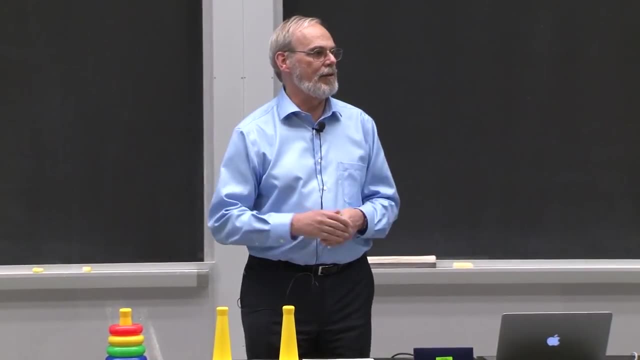 if I can't find any more, I'll set the flag to true, which means it will drop out of here and return the result, And I'm going to let you run this yourself. If you do that, you'll find that it comes up with not surprisingly, I think yes. 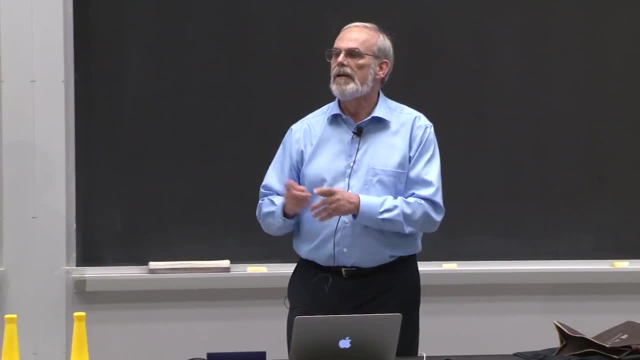 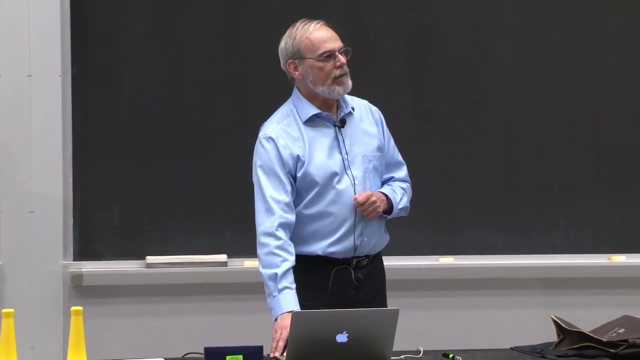 the most common one, and she loves you, followed by loves and a few others. What I want you to see here is how the dictionary captured the pieces we wanted to. Very last one, There's Fibonacci, as we called it before.